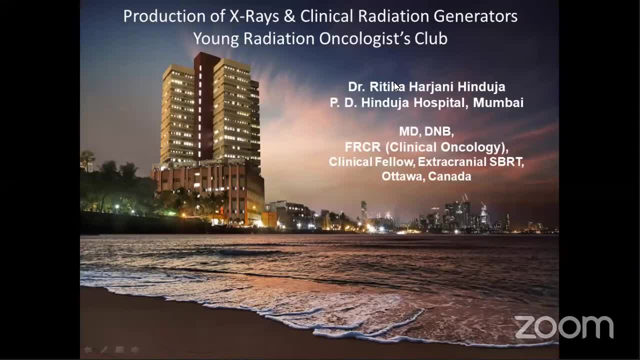 Thank you. Thank you, Can we start? Yes, sir, I think it's eight. Okay, Sayan, we can go. Yes, sir, We can start now, Because this is a big chapter. Okay, fine, So a very warm. 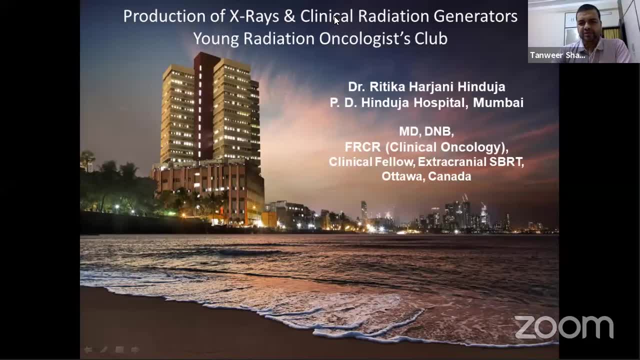 good evening to all of you. On the behalf of Young Radiation Oncology Club, I, Dr Tanvir Shahid, I welcome you all. Basically, Sayan has given me this privilege to introduce Dr Hrithika Harjani. 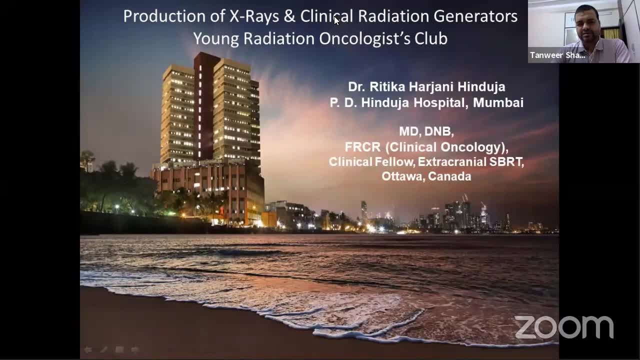 Before that, I'd like to thank Dr Sayan for basically bringing this concept of the physics classes. It was really long thought of and it was in the waiting, but Sayan made it happen, And what added to the entire beauty of this class was that. 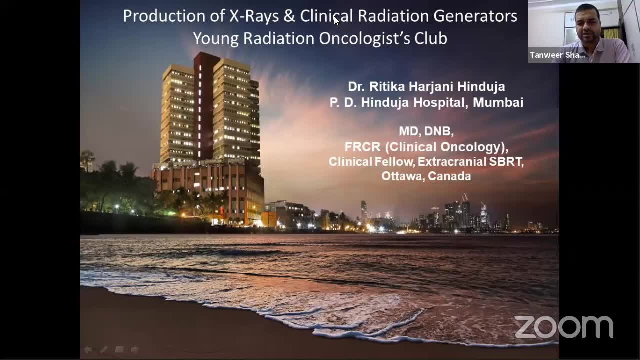 Shantam really stepped in and helped us a lot, along with a lot of young people like Dr Jeevak, Dr Mukti, Dr Sayan Sayan, Paul Sayan Das, Dr Rashi- everybody who is helping. 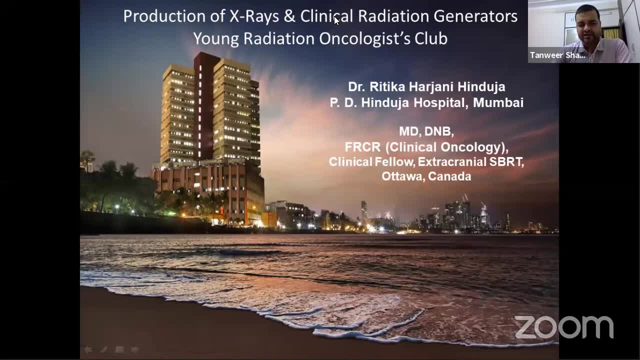 The first class was indeed a great, and I'm sure the second will be even better. To begin with, Dr Hrithika Harjani Hinduja. You know, I still remember how Dr Hrithika became such a famous overnight. 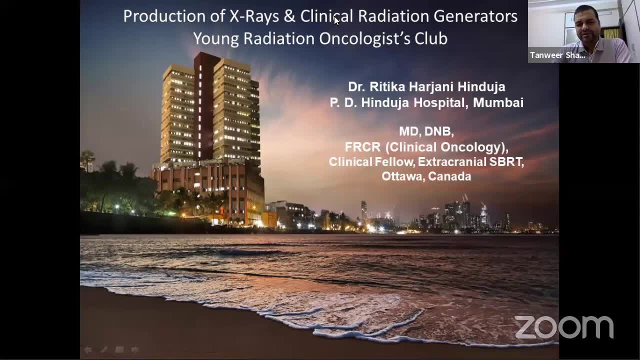 It was a month of June when she came with a concept called as Update Redong- And I still remember it was 13th of June- with six articles in which she had tried to extract the main abstracts from the six journals And she posted in all the groups. 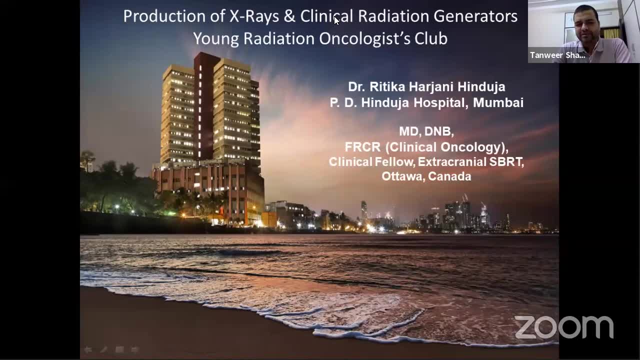 And I think not even overnight. during the day itself. she became so famous that everybody keeps on waiting that. when is the next issue going to come? July came with nine journals and August came with 12 journals. I don't know September, how many more journals will be added? 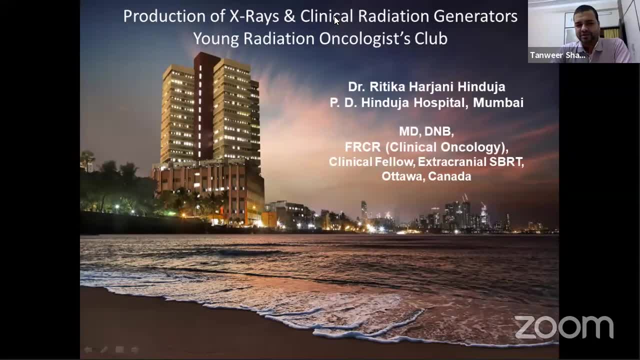 But Hrithika Harjani Hinduja, I must say you are doing a great job by putting that Update, Redong. It's really amazing compilation, I must say. Today she is going to take us to the journey of production of X-rays and clinical radiation. 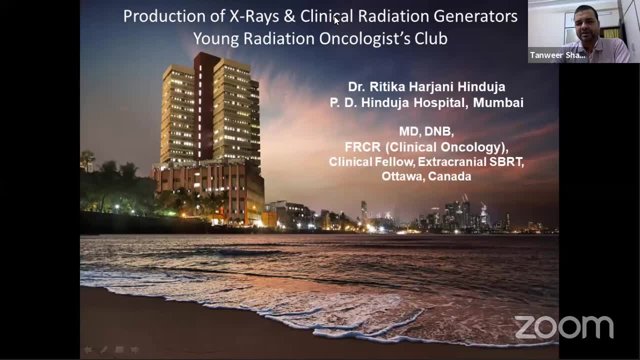 generators, And I am sure it will be a great class. So welcome you all. Welcome Hrithika, Now it's your, it's up to you, Just go ahead. Thank you so much. Thank you, sir, That was very kind. 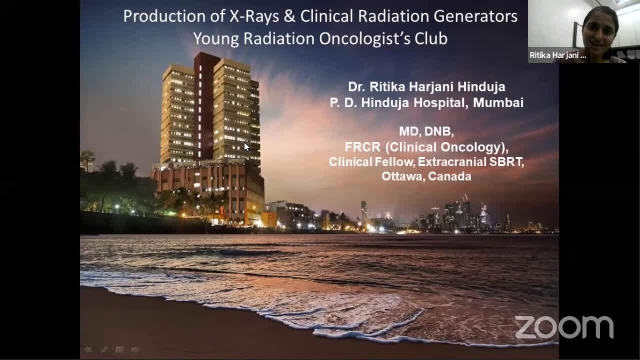 of you to praise it so much and mention it here, And thank you to the Young Radiation Oncology Club for giving me this opportunity. Of course, the first class was wonderful. Dr Jeebwag did a wonderful job and I hope I live up to the expectations. 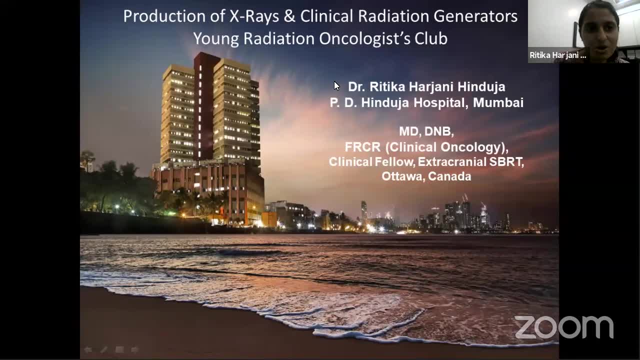 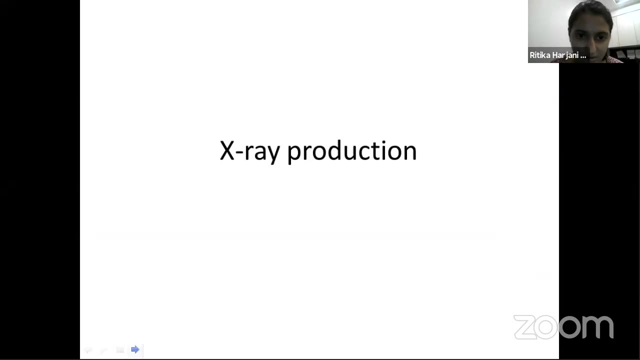 So, beginning with the class, I would be talking about production of X-rays and clinical radiation generators. My slides are moving fine, right On the screen, Absolutely, it's moving. So, beginning with the first part of it, as we have made it, 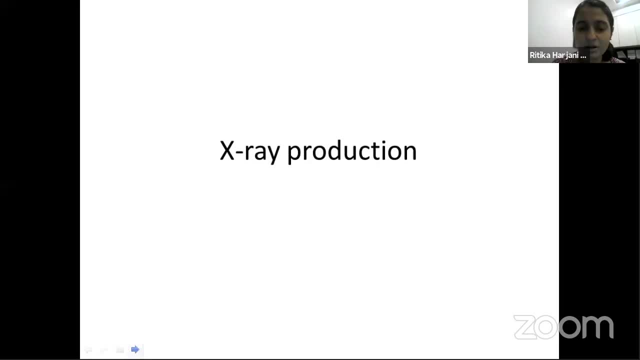 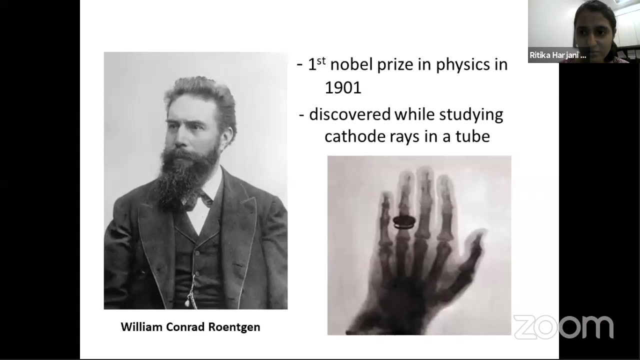 clear. we are covering FM Khan chapter wise. So the third chapter on the book, X-ray production, And then I will deal with the clinical radiation generators. So we all are very well aware that X-rays were discovered by Sir William Conrad Ronjan And 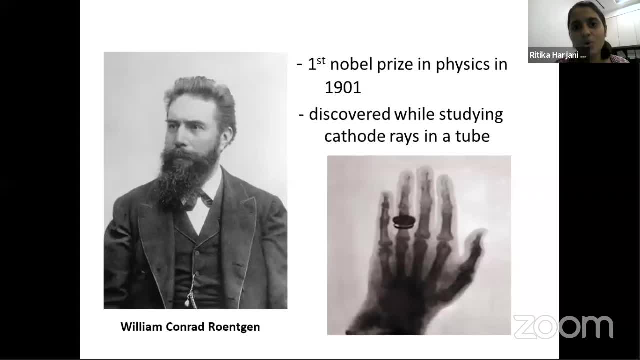 he discovered it actually accidentally, while he was studying cathode rays while passing through a tube, And then he thought that it could even pass through opaque substances and produce fluorescence. And then you always experiment with your wife, So he took an X-ray of his wife's hand and he actually 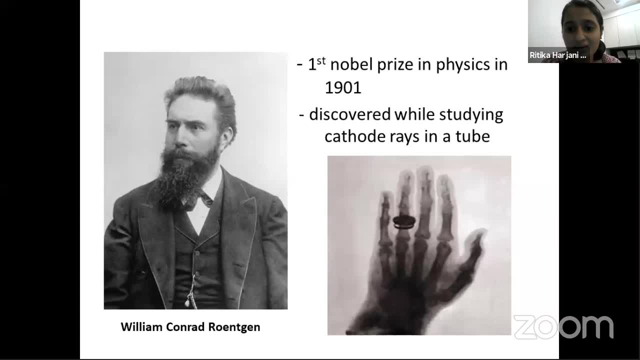 let the beam pass through his wife's hand and produced an X-ray. He called it X-ray because generally anything unknown, we call it X, So that's how X-rays were coined and he received a Nobel Prize. That was the first Nobel Prize in physics. 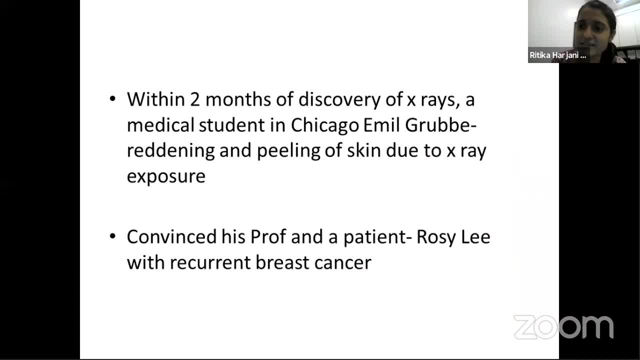 Within two months of discoveries of X-rays, there were people who were excited and wanted to try it in radiation, And there was this particular medical student, Emil Grue, who noticed that these X-rays produced reddening of the skin and even peeling of the skin. 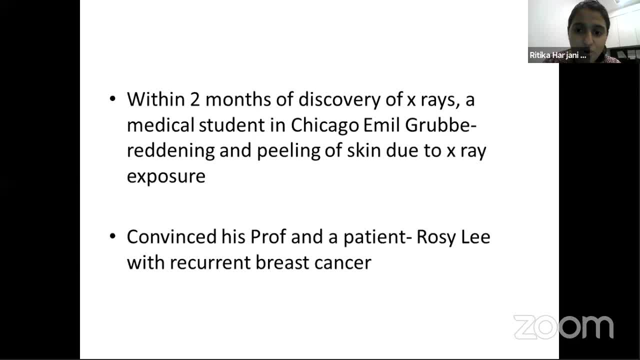 So he convinced his professor and, of course, a patient also who volunteered, And Rosie Lee was the first patient treated with X-rays for a recurrent breast cancer. So coming to the X-ray basics now. So this is a basic X-ray tube, A modern. 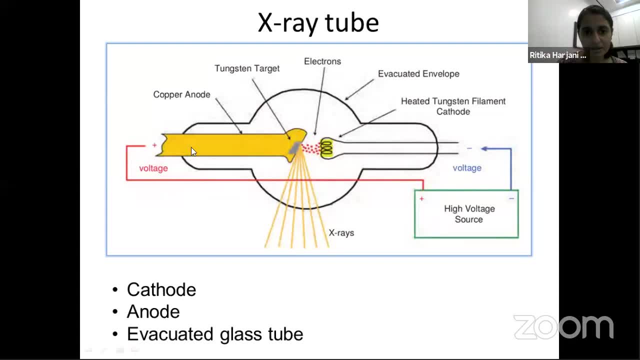 X-ray tube is called as a Coolidge tube, So it has three basic parts or more. This is the cathode end at the cursor, which has a filament. The opposite end is an anode, which is the positively charged element, And it is 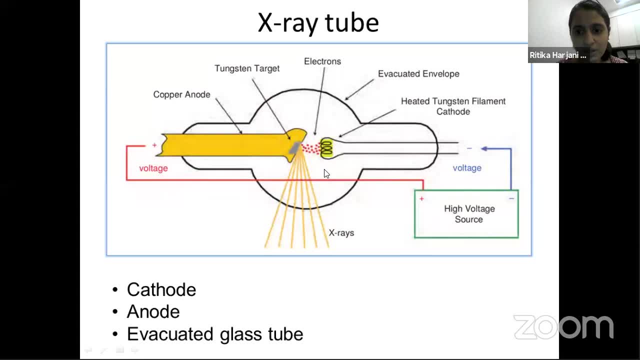 all in a glass, vacuum sealed tube. I will come to details of it. So, basically, what happens is this: cathode filament is provided with some voltage and it gets heated up. Once it is heated up, there is an electron cloud that forms around it and these electrons are ejected. 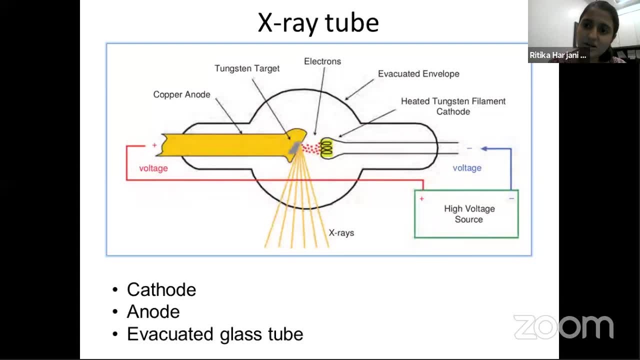 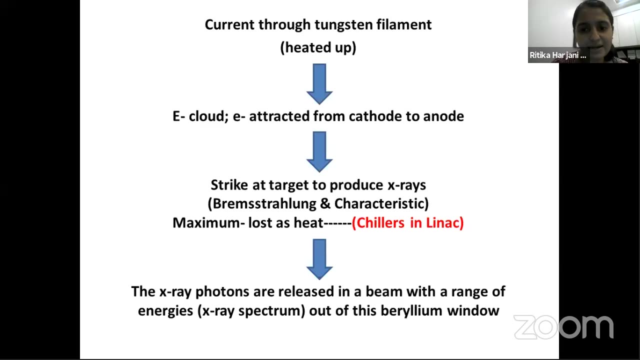 These electrons are ejected towards these negatively charged electrons are ejected towards the positively charged anode And they interact with the target in the anode and produce X-rays. So basically, they produce two types of X-rays: Bremstelung and characteristic. 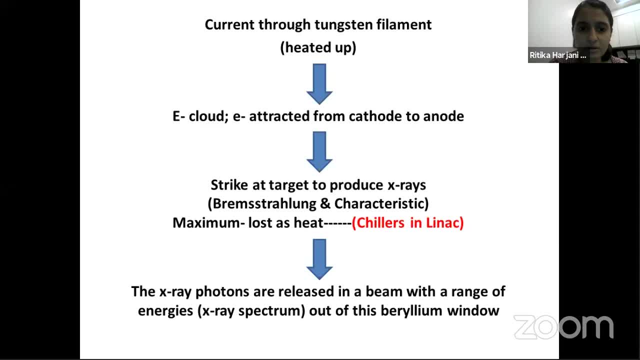 But we will deal with that a little later. And not that all the electrons that hit the target actually give rise to X-ray production. A lot of it, or rather 99% of it, is lost as heat. That is why, as an application, we would: 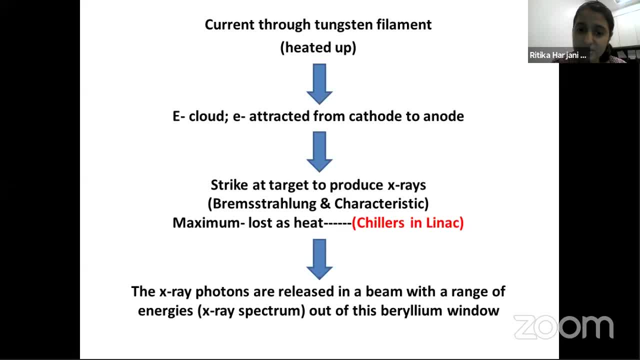 see very large chillers in our. that is because there is 90% or 99% is getting converted into heat and only efficiency of 1% is there. These X-ray photons are then released in a beam with a range of energies. So, coming to the cathode, 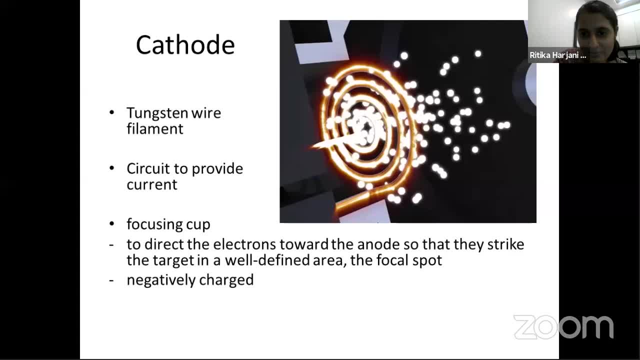 So this is the filament on fire and emitting those electrons. So, basically, the components are a cathode filament which is of tungsten and there is a circuit which is provided to it which provides the voltage for it to get heated up and release the electrons. There is a 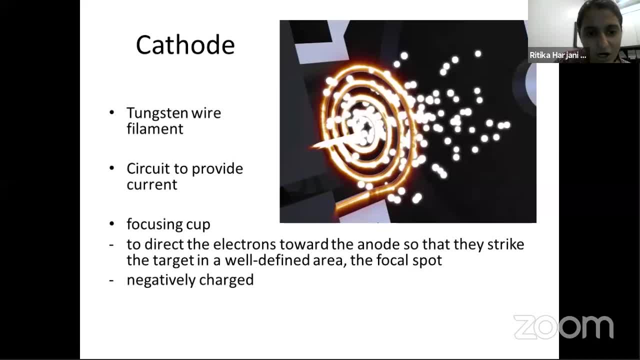 focusing cup- I will show the focusing cup in the next slide- To direct these electrons towards the anode so that they actually strike the target in a well defined spot Coming to the anode. So in this picture, if you also notice besides this, 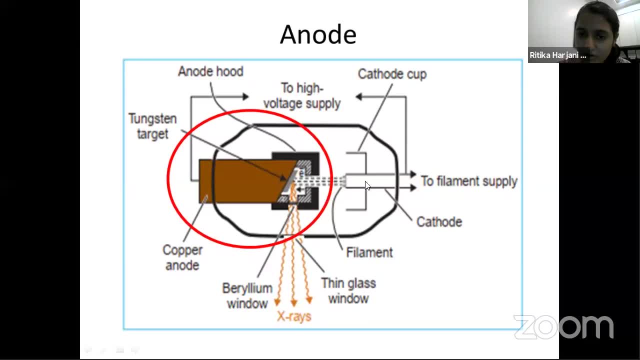 red envelope of anode. there is this cathode filament with this cup, focusing cup, Coming to the other part, the anode. So this is an anode complex which has certain parts. This brown part is the copper anode with a target where the electrons actually 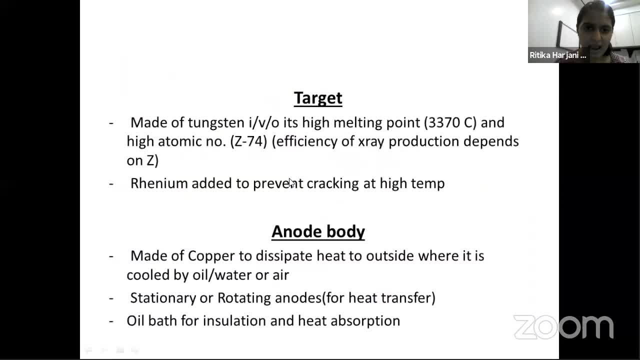 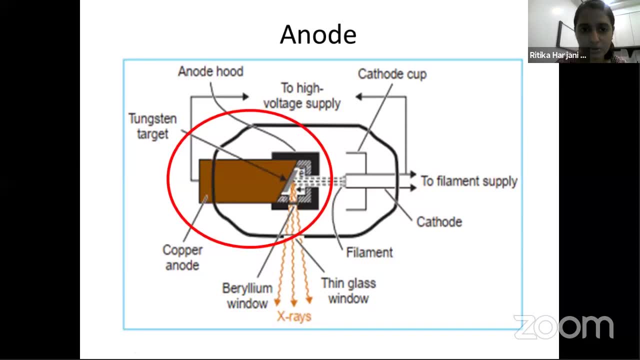 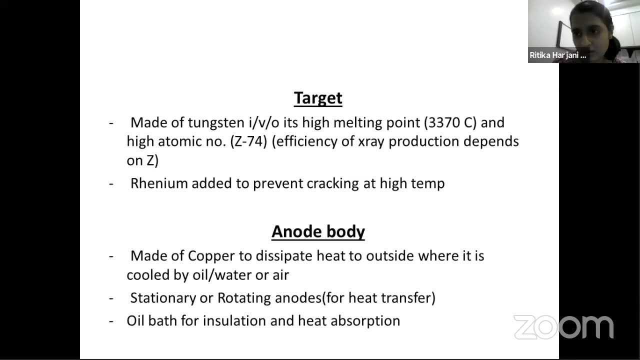 come and strike the copper anode and it also has a hood, or covering, which has its own function. We will come to it. It is called the anode hood, So each part by it. So the target which is the most important for us, is made of tungsten. 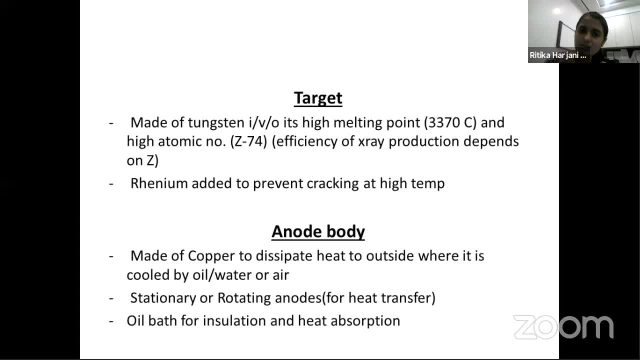 Often we are asked: why tungsten? So there are two reasons to it. One is tungsten is a high atomic number, material. Dr Jeebak very well covered what is atomic number, mass number. So the number of protons or electrons is high. 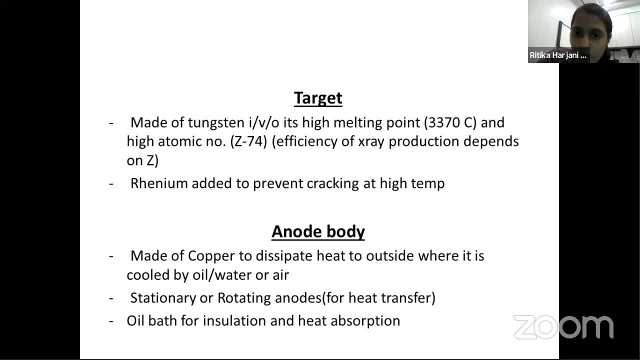 for tungsten 74. And it has a high melting point, So with the heat generated it would not melt. So that is the reason target is made of tungsten And generally it is not pure tungsten and alloy of other substances. 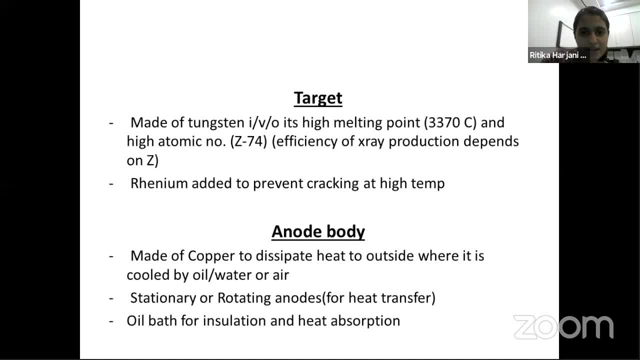 So commonly rhenium is added to prevent cracking at those high temperatures. Also, the efficiency of the X-ray. why we need a high Z material is important. That is because the efficiency of X-ray production, or how much bremsstrahlung X-rays are produced, would depend. 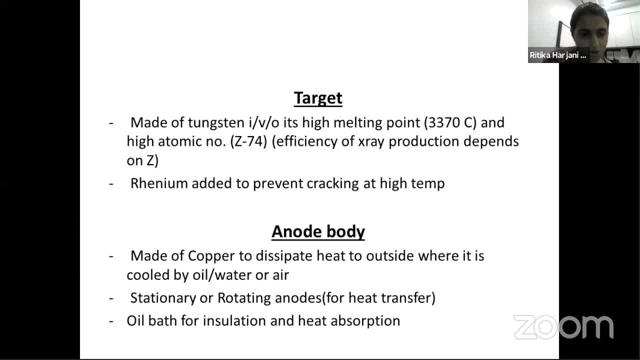 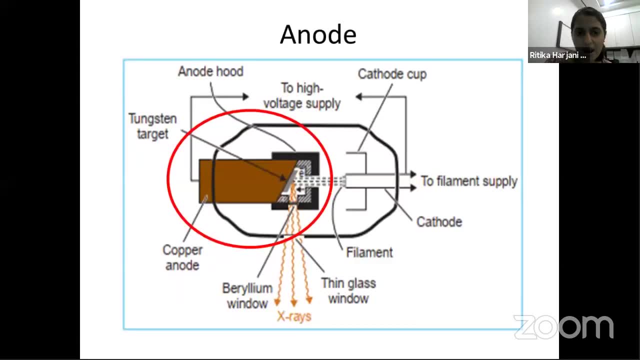 on the atomic number of the material. All that also I will talk in a little detail in a while- And the anode body. So the anode body is this brown part that is seen and on which the target is attached. So this anode body. 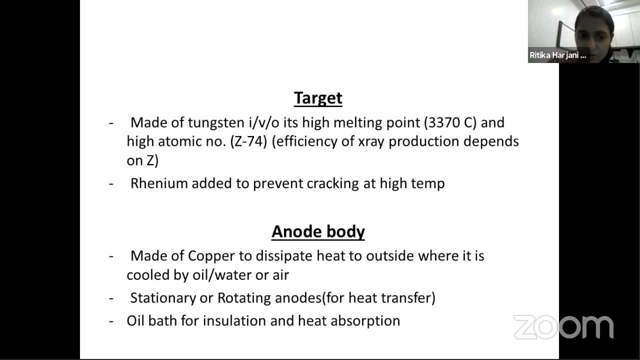 is generally made of copper to dissipate the heat to outside, And outside there is generally a water or a oil bath which takes away the heat. So there is incoming cool water and outgoing hot water, Sometimes more so in radiology machines and not therapy machines. the 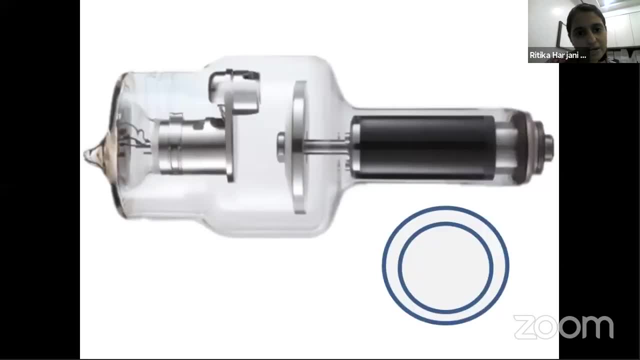 anode is rotating. So this is a photo of a rotating anode wherein, on the right hand side, or if you can notice the cursor, is the anode which there is a motor which, through which it rotates, it can rotate, and on the left hand side, 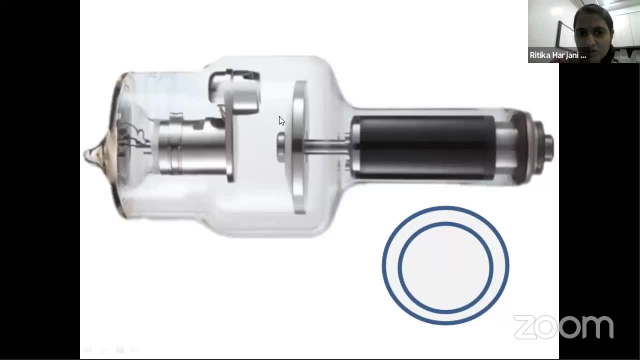 is a cathode, So this: if this anode is rotating, you would see, as in this cross section, it would strike at different areas in this rim, So not one area is receiving all the heat, So the heat dissipation is better. This is not. 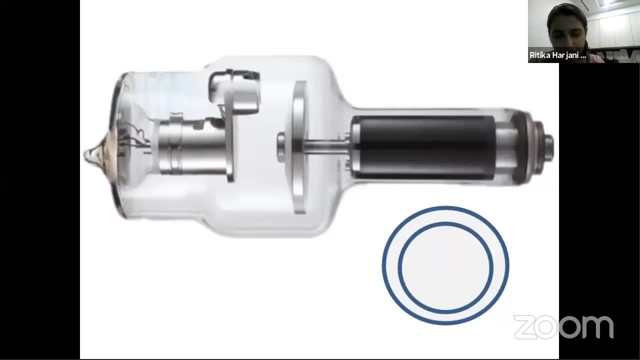 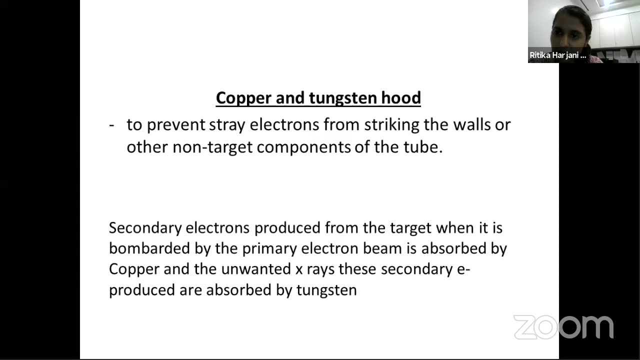 much of use in therapy machines but useful in radiological machines And coming to the copper and tungsten hood. So these electrons, when they strike the target, apart from producing the necessary x-ray beam, it also can produce some stray electrons which can then produce some x-ray emission. So all 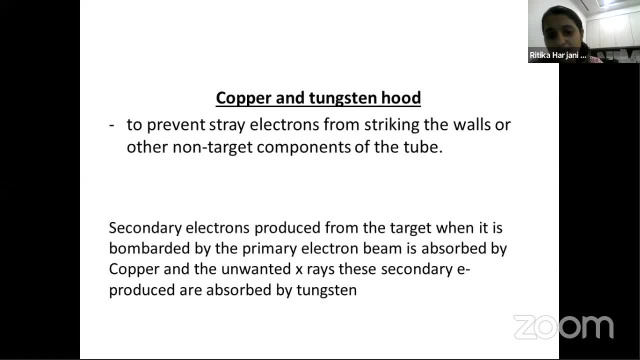 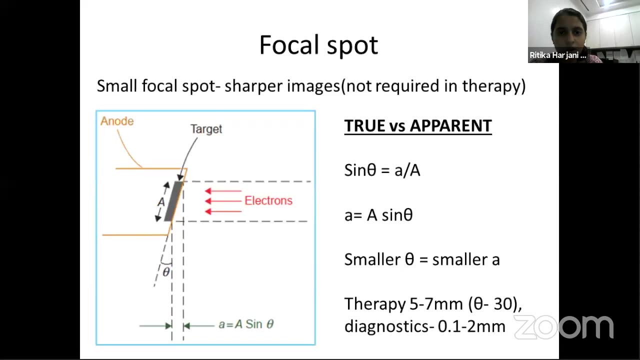 these unwanted, unpure x-ray beam and electron beam needs to be absorbed. So this copper takes away the electron beam and the tungsten takes away the unpure or the unnecessary x-rays that are produced. So when these come and strike on the target, 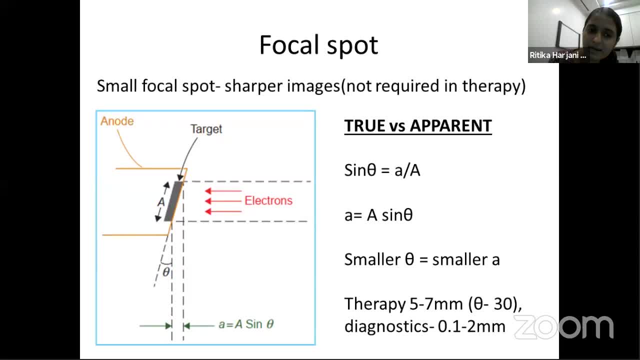 they have to strike on a very specific area on the target, and that is called as a focal spot. Now again, we are dealing with x-ray production, so we will cover it, but it is not much of use in a therapy machine. This is more of a radiology diagnostic. 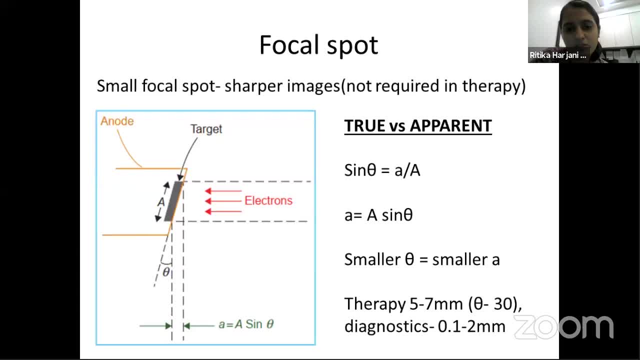 radiology point that if the point where the x-rays come and strike it is a very pinpoint, or smaller that spot is, the sharper the image will be or, in more correct terms, the resolution will be better. So in an x-ray tube we want 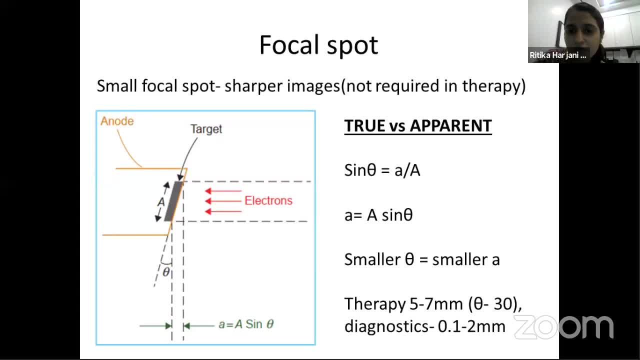 it to strike on a very particular focused point which is called as a focal spot. But then we also require a large amount of various area for the target or the focal spot, so that it has a large area for the electrons to come and strike and interact and produce x-rays, So to. 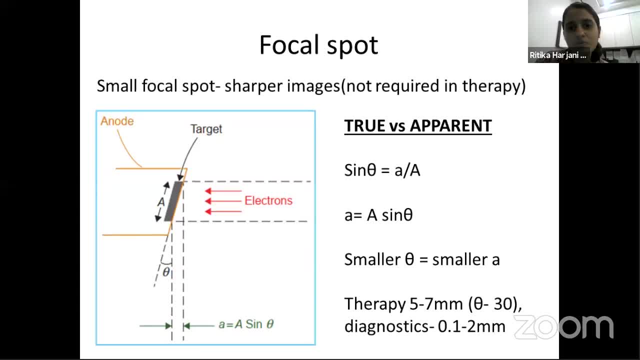 balance the two. there is something called as a true focal spot versus an apparent focal spot. So true focal spot is the big letter A and its projection onto the patient's surface or the machine. exterior is the small letter A which is given by these green arrows. So we 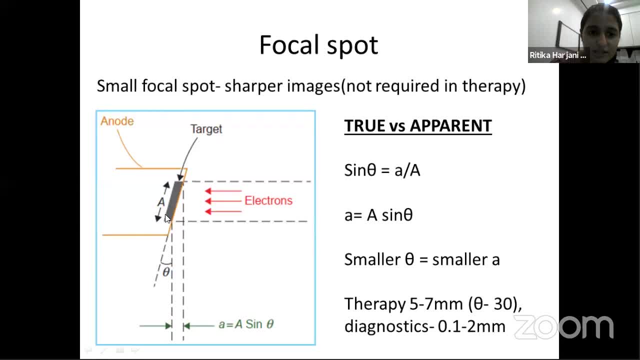 want a small A to be small effectively, So applying some mathematics here. so if this angle with which the target is angulated, if we consider it theta, and to just remember basic trigonometry, sine theta is opposite upon hypotenuse. So then sine. 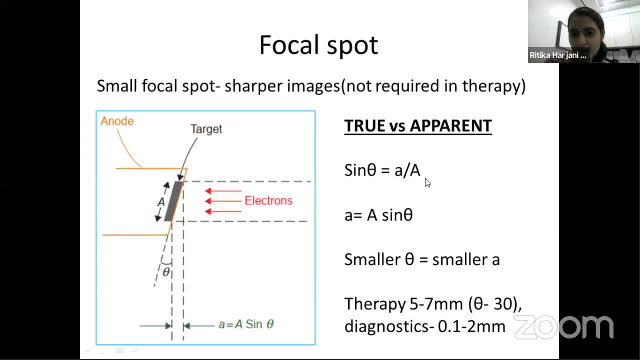 theta would be small A upon big A, and hence we get the small A or the apparent focal spot to be the actual focal spot, but it length into sine theta. So smaller the theta would be smaller the apparent focal spot would be. And in therapy, 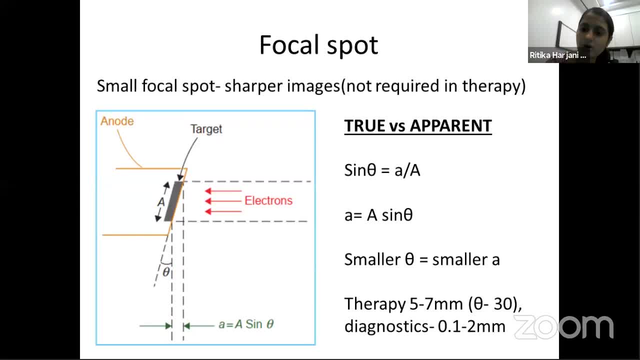 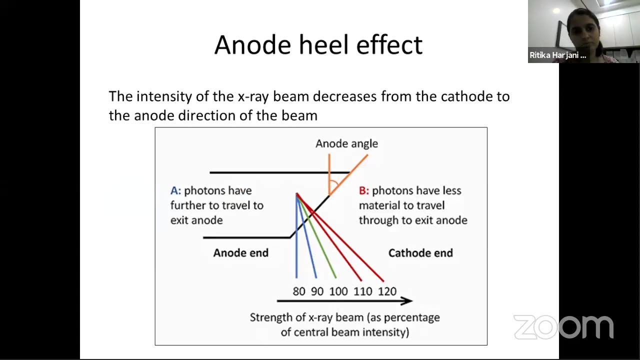 we accept a focal spot of 5 to 7 mm, but in diagnostics they want it to as low as 0.1 mm to produce a sharp image. Again, not very useful in therapy, but useful as a radiation oncologist to know Another thing about the 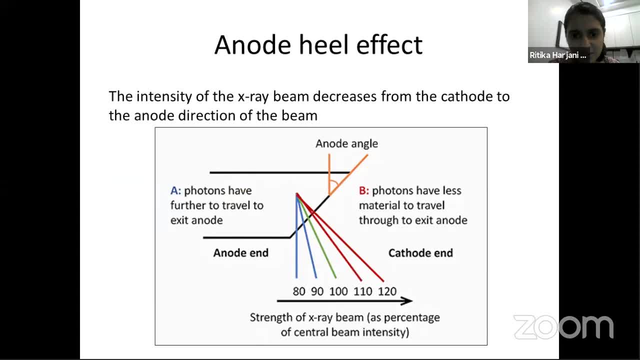 anode that we need to know is this actually sometimes comes as a short question? at least when I passed my PG, it was important to know. So the target is basically angulated, as we just saw, and when it is angulated when the electrons are coming from. 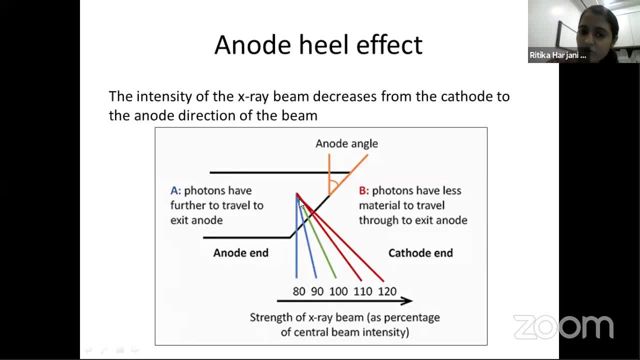 the cathode end and when they are emitted they have to pass through different lengths of the anode material before coming out. So these red rays have to pass a smaller material or a smaller length of material than these blue rays. So the intensity of the x-rays 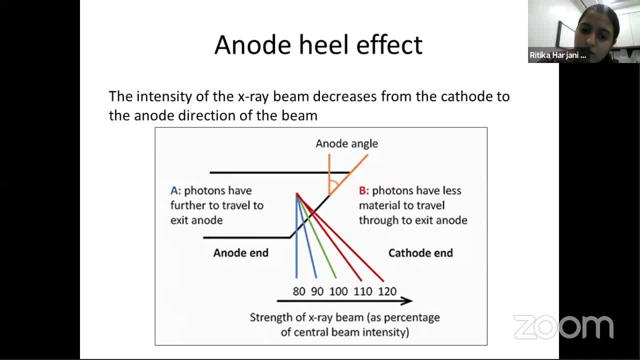 from the cathode end to the anode end actually decreases slightly, and this is called as the anode heel effect. Now, anode heel effect, there may be filters to correct for it, but many times in diagnostic radiology what they do is they make use of it. 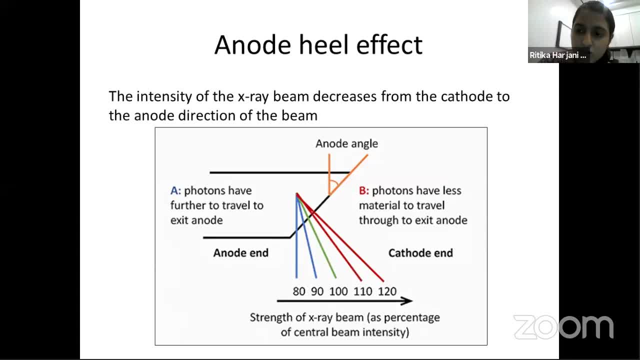 If you want to do an x-ray of a patient. so the high density or the more wherever there is more dense material, they keep it on the cathode end, like if you are taking a foot, the ankle side would be near the cathode versus the anode side. 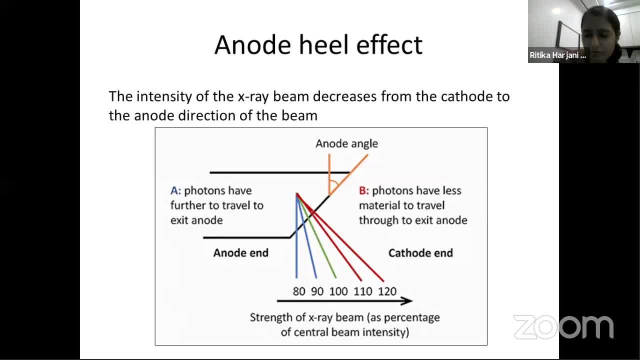 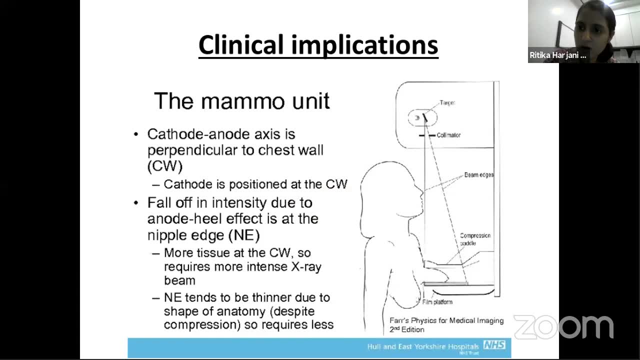 will be near the anode, the toe side Or in oncology. an implication would be when you are doing a mammograph, when you are doing the cranial caudal, if you make sure that, if you notice in this image, if the anode side or where the intensity 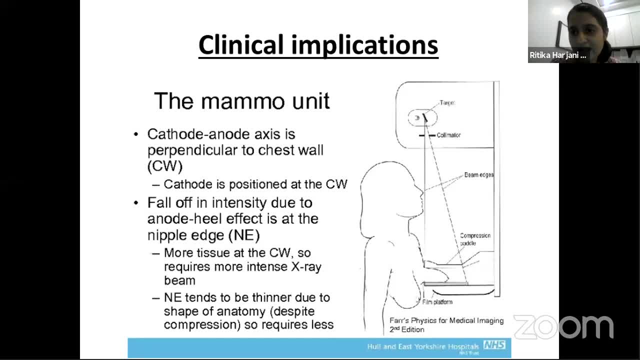 is less is kept near the nipple end and the cathode side, where the intensity is more, is kept near the chest wall and as a normal contour of a breast would be. that will take use of the anode heel effect and a sharp image will still be created. 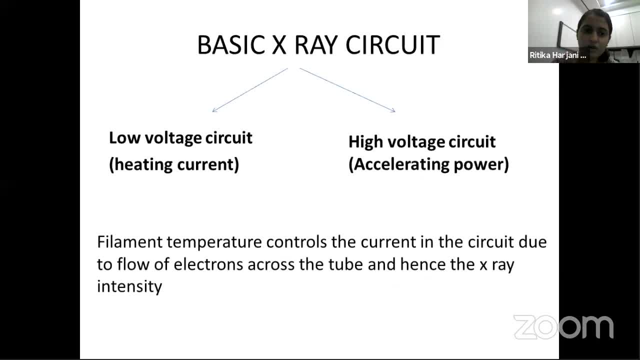 So basic x-ray circuit that we provide would have. we will provide a circuit to the low voltage circuit to the filament for it to get heated up and once it is heated up through thermionic emission it emits electrons to the anode and a high voltage circuit is created, which is the 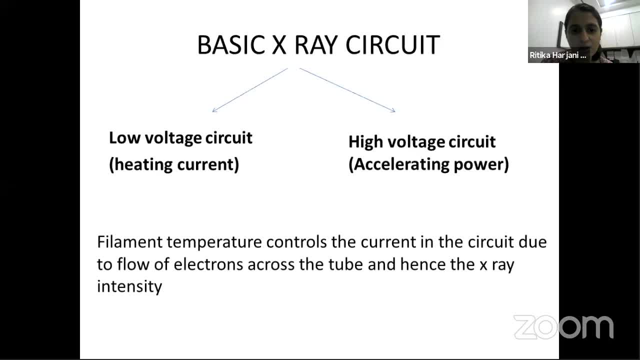 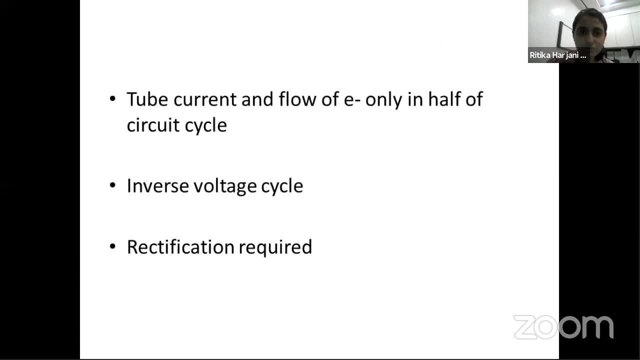 higher voltage because of movement of electrons to anode. The filament temperature that we provide controls the current and then it causes the flow, as I mentioned. So this is not much of requirement for us as radiation oncologists, but just to touch up on the basics. this 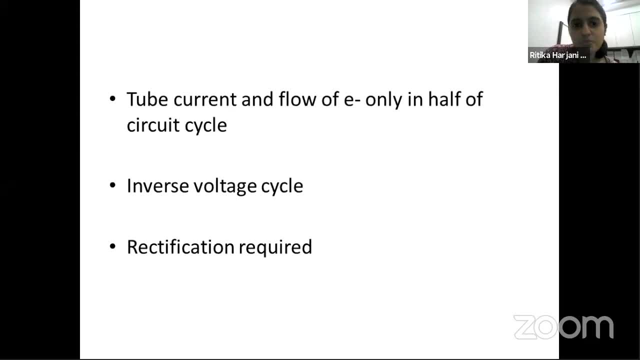 tube current that we, because it has pulse cycles, this tube current and flow of electrons occurs only in half of the circuit cycle because because of the pulses- voltage, pulses- the cathode is negative with respect to anode only in the half cycle. so the reverse, so overall. 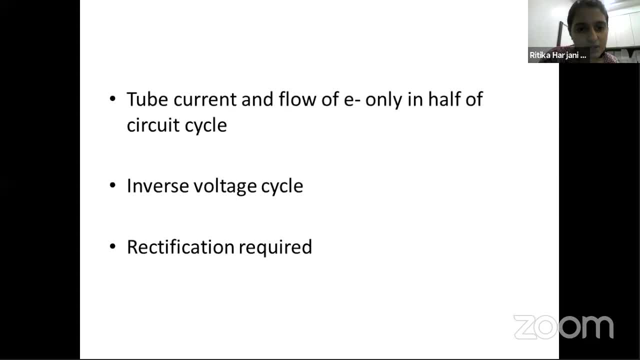 by that we imply that, okay, the efficiency must be there only in half the cycle. but sometimes what happens is because of the heat generated in the anode, the anode becomes heated up and emits electrons. because of thermionic emission and when there is no negative voltage to cathode, 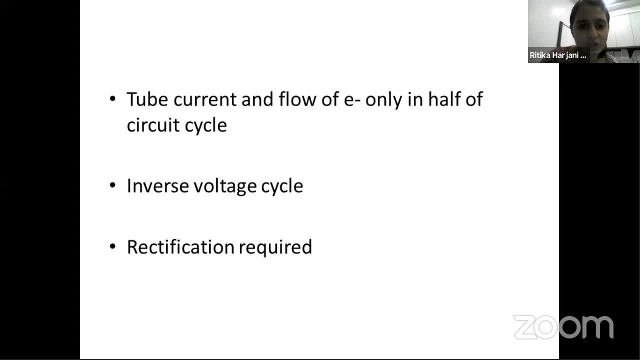 there is a reverse current that may flow and damage our x-ray tube. so that is where we apply some rectifications, which may be half wave and full wave. I don't think we need to dwell into the details of these rectifications and for the constraints, 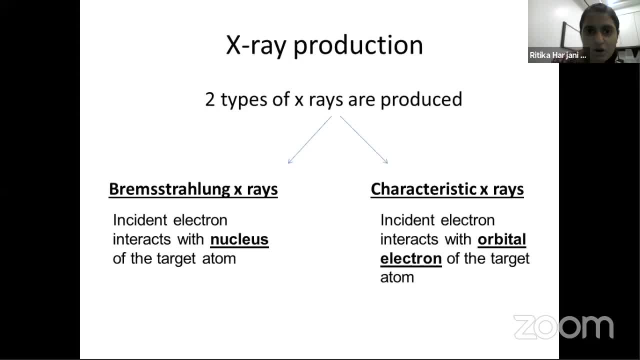 of time, I have not covered that. so this is how the x-ray tube basically is. and then, as I mentioned, when the x-ray tube, when the electrons in the x-ray tube, come and strike the target, there are x-rays produced. there are two types of x-rays produced. 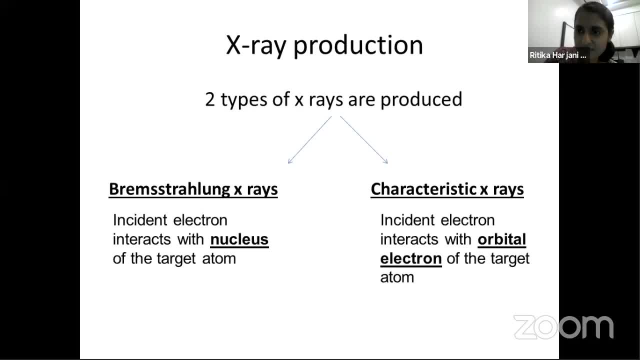 to remember: bremsstrahlung and characteristic, two basic things in that is: bremsstrahlung is when the electron interacts with the nucleus, and characteristic is when the electron interacts with another orbital electron. so bremsstrahlung with nucleus and characteristic with electrons. 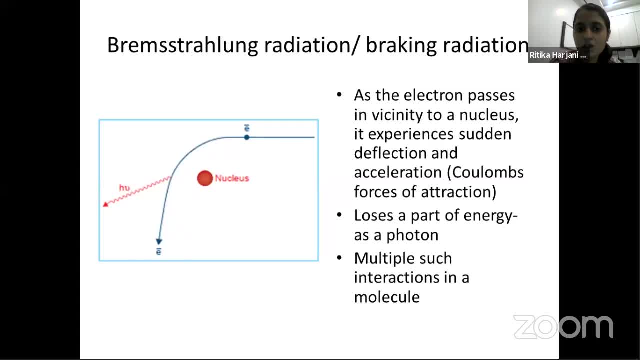 coming to the first, the bremsstrahlung or the breaking radiation. so as we know that electron is negatively charged and nucleus is positively charged because of the proton, so as the electron comes in vicinity to a nucleus, it experiences coulomb's force of attraction. 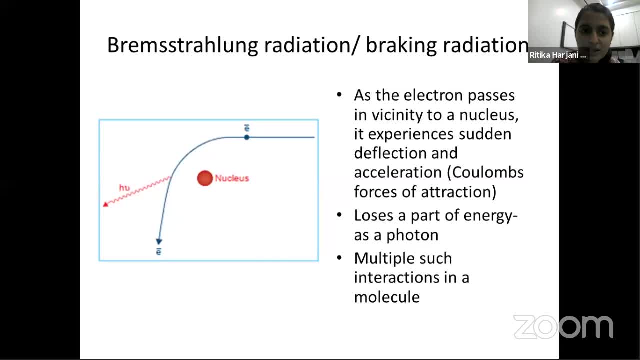 towards the nucleus, so it changes its direction and loses some amount of its energy. this amount of energy is lost as a photon or an x-ray is released with the energy h nu that is the Planck's constant into frequency. so this is how bremsstrahlung 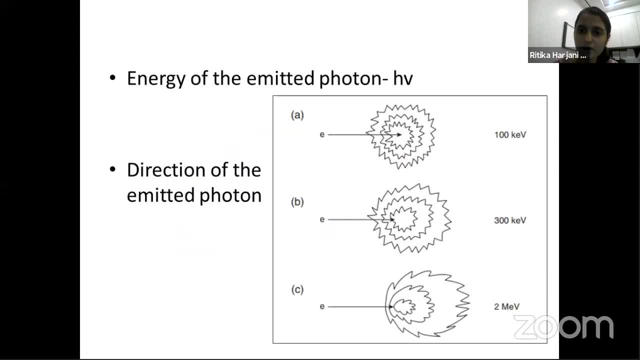 x-rays are produced. an applied point here would be the direction of these emitted photons. they depend on the energy of the voltage that we have applied. so or the initial electron that is coming and interacting with the nucleus, to be precise, so in a lower energy electron, as 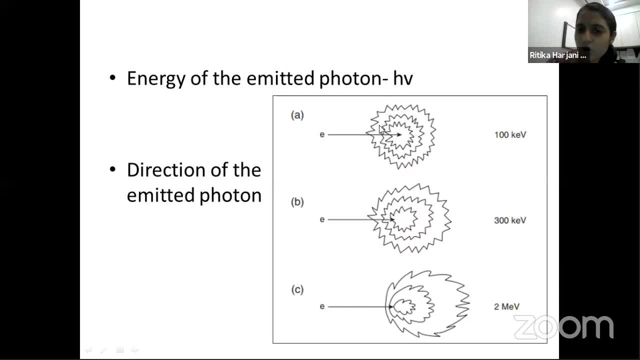 you notice in the figure a part, the photons are going in almost all directions, from the center towards the periphery. it has no particular direction. but as we slightly increase the energy to 300 keV it is slightly forward and when you come to 2 MeV it is much, much forward. 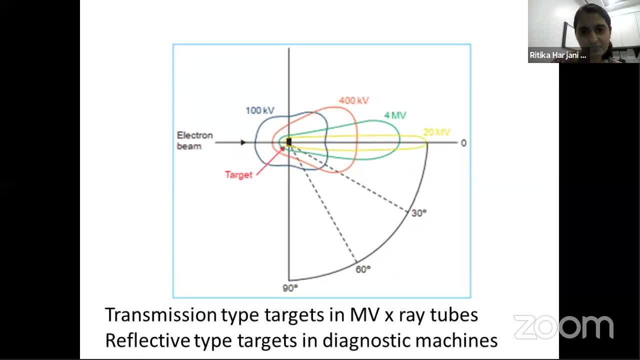 than the 100 keV just in the next figure, same thing. so 100 keV is, as you, multi-directional and uniformly spread. that if you notice the 4 MeV or the 20 MeV, which are our therapy machines, around 6 MeV or 15. 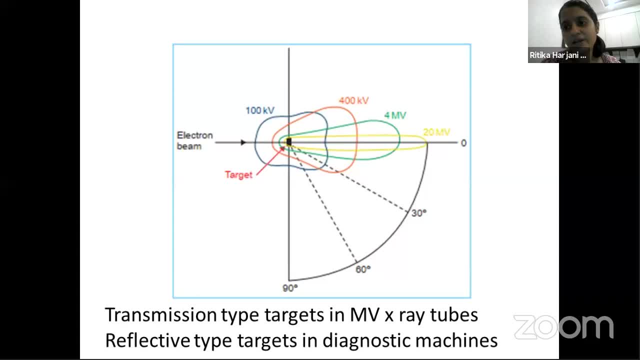 MeV, it is predominantly forward, so when it comes and strikes a target, the x-rays are produced from the opposite direction, from where the of the target. so that is why we use in therapy radiation therapy. we use transmission type targets in our x-ray tubes rather in diagnostic radiology. 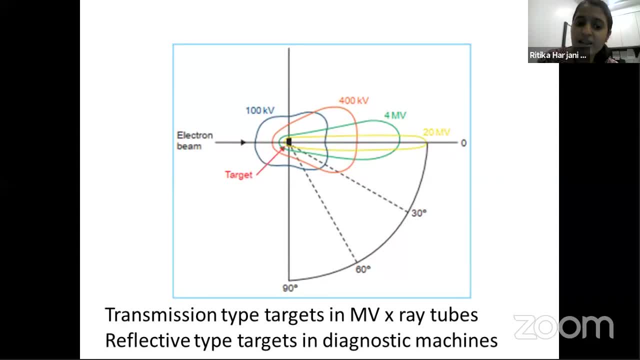 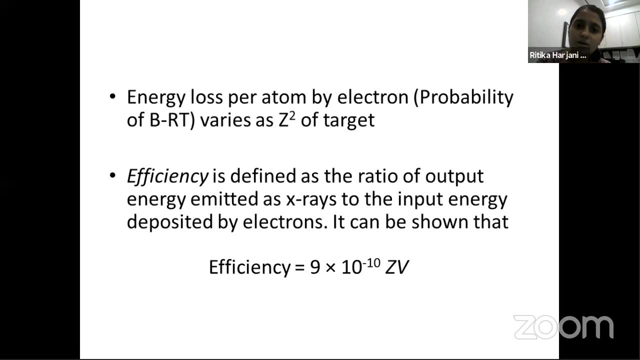 because they are using kV range and they use reflective type targets and not transmission types. then the energy loss for this bremsstrahlung when an electron comes and interacts with an atom, so the energy loss per atom by the electron depends on the z-square. so the probability of 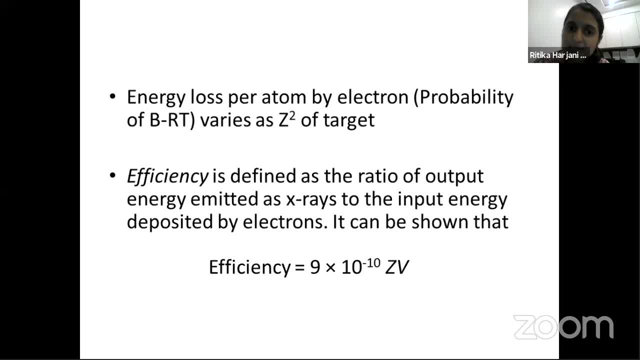 this bremsstrahlung radiation varies as z-square and that is why we want a higher z material like tungsten for the target, so that we have as much as energy loss by the electron to produce a photon or an x-ray. efficiency is basically a term defined as the 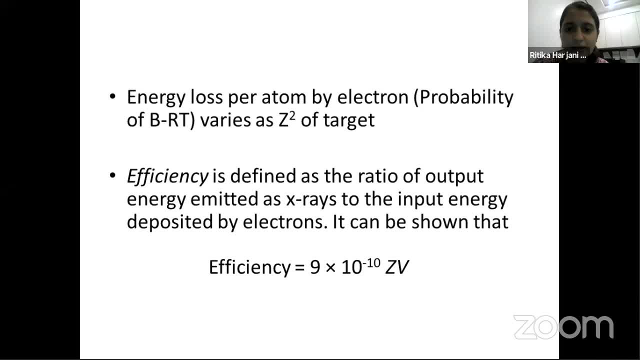 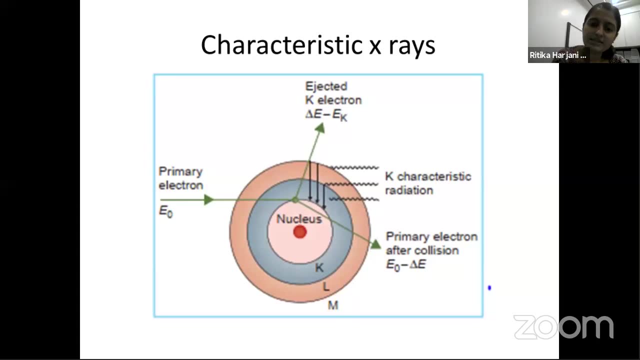 output of photon upon the input of the electron energy, and that does not depend on the square but depends on the z. so that again explains overall using tungsten as the target. another type of x-rays that are produced are the characteristic x-rays. so, as i mentioned, 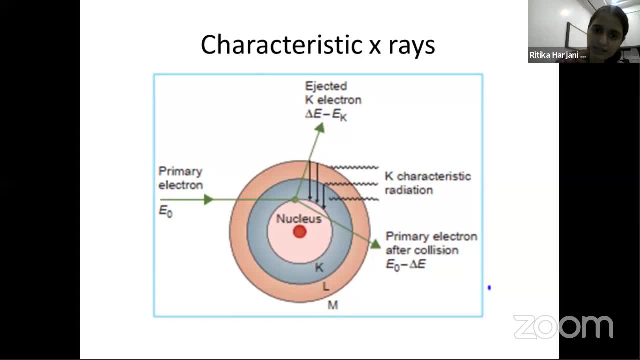 previously. the main point is here the electron is interacting with another electron. so how it does, that is when a primary electron is coming and it is interacting with an electron. suppose an electron comes with an energy e, and it comes and hits this k shell electron, this k shell electron. 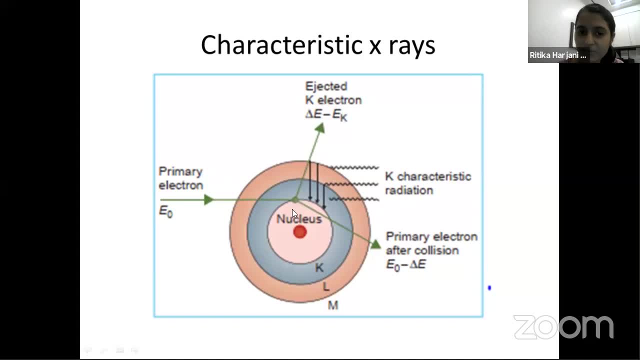 it has removed it from its path and the primary electron is now ejected with its initial energy, e0, minus some energy that it has given off to this new electron. this, because of the energy loss, has changed its direction and this new electron has been released with an energy which is 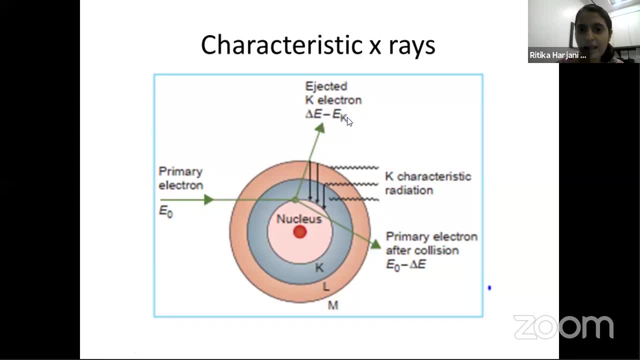 equal to the energy it received from the primary electron, and some energy was given up to. for the binding energy to leave that atom, it required some energy. so now this electron is left, this electron is gone. so there is a vacancy left behind, and because this vacancy needs, 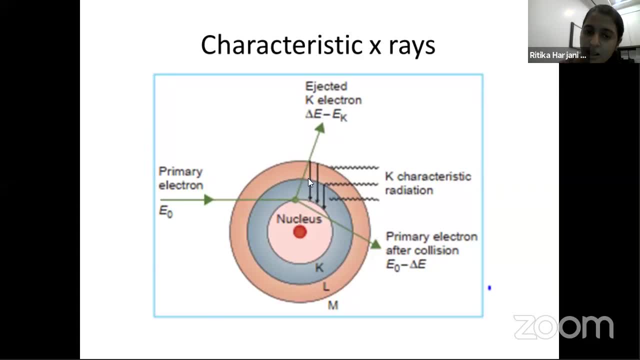 to be filled up and hence electrons from the outer shell come and fall into this shell and in this process they lose some energy, and this energy is lost as x-rays. these x-rays are called characteristic x-rays. now why was the term characteristic given for them? characteristic is because 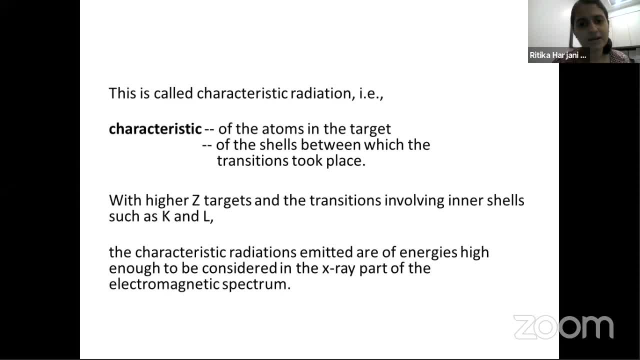 it is characteristic of an atom in the target- a characteristic x-ray of tungsten interaction would be different from molybdenum- and it is characteristic of the shells between which the transitions took place- x-ray transition between l and k shell of a tungsten. and 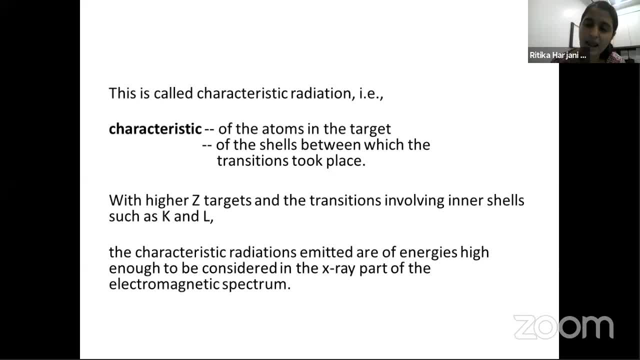 m and l shell of a tungsten would be different. so it's characteristic to the atom and to the shells through which it is taking place, and with high z materials and involving the inertials, the, they are enough to be considered a part of the spectrum, again an applied 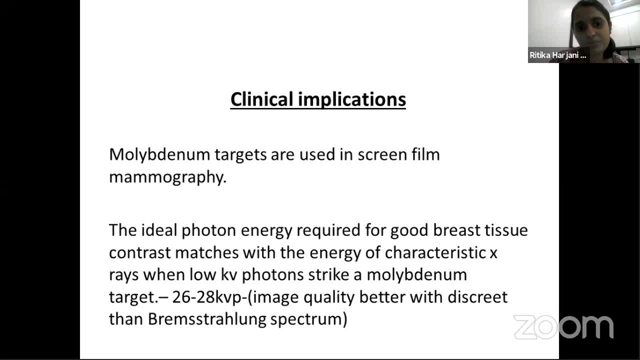 point here would be: molybdenum targets are particularly used in screening film mammography. so when the when there is characteristic x-ray interactions of the electrons in the target, they produce characteristic x-rays of 26 to 28 kilo volts, and that kilo volts are 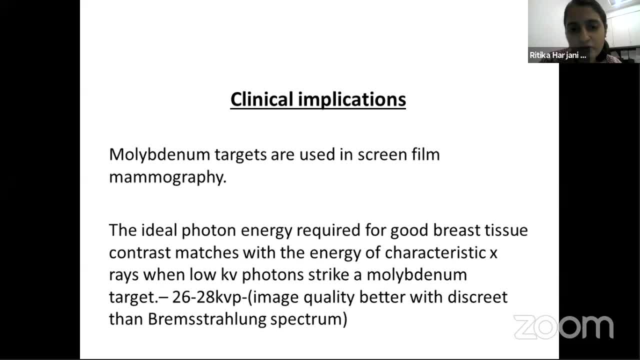 good for soft tissue contrast in a mammogram, and we could have produced this 26 to 28 range of kilo volts through a bremsstrahlung using some other target. but when we use a discrete energy packet, the other photons do not interfere like 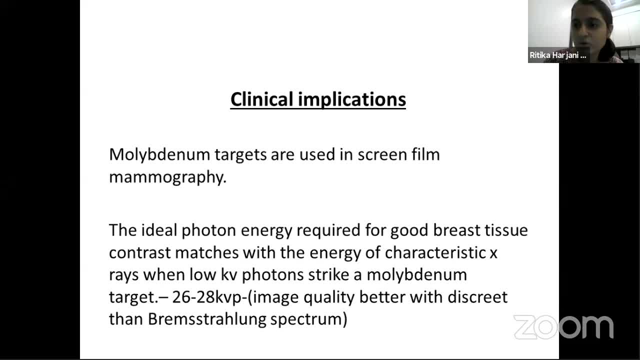 that energy range is ideal for that soft tissue contrast and we do not want to mix up the energy. so that is why molybdenum targets are used in screen mammography to make use of this characteristic x-rays coming to energy spectrum of x-rays. so for 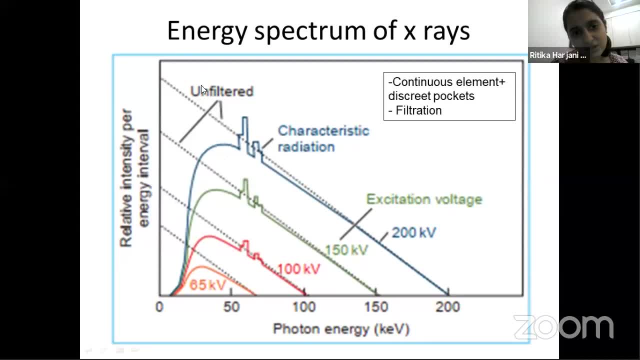 few seconds, we will ignore these full lines and just concentrate on the dotted lines. so, and let's take the blue one where the dotted line is. so, for a 200 kilo volt electron beam or the x-ray- sorry, the x-ray beam- that is produced, it has 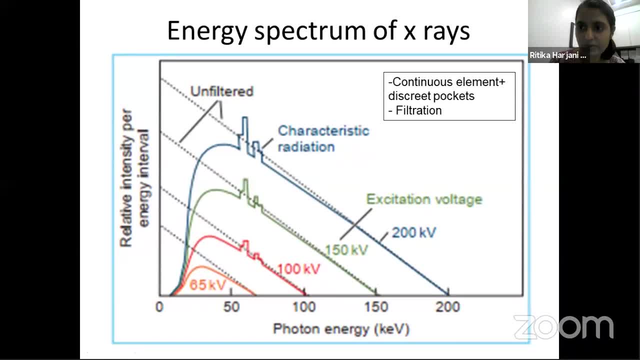 a bremsstrahlung spectrum, as i told it will. bremsstrahlung will have a spectrum of energies, so it will range from nearly 0 to 200 kv. some of the photons when the electron had interacted with the nucleus. not all the electron. some of it is. 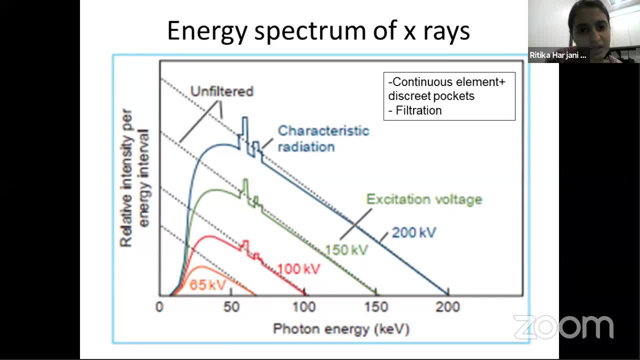 given to the photon. it could be maximum or it could be very minimal, so that entire range of x-rays are produced, and in this tungsten molecule, at particular, 60, around 60 level. these are characteristic x-rays produced, so characteristic x-rays are superimposed. 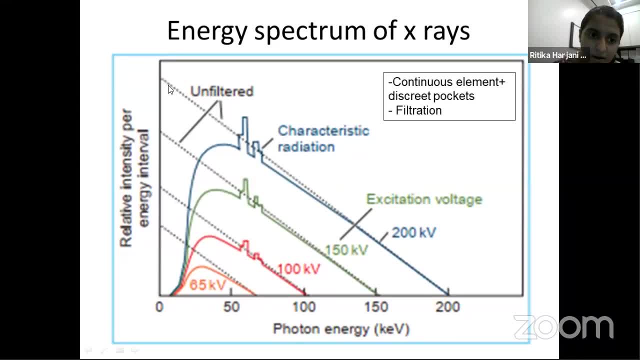 on the continuous. so why, while these dotted lines begin from nearly zero, we add something called as a filter in between, before the emission of these x-rays, so that the low energy now we do not want the 2 kv, 1 kv x-rays to come and complicate. 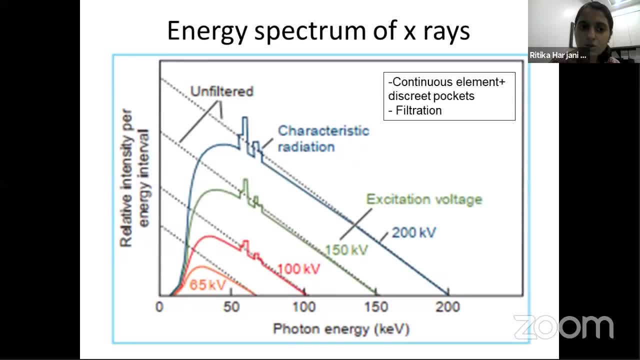 the to interfere with our imaging. so the lower, very low energy x-rays are filtered out through placing some appropriate filters in the beam and hence these solid lines are the filter that we are seeing, after aluminum or copper filters. so filtration basically hardens the beam or increases the 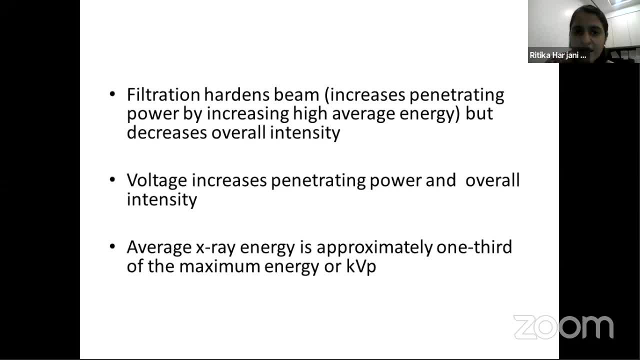 penetrating power. it removes of the very low energy x-rays and so it increases the average energy of the beam. but if you count the overall intensity, because some amount of energy has been removed of the overall intensity decreases in the beam. the voltage increases both the overall intensity. 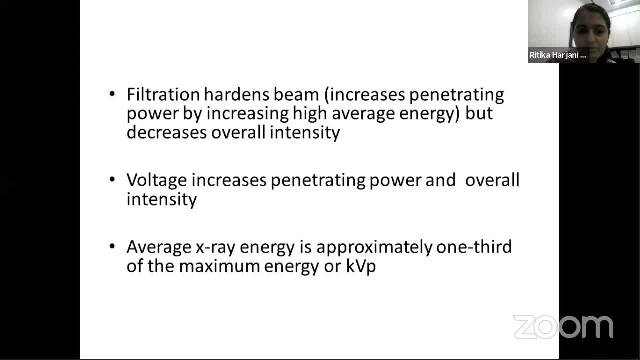 and the penetrating power. and just to remember as a term many times we hear across the time average x-ray energy for any beam. so it is generally one third of the maximum energy. so in a 6 mv linac the average energy would be 2 mv. 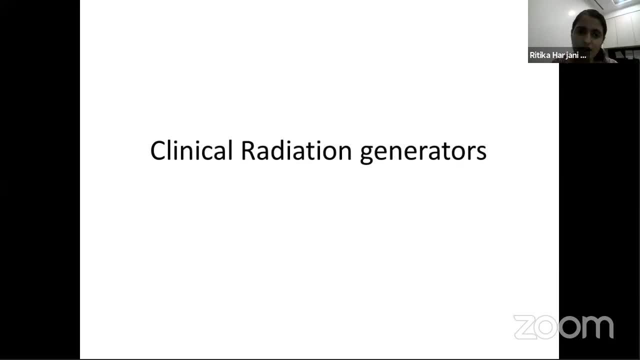 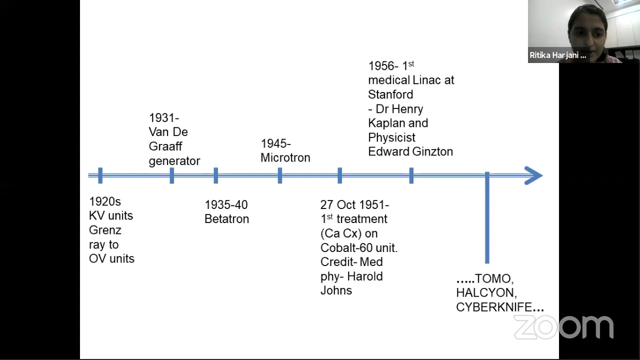 this. with this we cover x-ray production, and now we will go on to the next part of the presentation, the clinical radiation generators. so this is just a brief timeline of things, how it evolved. so in 1920s we had just the kv units and it began with very 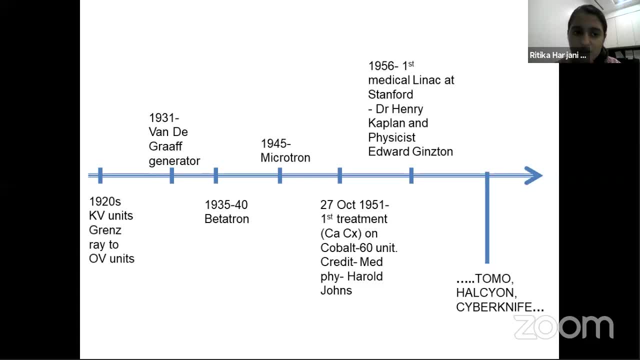 low energies with a grenz rays, 2 or 2 voltage units. we will deal with all of this in detail and then gradually over the years between 1930 and 45 or 50, we had a couple of other accelerators called as vandegraaffs. 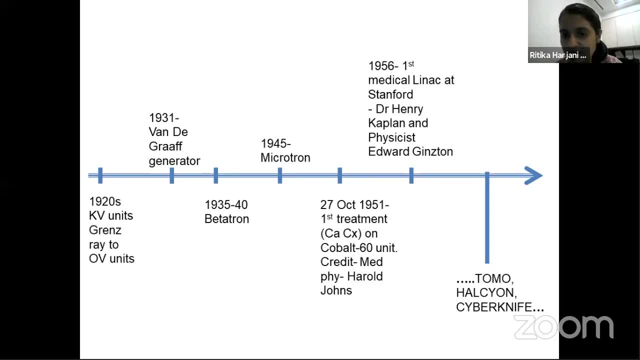 betatron and microtron. then there was a path breaking discovery: in 1951 a first patient on cobalt therapy machine was treated in canada. the physicist harold johns was to credit, who requested the canadian council to help manufacture cobalt sources for teletherapy. 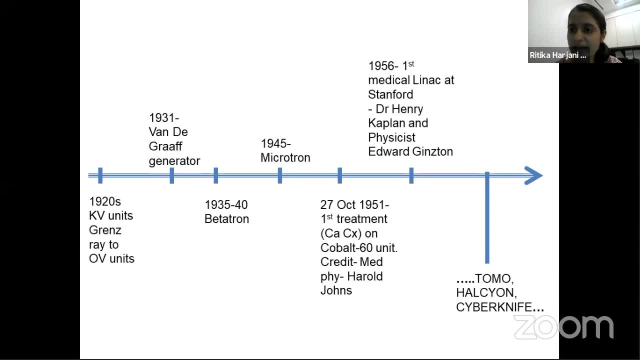 and in 1956 the first medical linac was used, and the people behind it were dr henry caplan and physicist edward ginston, and then, of course, once we have got our linac, we have. we've had tremendous evolution in the linac itself from c arm based. 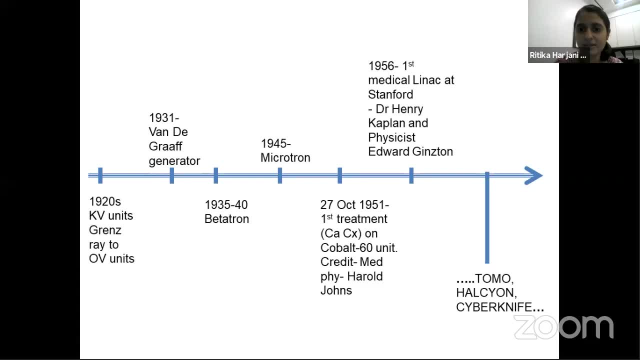 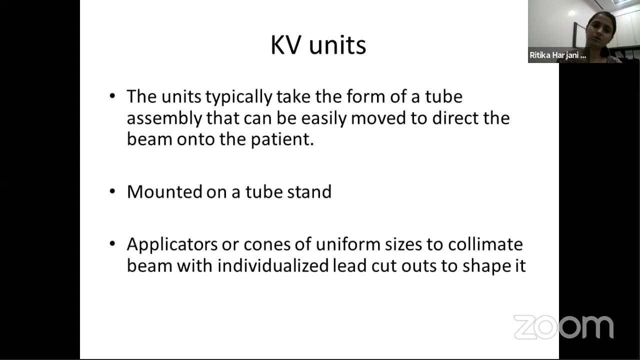 linacs. we have moved on to ring linacs, and then there is cyber knife and many, many machines still coming up. so this is how we have evolved in terms of x-ray unit or the therapy units. coming to the first, the kv units, these units are basically just to 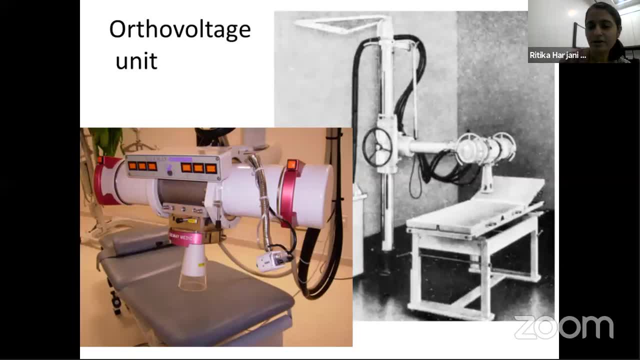 show a photo. they are tube. there's a tube stand and tube mounted and then generally in the end there are applicators of various sizes individualized for each treatment. this is a picture of an orca voltage unit, an old picture, and this is from fm khan, and this is 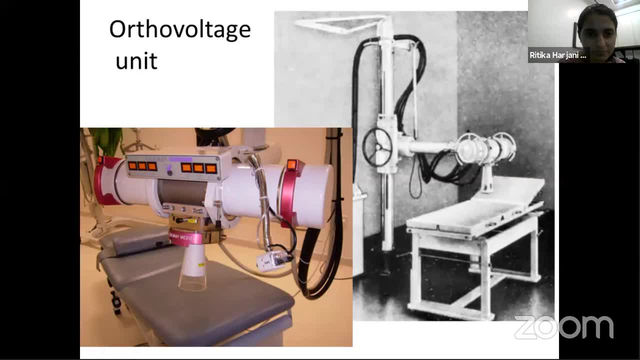 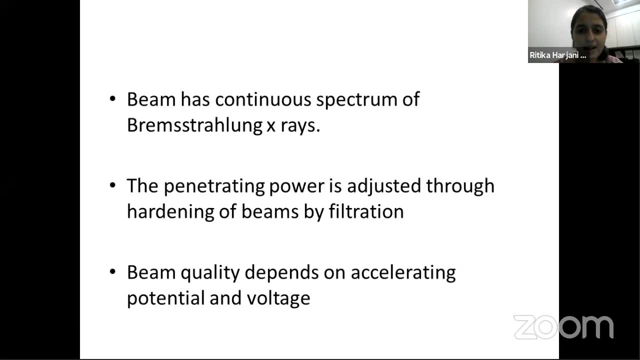 a better picture, just to show the details. so these beams- kv beams- have a continuous spectrum of bramstilling x-rays and the penetrating power is generally adjusted by filtration, and beam quality of course depends on the accelerating potential and the voltage that we apply. this is just a 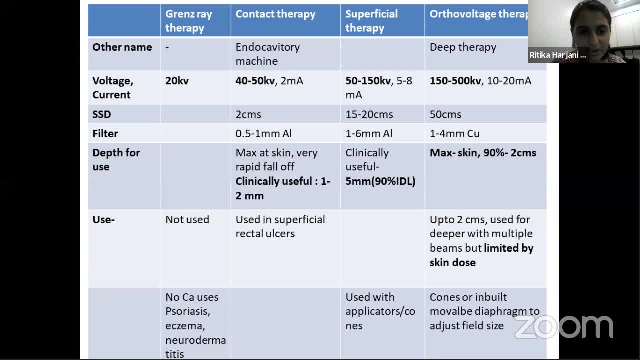 chart from all the material from fm khan, because many times for an exam we didn't i understand many of us, many of the attendees are students. so basically this is just a small table for whatever is mentioned in the book. so we evolved from grenz ray to contact. 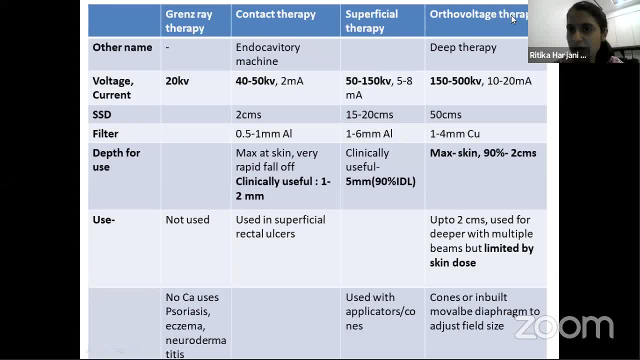 contact therapy, to superficial therapy and to ortho voltage therapy. i have worked with an ortho voltage therapy unit. briefly, very few cases, i would say so. this is something many of us would have seen, but i think this is something. the other three are something not, i don't think if anyone has. 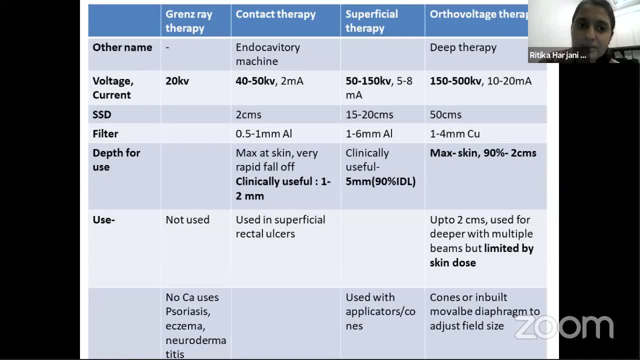 experience in the present era. so what to remember in this is you have is the how the voltage was evolved: 20, it raised from 20 kv to 50 to 150, and now ortho voltage was 150 to 500 kv. so this is one important point to remember. 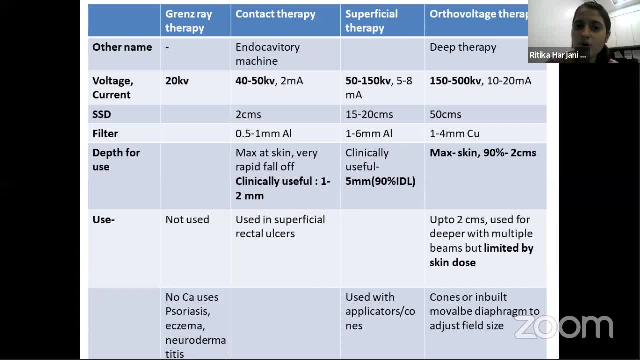 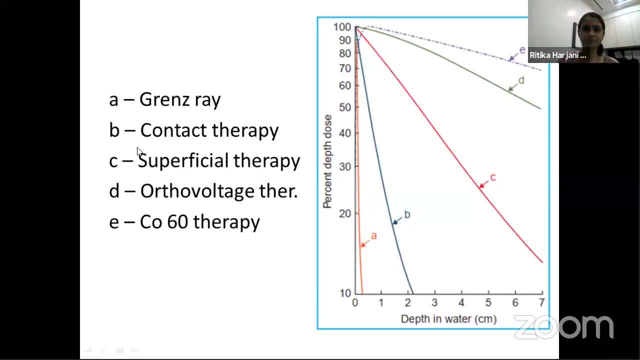 and then, because these are such slow voltage units, the ssd at which we treat is very less as compared to the present 100 centimeters. and another important point is the depth for you, so that i will explain in a diagram. so this is the energy loss in water. 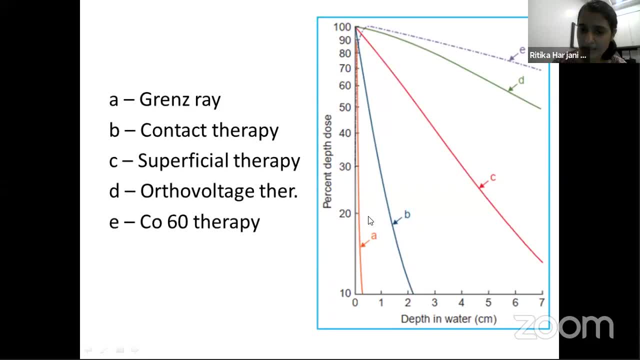 studied in a phantom, and so a here is the grenz ray. this is contact therapy or endocavatory therapy, superficial therapy, c, d is ortho voltage and e is a cobalt beam. so if you notice the grenz ray, whatever is useful is our 90 percent isodose line to 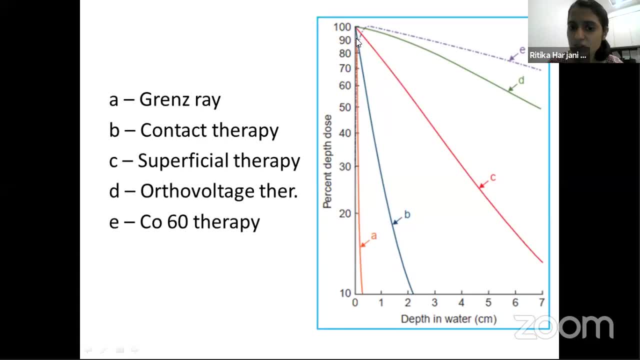 be generous, but generally 95 percent isodose line. so that is just there at the skin for grenz ray. so that is not much of use. it was in fact used for skin conditions in the past like psoriasis, neurodermatitis. not much in oncology. 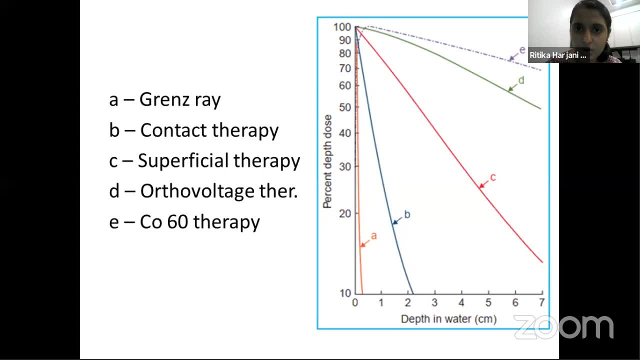 then contact therapy if you. if my cursor is visible, 95 percent would be somewhere around few mm. 1 to 2 mm. so that was in the past used for superficial rectal ulcers and, as we were, superficial therapy generally 5 mm then ortho voltage. 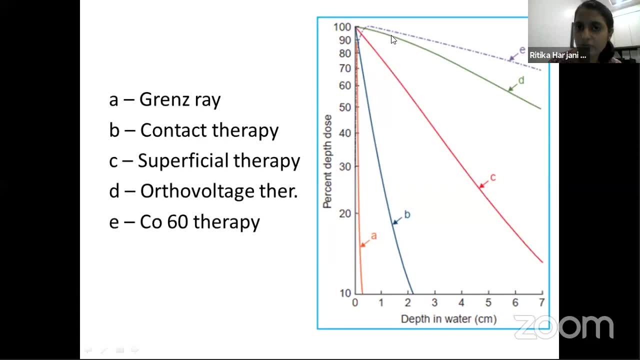 therapy does have some important good coverage- 95 percent till about 2 centimeters- and that was something that was used for quite a while, and so what was done in the past was when the best therapy available was an ortho voltage unit. superficial treatments were comfortable because it could give a 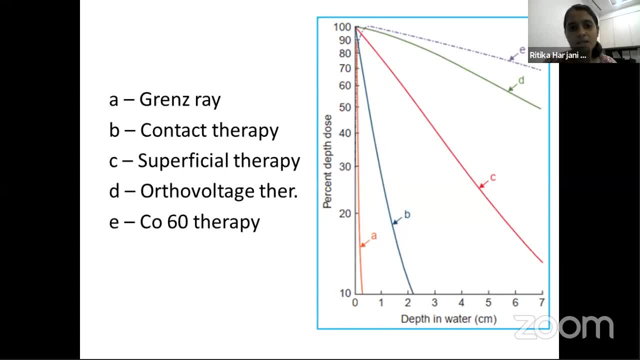 good dose distribution. but deeper treatments were attempted by giving multiple fields from different angles so as to be able to reach some dose or a good amount of dose to a deeper tissue and as much as fancy dosimetry that we have today with the exact number of 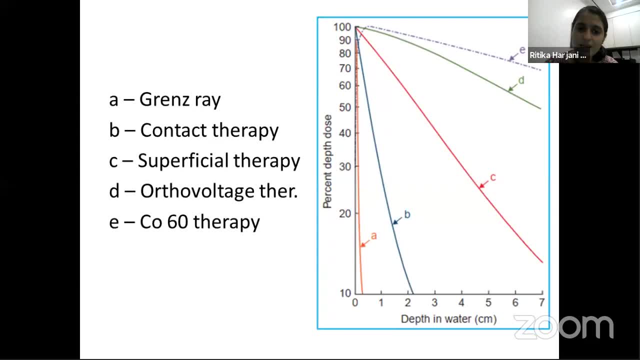 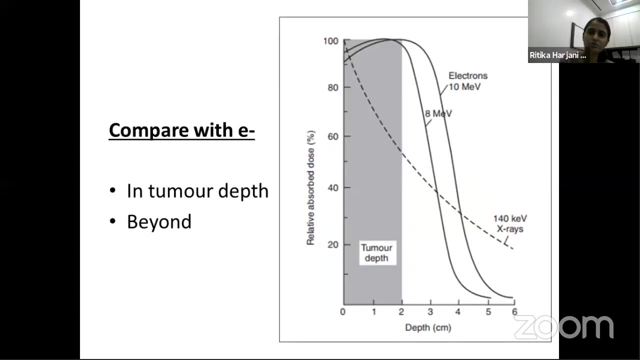 MUs and other things. previously it was more like you give till your skin is able to tolerate. so skin toxicity was a limiting point in the past wherein you had to stop when the skin could not tolerate beyond. in these KV units, when you compare it with an electron therapy, 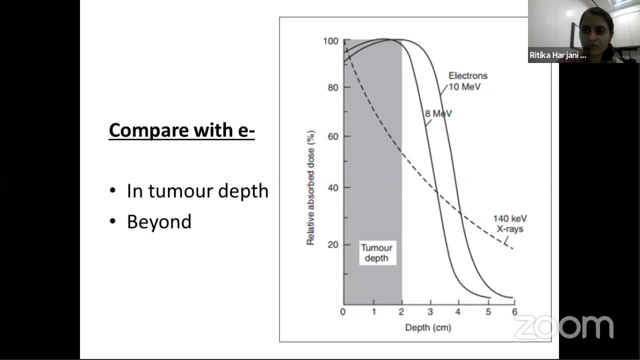 beam. so I would say we should notice that electrons fair better, because if the tumor is at a depth of 2 cm the electron is nearly giving maximum dose or a good amount of dose for that length, and then it generally has a sharp fall off. so in the normal tissue. 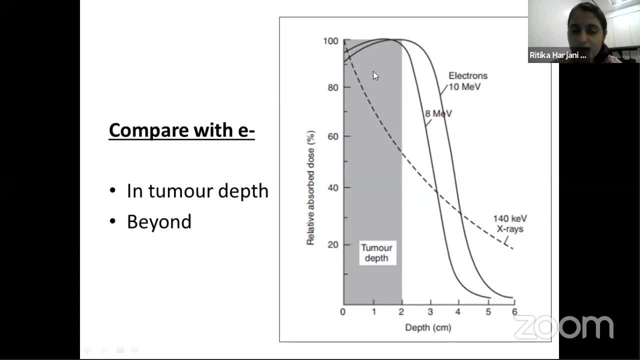 the dose is, the fall off is good, whereas in this KV beam or ortho voltage beam, even in the tissue area there is a fall off of beam and that is continuing in the same manner in the normal tissue. so some of the tumor is under the overdose and some of the normal tissues 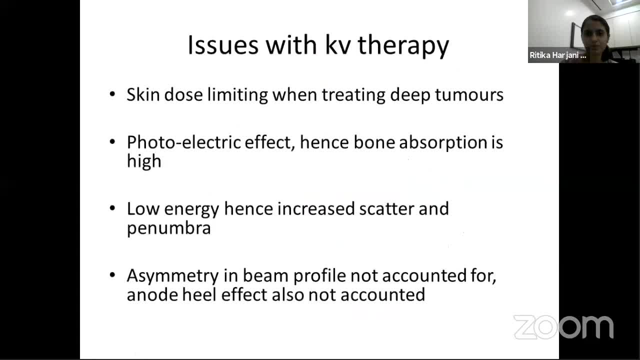 are overdosed when you compare it with an electron beam. so issues, what were the issues with KV therapy? as I mentioned, that skin dose was the limiting and before you could reach a therapeutic dose for your deep tumor, the skin dose would stop you again, as we know. 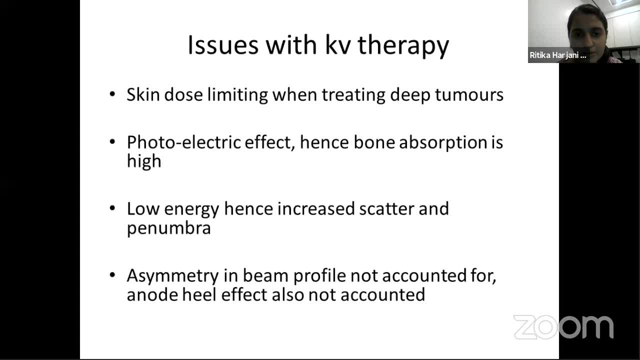 photoelectric effect is active at in the KV range of x-rays. so because of photoelectric effect there was more absorption of the x-rays in the bone and then osteoradionecrosis was much more common than it is today. again, low energy beams are there. 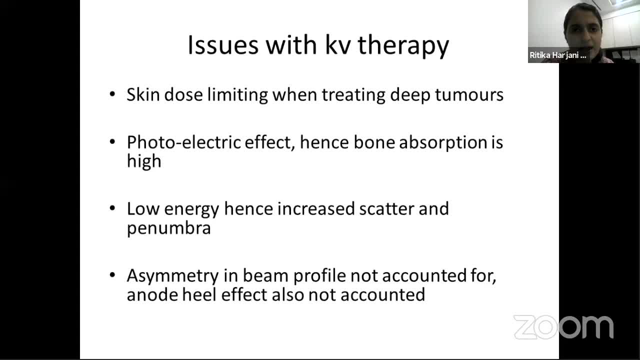 so we are aware that lower energy x-rays have more of a scatter, so the scatter radiation and the penumbra was much more. and then I mentioned about some effects like the anode heel effect or asymmetry, although there was nothing, no mechanisms to to correct for. 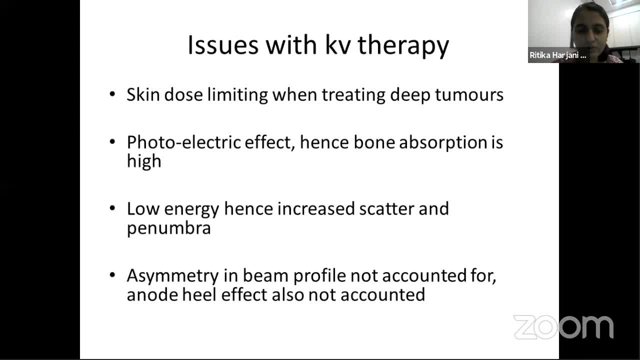 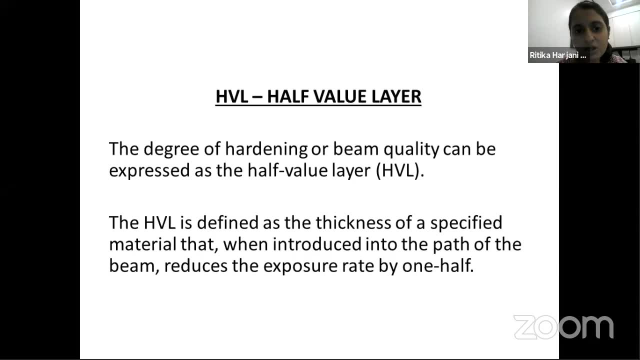 it in the KV therapy unit, so we just accepted what we got. this was just a term that comes across in the entire discussion- the half value layer. so it is basically a measure of a beam quality, and this is defined as the thickness of a specified material which, when placed, 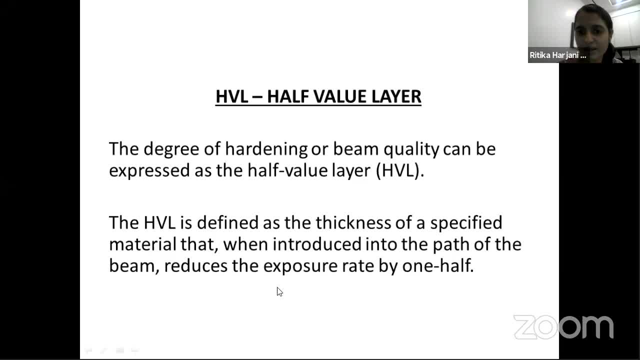 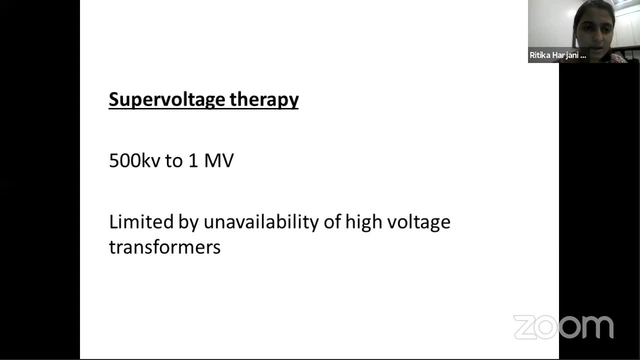 into the path of the beam reduces the exposure rate by one half. then before we got our mega voltage units like cobalt or linac, we also had something, and after the ortho voltage therapy we had something called a super voltage. so it is nearing a mega voltage range: 500 KV to. 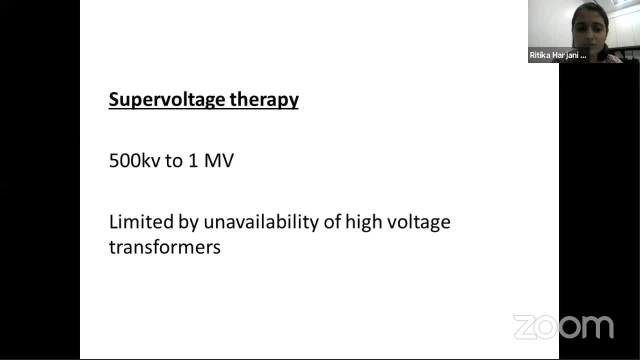 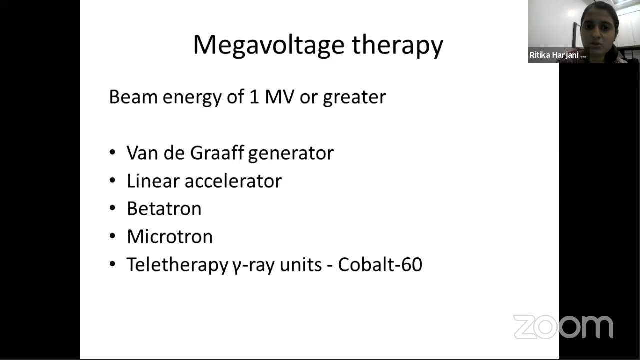 1 MV, but I would say it was not very famous because of problems of unavailability of transformers and it would be like a bridge from ortho voltage to mega voltage units, then coming to mega voltage therapy. so basically any therapy unit with a beam energy of more. 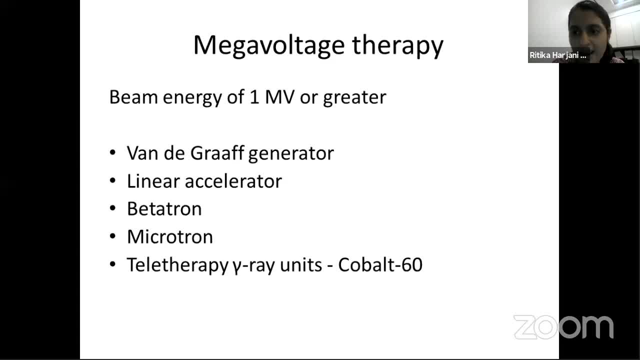 than 1 MV is or more, and there are many that are there in that category. so I would be dealing in detail about the linac today and a cobalt unit. I do not think as a radiation oncologist or an exam going student. we need to know. 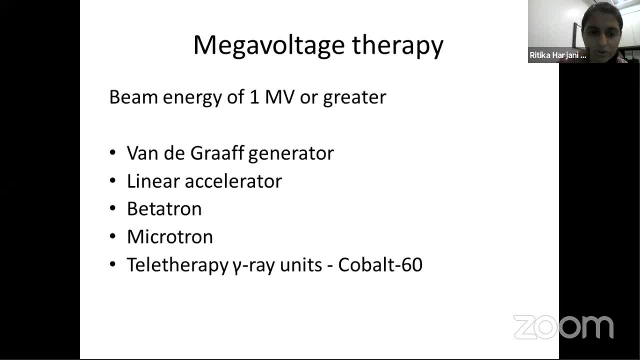 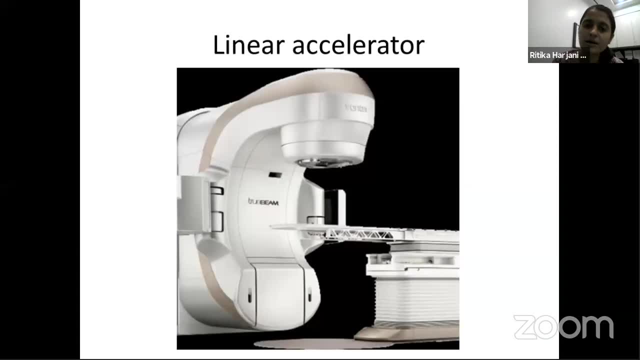 a lot of detail about a Van de Graaff or a beta tron microtron. still, if there is time in the end, and if someone wants to, I will cover it. I will just skip this Van de Graaff. so coming to a linear accelerator. so this: 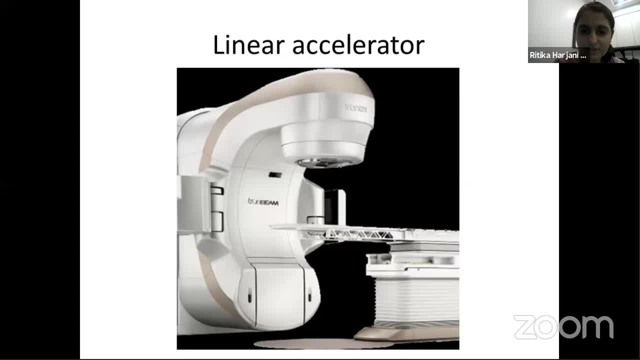 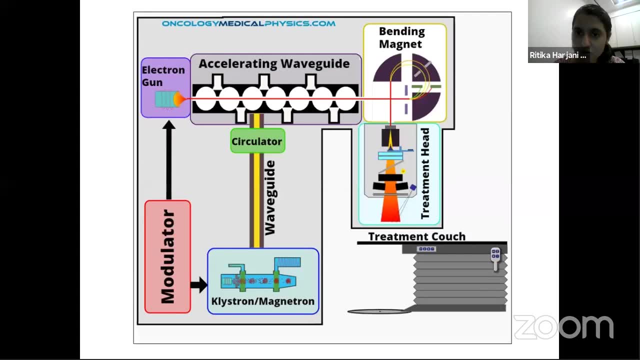 is what we are commonly accustomed to and this is what we go to every day. so what is it inside of this? linac is something like this. so there are a lot of components I would just name now, like the modulator, a microwave source, crystal magnetron. 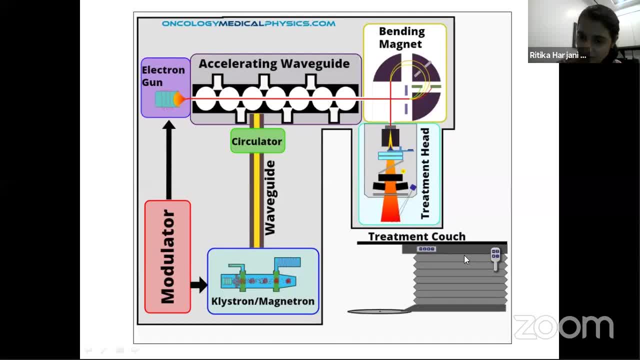 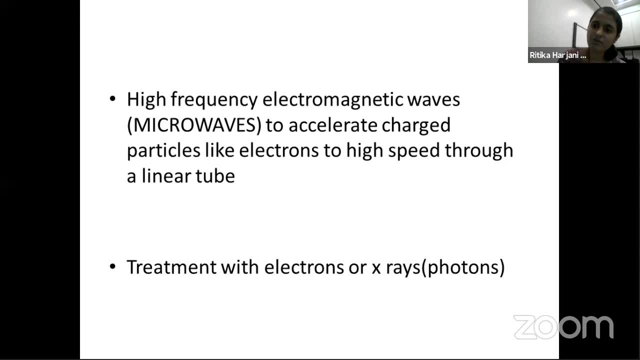 wave guide magnets and a treatment head and a couch. so all this is compactly packed in our linear accelerator, and the basic principle of functioning of a linear accelerator is high frequency microwaves are used to accelerate the electrons, and these electrons then are used for treatment or are made to strike. 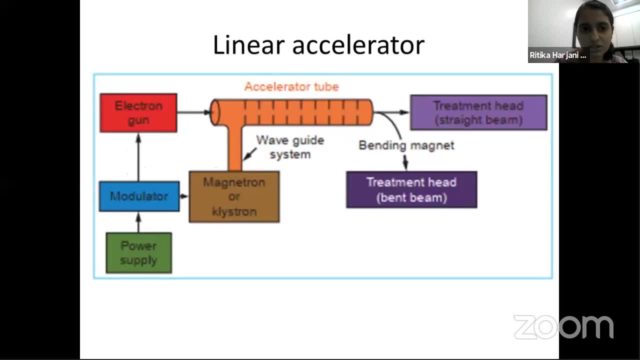 a target and produce photons for energy. so again coming. these are basically a similar diagram with just boxes. what are the components of a linear accelerator? so basically, it starts with power supply. this power supply gives power to the modulator which generates the voltage pulses and it supplies those pulses. 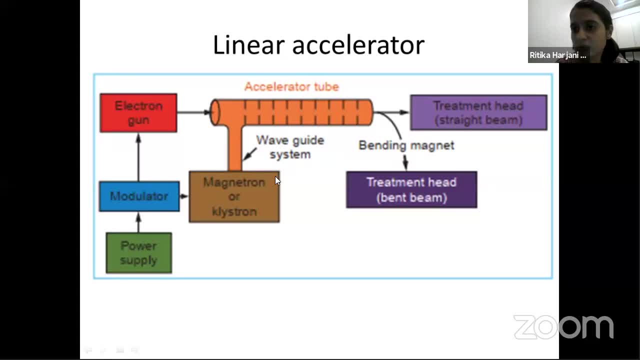 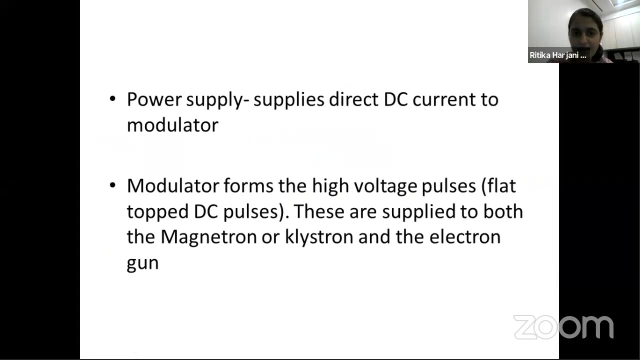 to the electron gun and to a microwave producing source. I would still not go into magnetron or crystal, let's call it a microwave source. and then it proceeds further into the accelerator tube. so this power supply supplies direct DC current and this modulator forms the high 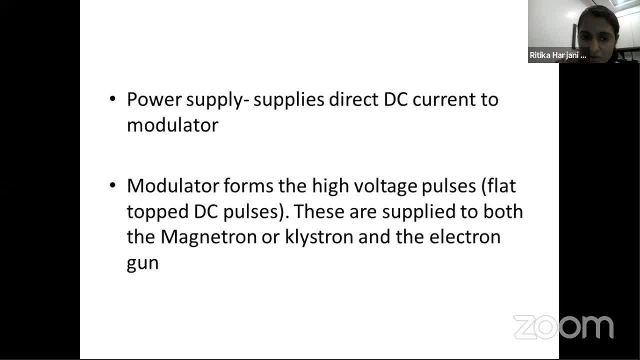 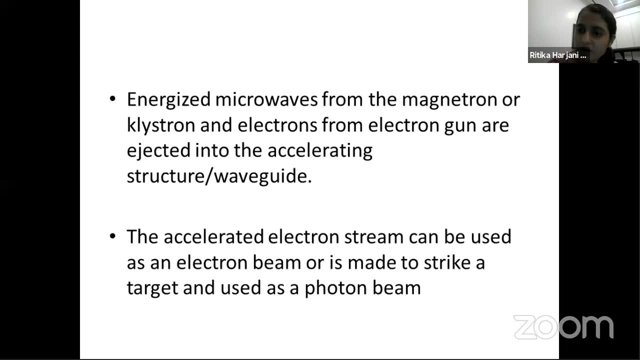 voltage pulses which are supplied, as I mentioned, to the microwave source and the electron gun. the microwaves from the magnetron or crystal and the electrons from electron gun in the wave guide are then sped up, and then these speed electrons and high energy electrons are used to treat. 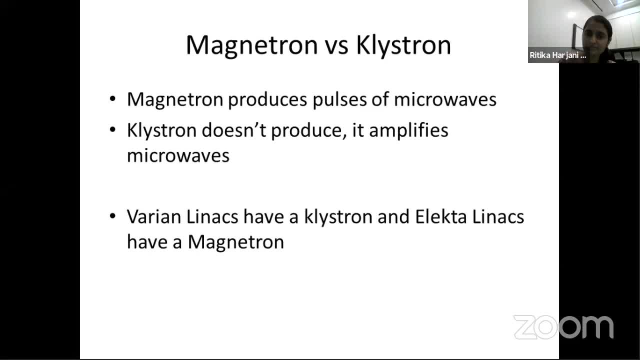 electrons or through photons. now, what is this magnetron and crystal? they are basically microwave sources. magnetron produces a pulse of high energy microwaves, whereas crystal you give a low energy microwave and it amplifies microwaves to produce high energy microwaves. just a point that. 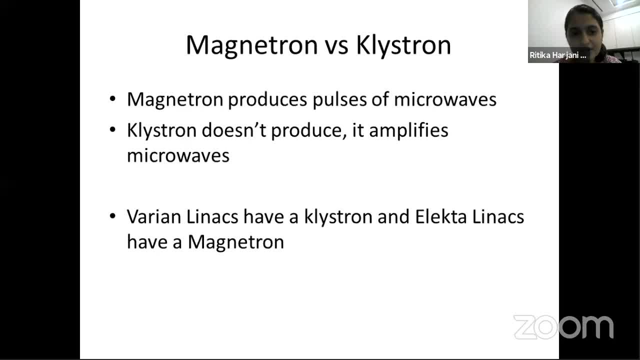 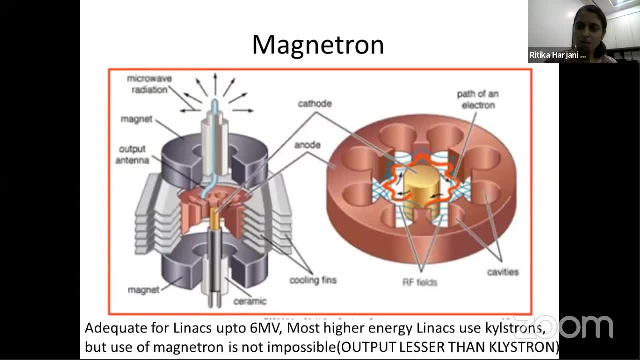 variant. linax generally have a crystal and electron. linax generally have a magnetron. so what happens in this magnetron is basically again, the basic unit remains constant. there is a central cathode and there is a peripheral anode, and an electric field is applied between the two. so 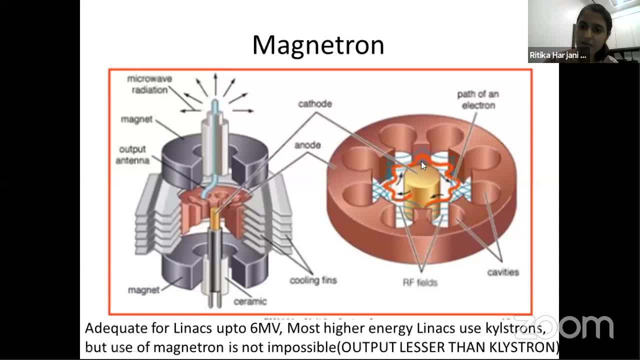 and what is different here is, while the electric field is applied between the cathode and the anode, a magnetic field is applied perpendicular to it. so here, if in the left hand side diagram you can see, there are two magnets, superior and inferior to the cathode anode design. 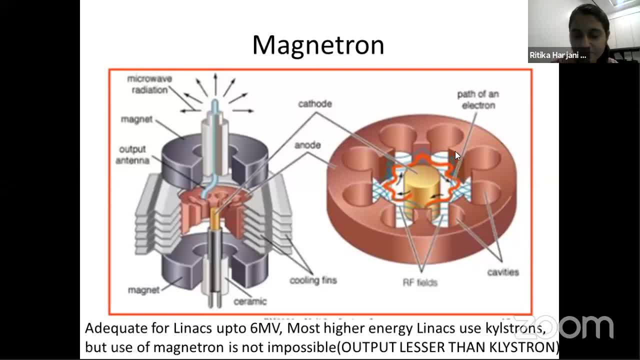 and they supply the magnetic field to it. so when the cathode electrons, when the cathode is heated up or the filament is heated up, it emits electrons and while they travel from the cathode to the anode because of the magnetic field, they tend to take a circular. 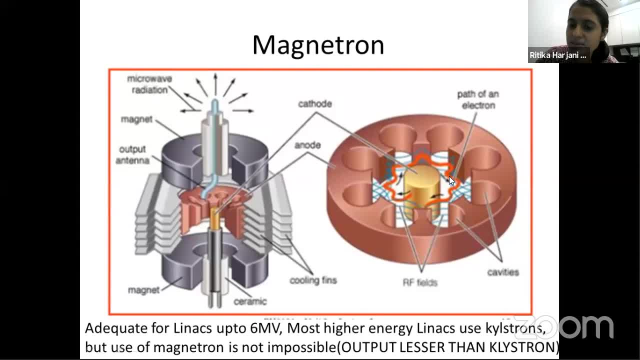 path, and while going in this circular path, some of their energy is lost and this energy is released as microwaves. and then microwaves are released from a microwave output into a waveguide, which takes it to the waveguide, the accelerating waveguide. so magnetron is adequate for linax. 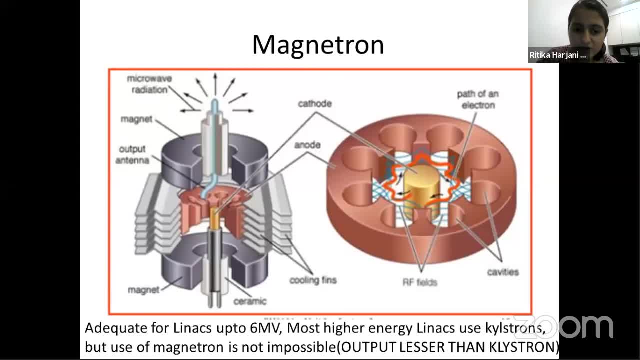 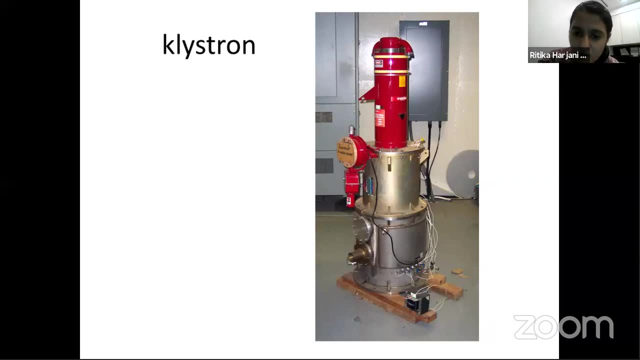 up to 6 mv very comfortably, but are also used for linax of higher energy. but in comparison just said that klystron produces more output than magnetron. and this is the another unit, which is the klystron, klystron which is 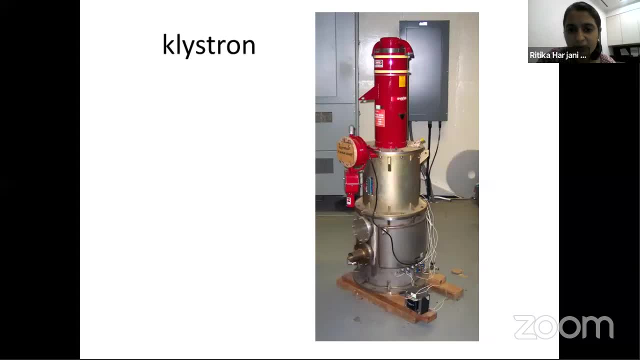 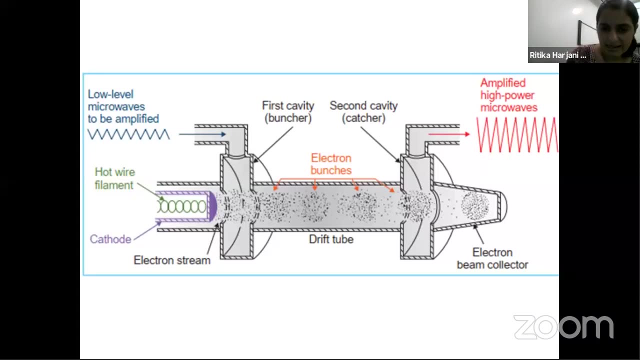 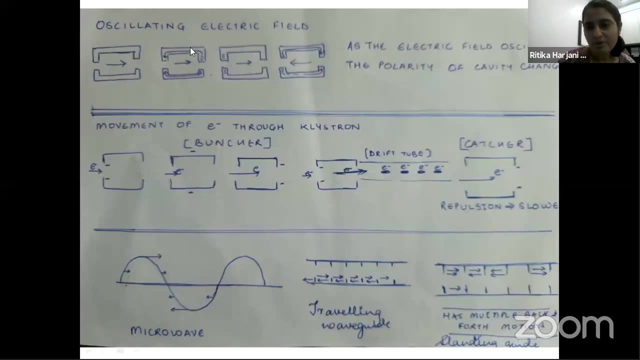 present in variant linax. it doesn't produce microwaves. it is given microwaves and it amplifies them. so this is a slightly complicated diagram, but i have tried to simplify it so my arrows are visible. so what? basically, now we are providing microwaves. 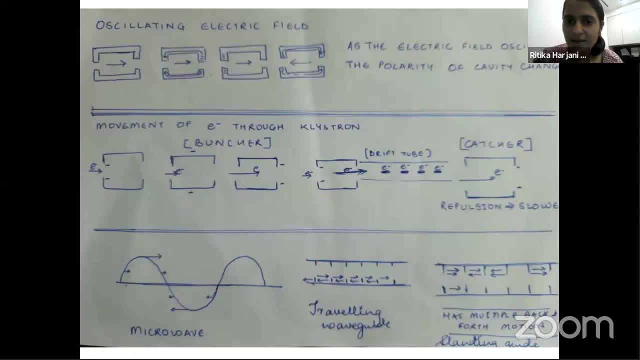 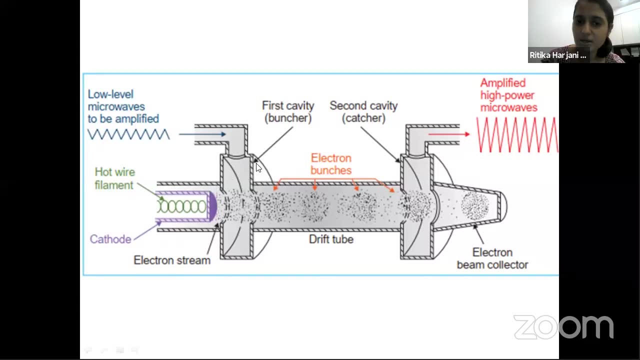 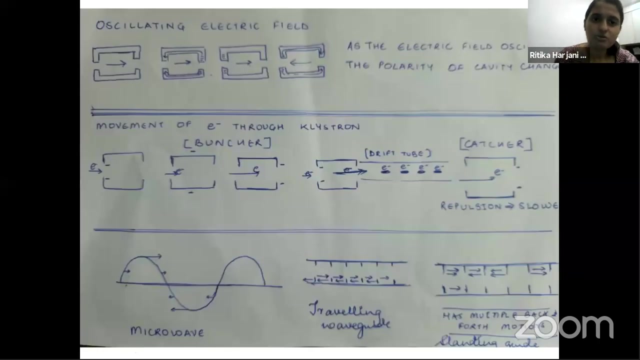 to cavity to, and we have to in this, in this klystron, while we have provided low energy microwaves here, we want high energy microwaves to come out of it. so, while we just to understand what are microwaves basically, they are, of course, waves of. 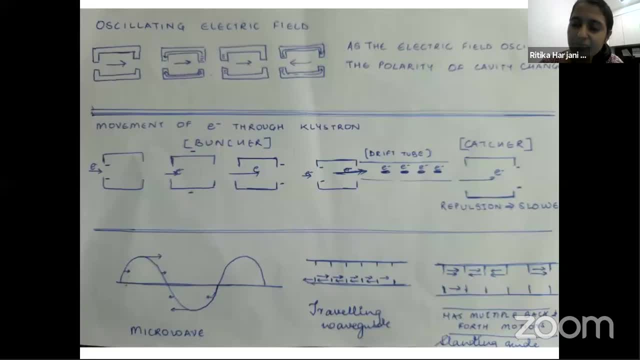 the electromagnetic spectrum, but they have a property that they produce oscillating electric fields is something we should remember. so when we, when these microwaves are inserted into a cavity- by a cavity i mean a metal with a hole inside, with just the walls- it may, of course. yeah, 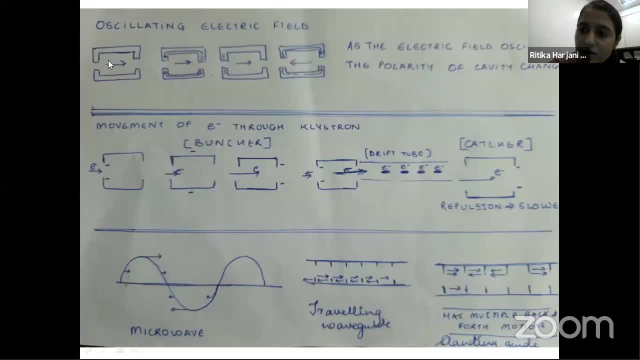 so this: when there is an and it, these microwaves tend to produce an oscillating field. in one point the electrons are moving in one direction, and in the next point the electrons are moving in the other direction, it's producing an oscillating electric field. so now suppose. 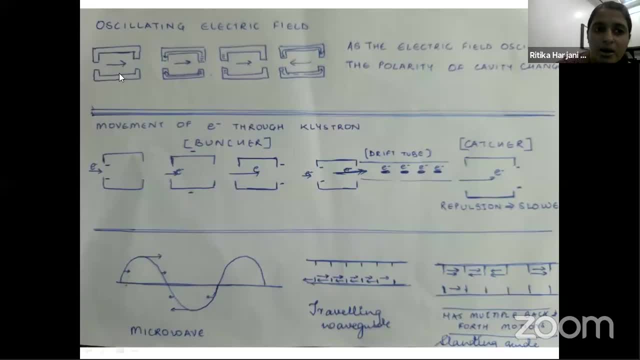 in this cavity, the first cavity in the top, we, there is a microwave which is a produced field in the right hand side direction. then these electrons, because of the field movement, the electron is moving in this direction, these electrons in the right hand side wall of the cavity. 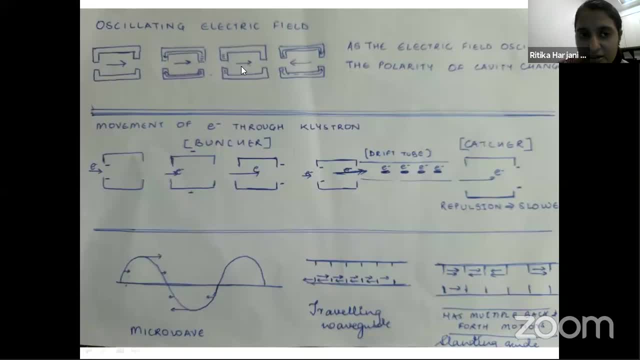 this is still the first same cavity, just in different phases. so this electrons experience a force of repulsion and go back to this side. and now the field is here, but the electrons in this cavity have moved this side. now the microwaves will flip its electrical 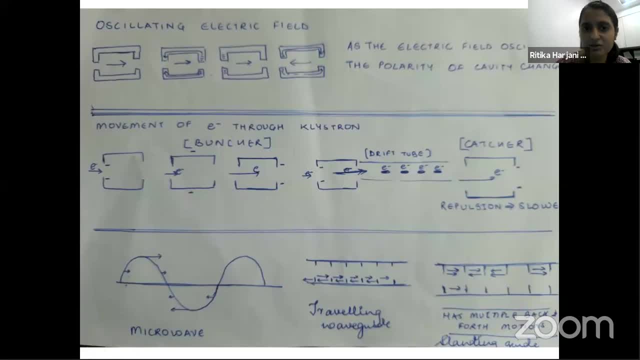 field. so now the electric field is going in this side and the these electrons will be repelled to go to the opposite side. so the, as the electric field oscillates, the polarity of the cavity keeps changing because of microwaves now coming to a clistron. 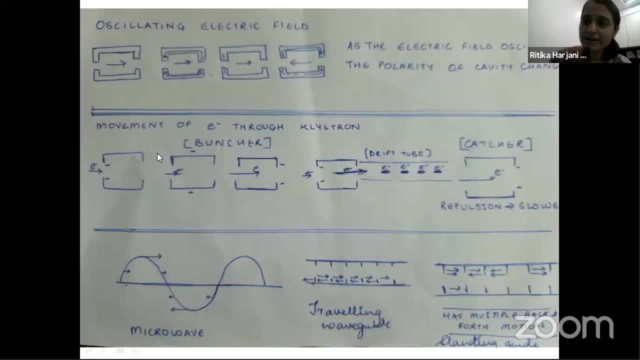 so when now this clistron contains at least two cavities, one is a catching cavity, a buncher cavity, i would say, and one is the catcher cavity, so one is the first cavity wherein these electrons are injected and microwaves are injected, so wherein microwaves are producing an oscillating 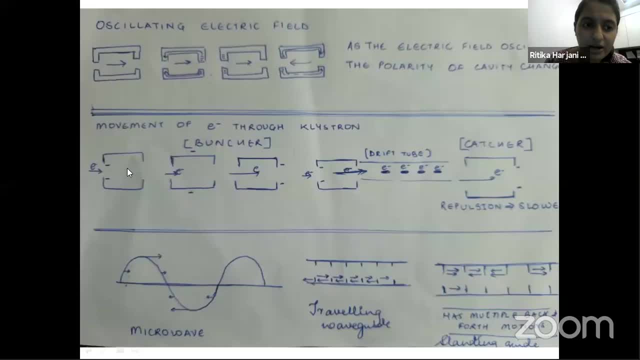 field. so when these electrons suppose because of the electric field cause the, it is negative on this side. so this electron will not pass because it is repelled from it. but eventually then when it flips, when it is goes, this center is going to the negative charge is going on the center. 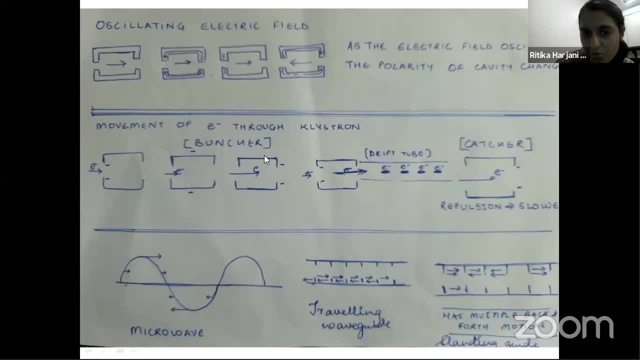 this electron slowly moves inside while the charge electrons are moving from one side to another, and then, when again it flips to this side, this electron gets separated from the other electrons and forms bunches, because this negative charge over here has stopped the other electrons from entering and 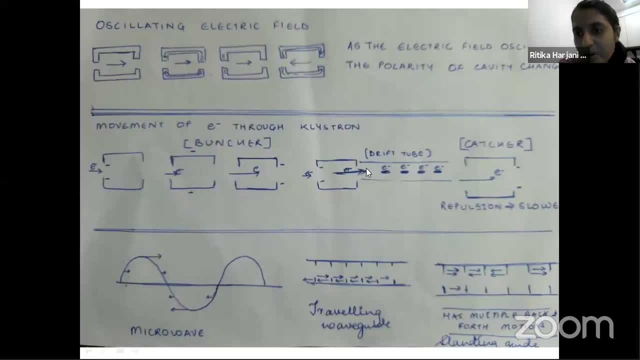 also push these electrons to go further. so that way bunches of electrons are passed which go through a drift tube and in the catcher cavity it is made so that these electrons, the negative end repels the electrons, and these electrons then lose up their energy because of the 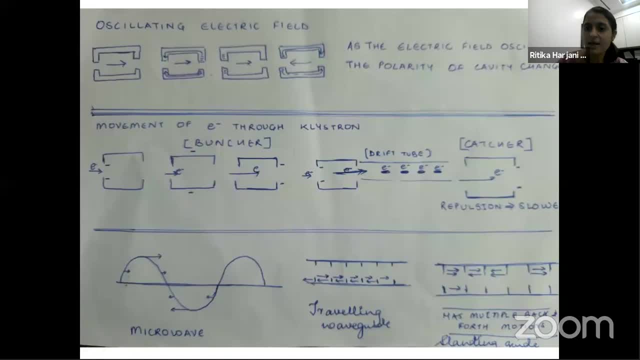 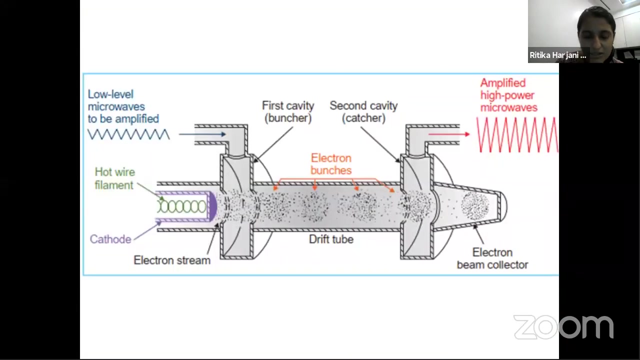 repulsion and these energies are given to the microwaves. basically, this is how electrons are the ones who which give energy to microwaves, and then we remove of these microwaves for our accelerator waveguide to accelerate our the therapy electrons. so this is how a klystron 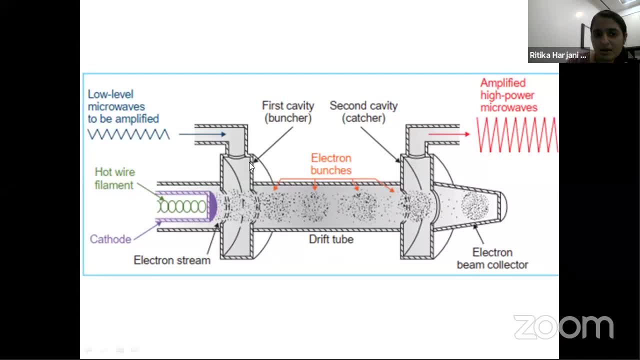 works this? the left hand side cavity, is the bunching cavity, where the filament has given up electrons and then they, because of the alternating field and the alternating polarity of this cavity, these electrons pass forward in bunches and ultimately, in bunches reaches catcher cavity, wherein, because of the 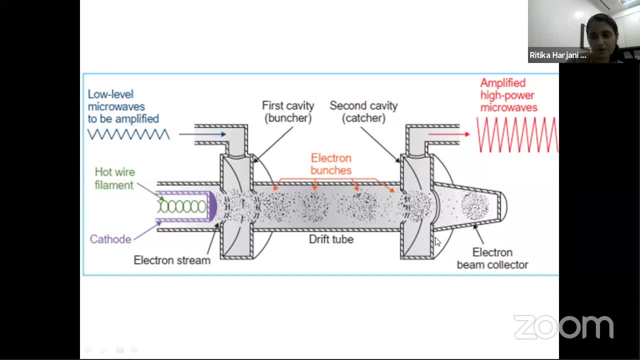 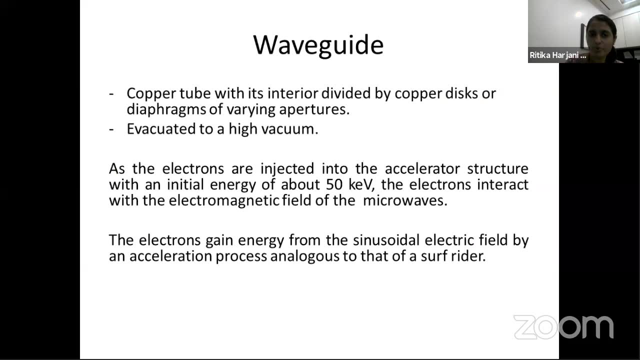 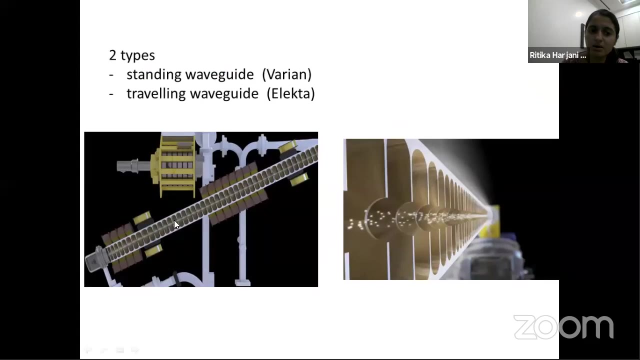 negative charge, they lose energy and give to microwaves. so once that is done, we enter the waveguide. waveguide is basically a copper tube with- just to show photos- a copper tube and with some disks of copper which form varying apertures. in the middle i have a 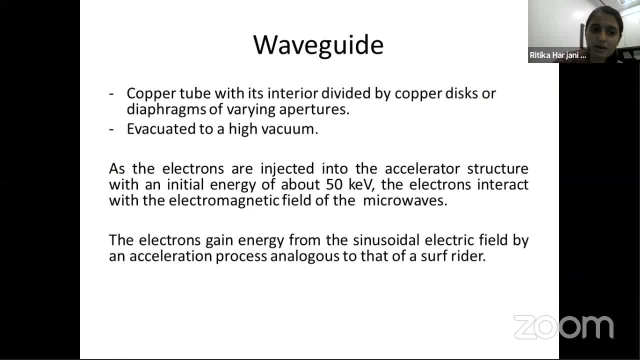 video and some photos to it and as electrons. the electron gun is there which is on one end of the accelerator waveguide. when that is injected, the electrons are injected into the waveguide at an energy of about 50 keV and microwaves which are energized are also inserted. 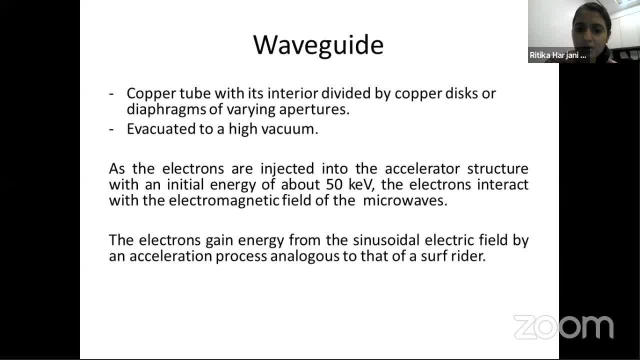 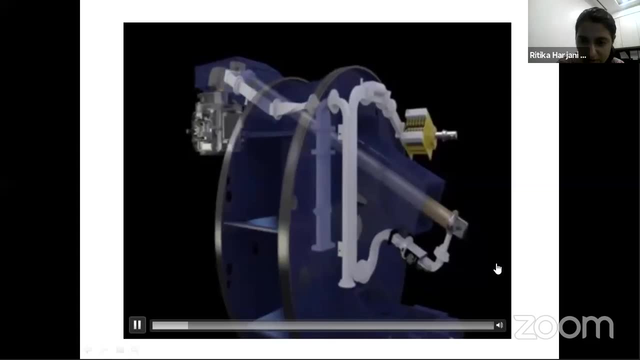 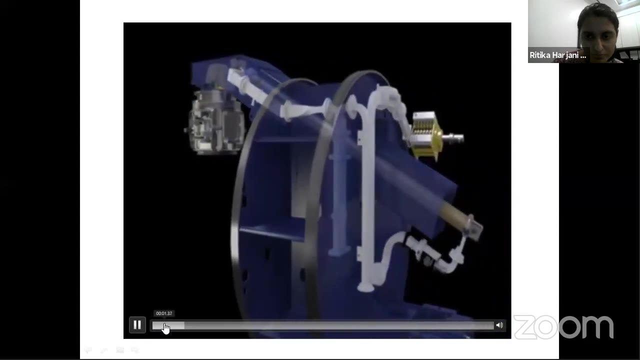 together and then these waveguide enable the electrons to get speeded up and energized while it goes from one end of the waveguide to another. so this is a small video. i will try to put up the volume waveguide. by the magnetron generation, radio frequency waves are pulsed. 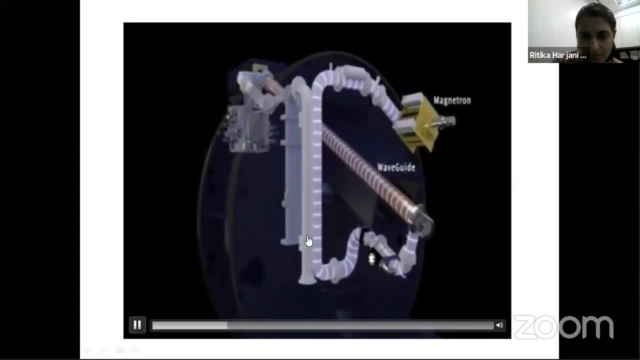 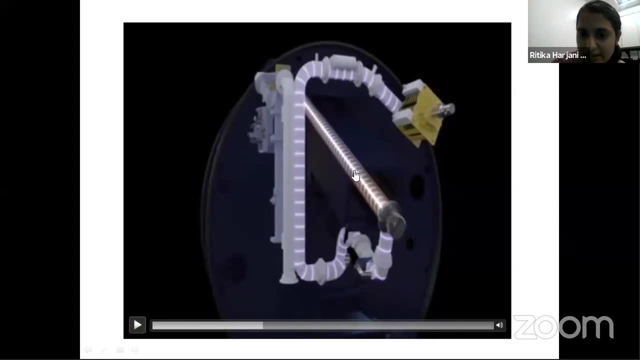 into the waveguide by the magnetron. this is synchronized with the injection of electrons into the waveguide by the electron. so this electron gun is over here which is injecting the electrons into the waveguide and this is a magnetron based machine. so the magnetron 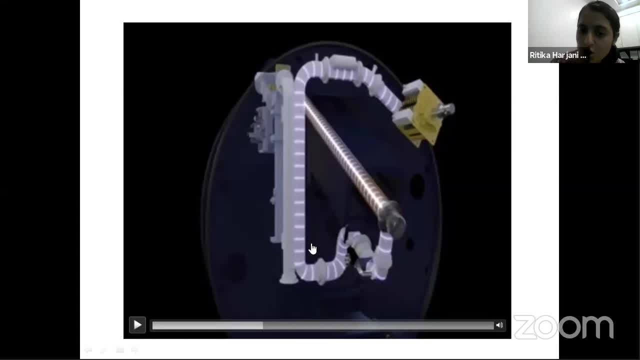 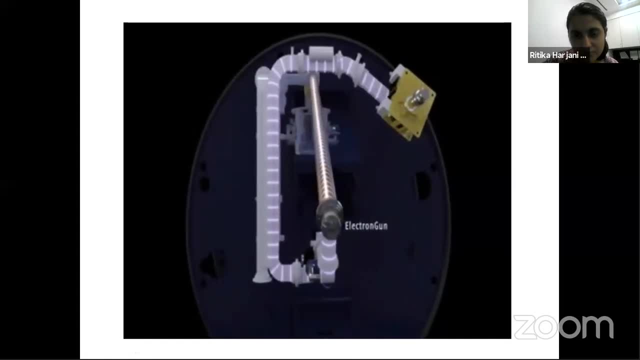 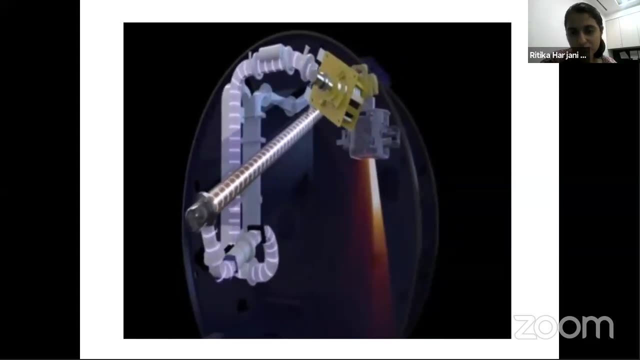 gives microwaves which are carried by another tube to the accelerating waveguide done. the radio frequency waves accelerate the electrons along the waveguide to a speed approaching the speed of light. the x-ray beam is created when the electrons hit and interact with a constant target at the opposite end. 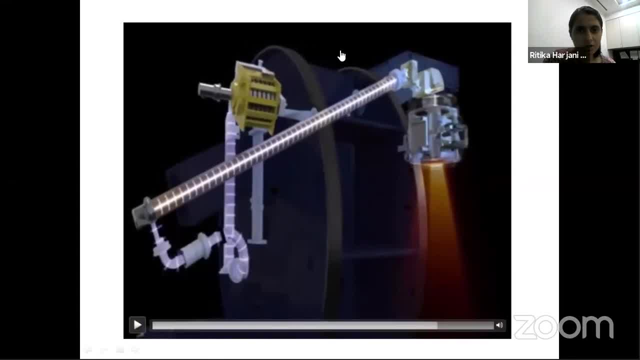 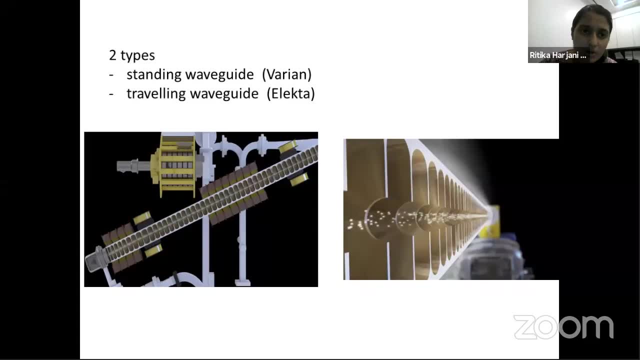 the magnetron controls the power. so this is how basically it functions. the entire circuit is. there are two types of waveguides: a standing waveguide and a travelling waveguide. then it's: electa generally uses a travelling waveguide and variant generally uses a standing waveguide. 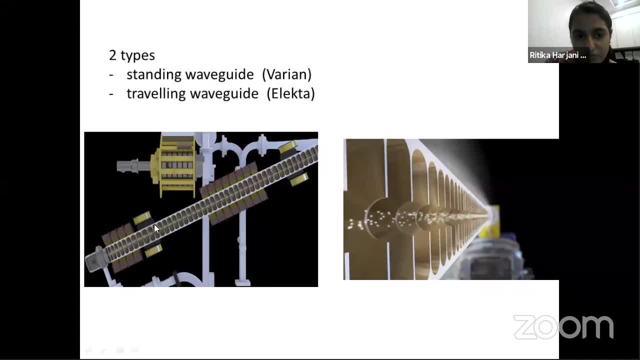 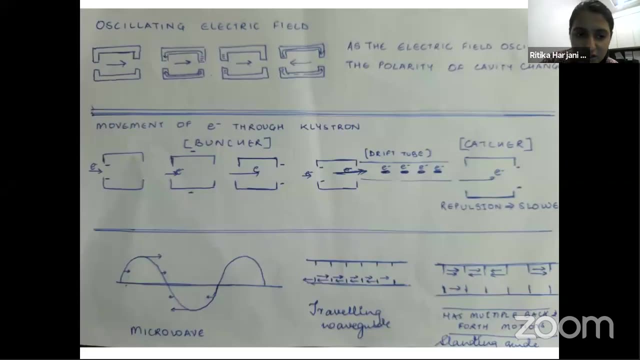 these are just pictures, cross sectional view of the waveguide and just animation of the electrons actually going through the waveguide. so just to explain how these travelling and standing waveguides function is: these microwaves are basically waveforms of energy, so they have a peak and a 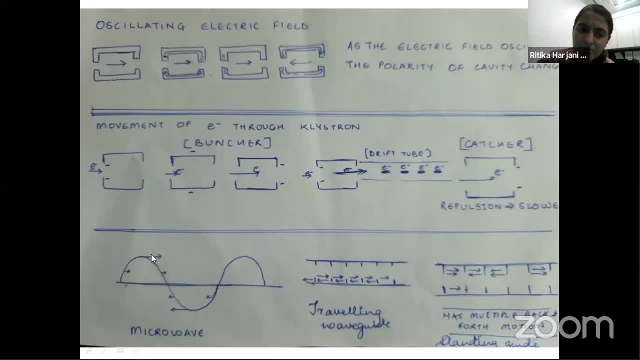 drop, so in the peak it has maximum velocity. this direction in the forward direction, in the drop in the opposite direction. so the electrons are injected in the waveguide, accelerating waveguide, at such a point where the microwaves frequency and the electrons frequency resonate. there is 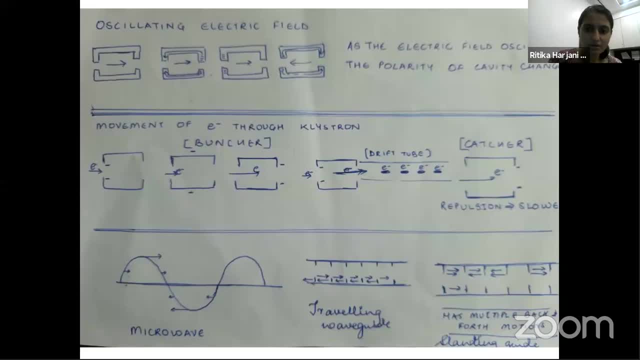 resonating frequency and they are kind of. you can imagine that they are given at the peak. so then they. it said that they like the surfer rider of us surfing person. he takes up the energy on a wave form and is accelerated forward, whereas in a standing waveguide. 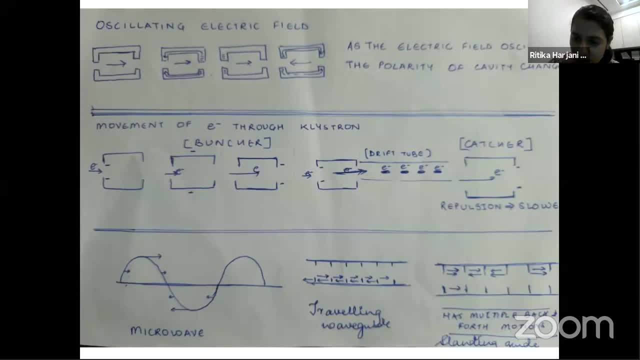 the waveguides the microwaves are given are inserted from the center going to both ends, and then charges are created in such a way that the electron moves forward as the microwaves switch its polarity of the cavity and this standing waveguide, the electrons in the 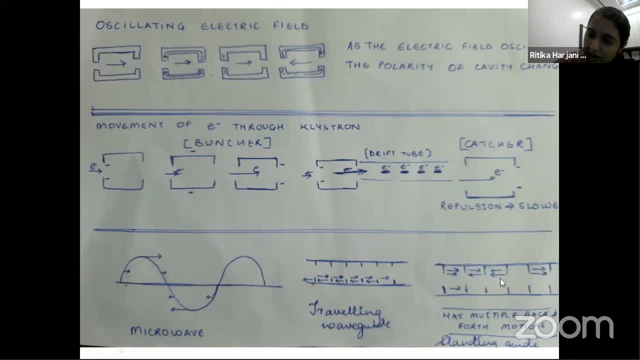 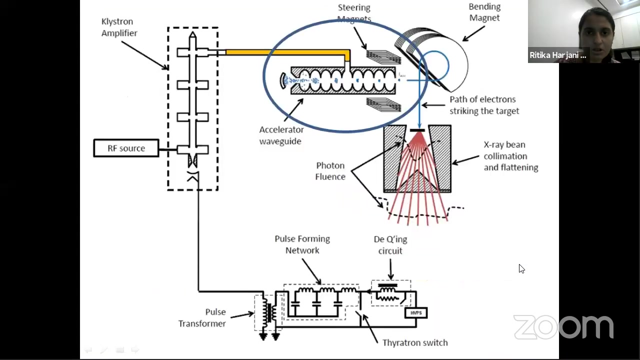 standing waveguide and the microwaves. they go from one direction to the other direction multiple times before emitting out, so the energy or the speed of the electron energy gained by the electrons is much higher. so, in the entire scheme of things, while we have given the power to the 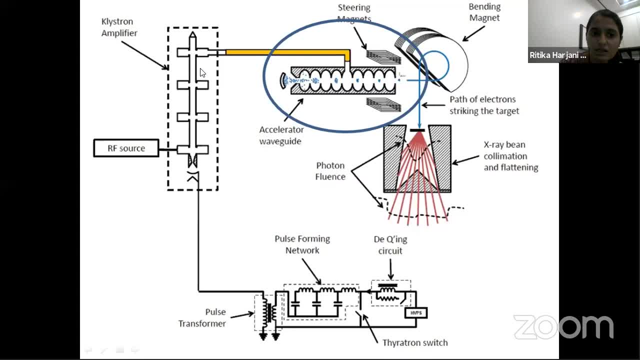 modulator to the modulator, and then we have had a magnetron, and then these microwaves are carried to the accelerating tube. from the accelerating tube we get now a thin electron beam. this thin electron beam then passes into the treatment head to produce a therapy beam. so this 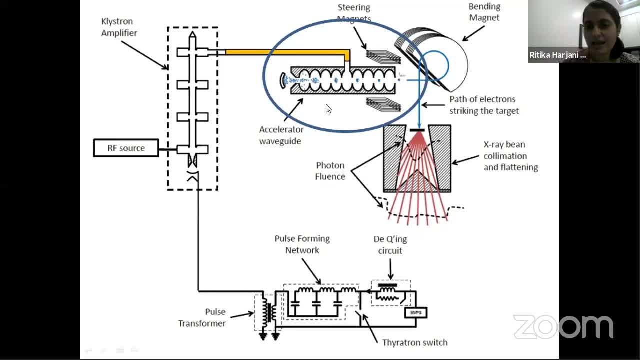 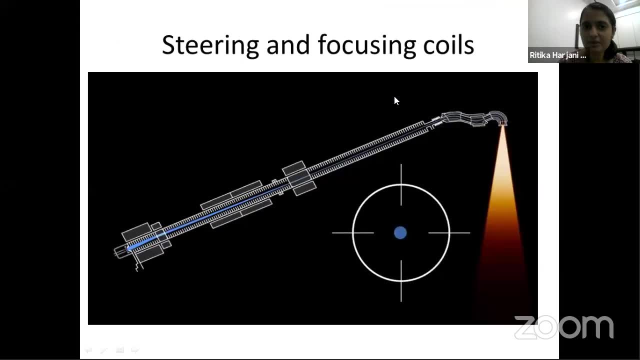 is the. this blue circle shows the the position of the accelerating waveguide in the end. we see here that there is these magnets, so these are basically stirring and focusing magnets around the waveguide. these stirring and focusing so this: if you notice this blue electron beam in the center, 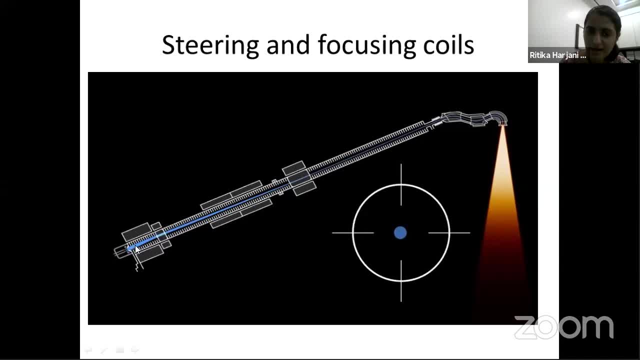 it is quite thick at one end and as it passes it is made to be very precise and go and hit. it's like a pencil beam to go and hit the target at its particular focal spot. so these stirring and focusing coils would steer the beam to help it navigate and 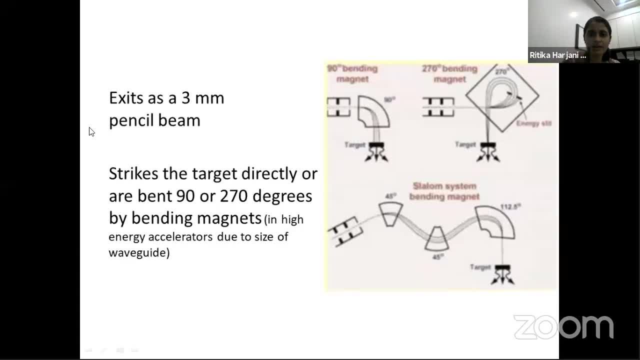 focus it on a particular point. when it exits, the beam, exits the waveguide. it is a 3 mm pencil beam and it is made generally. these waveguides are quite large in size and that is why it is logistically or technically not possible to have the gantry. 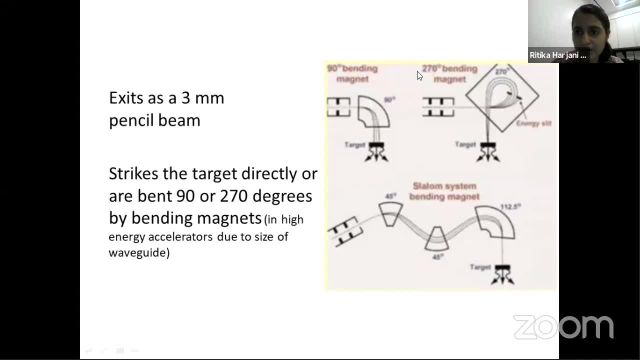 still in the forward direction, so it is made to bend into the treatment head. we say machine head. so again it is bent, sometimes just 90 degrees, or sometimes it is made to take a 270 degrees turn to come down. and now there are modern, more machines. 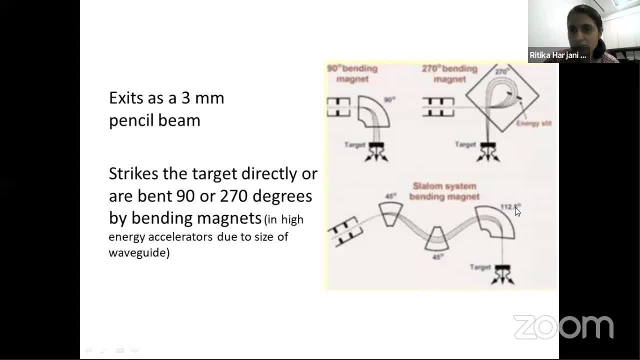 with more complex form of turns. so why these 90? appears to be the most simple then why go on to these complicated turns? is because then you have a chance to bring in more magnets in place. generally these are 3 magnets. in this diagram it is not visible, but I will show you in a further. 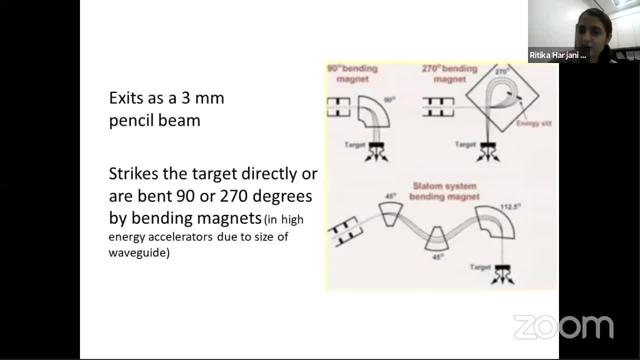 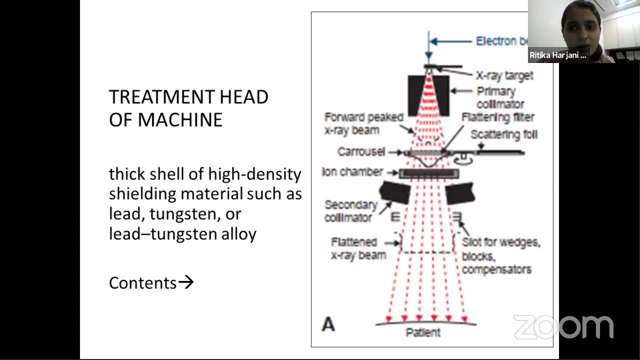 diagram. there are 2-3 magnets in this 270 degrees bending magnet which help to again focus the beam onto a particular point, and once then the next step is it comes and strikes the target. now target onwards things, or the components are in the treatment head of. 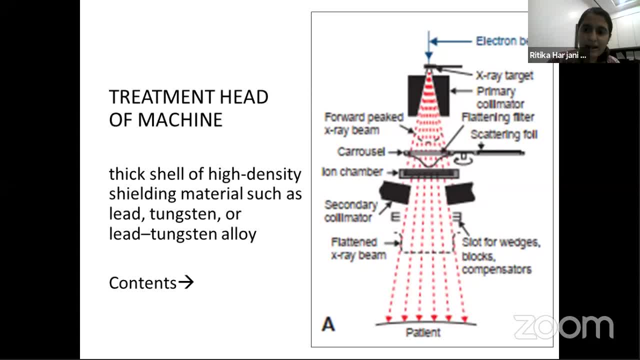 the machine. so it is basically the head of the machine that we see, or the gantry or the sea arm that we see is the head, which is made of a thick shell of high density shielding material like lead or an alloy, and it has many components. so, as you 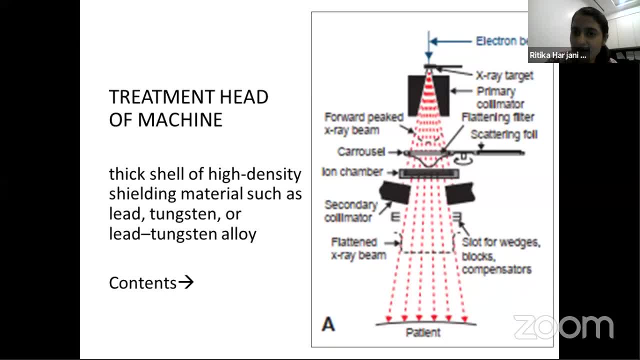 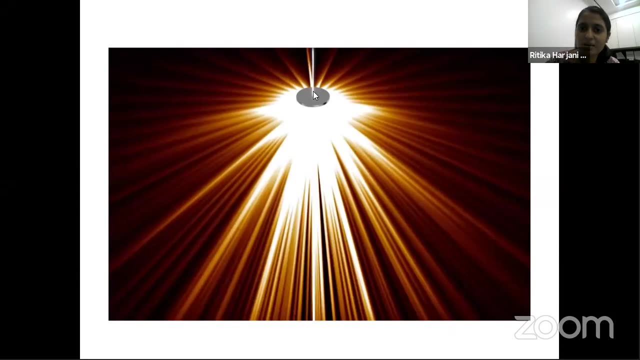 see in the diagram, electron beam has come and hit the target, and then there is a primary collimator, a flattening filter or a carousel with a scattering coil ion chamber, other collimators and wedges. so basically, now the beam, the pencil beam that we had, comes and 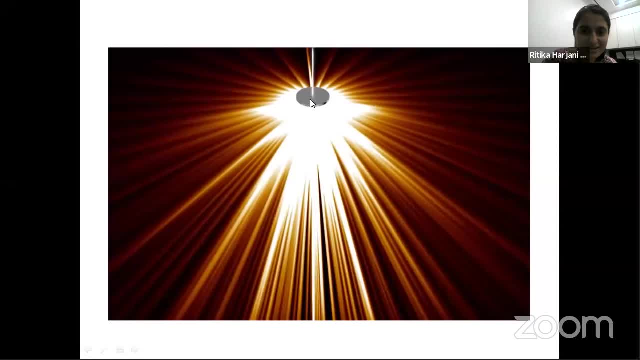 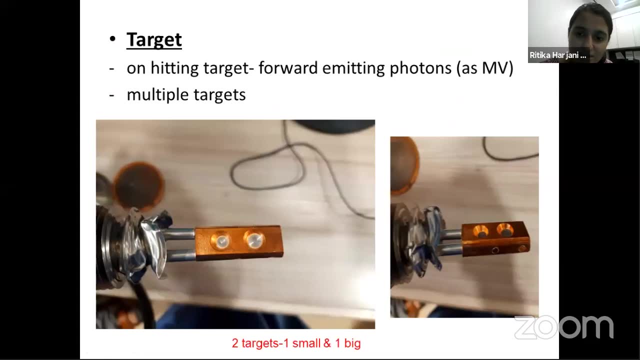 hits the target and then the x-rays are produced. just a very dramatic show of that. so, coming on to a realistic target, so this is a a target of one of our machines that we uninstalled. so these are two areas on the target. so, because many of our machines are, 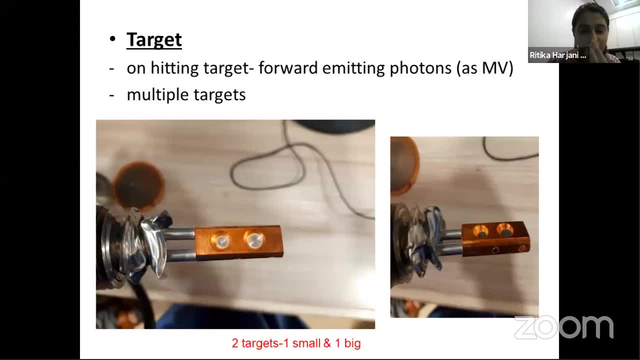 dual energy machines. so the target is different from for each energy, the energy that we choose, the target changes and we, as you remember, we have transmitting type of target, so the electron comes and hits from one end and the photons are released from the other end. so you would notice that. 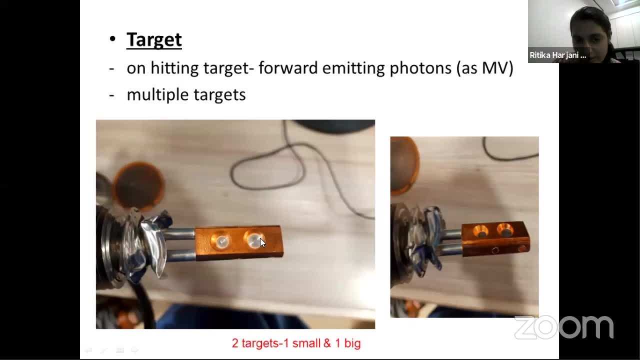 one target is smaller and one target is bigger. so initial thought would be 6 mv linac would have a smaller and 18 mv linac would have a bigger target- the x-ray beam. but it is actually opposite. the 6 mv linac has, as it depends, the 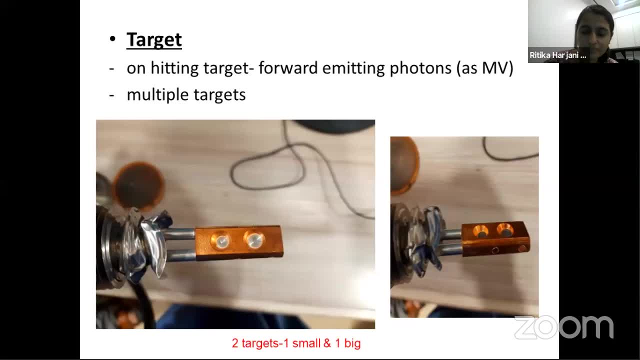 efficiency depends on the voltage also, so 6 mv linac will have a slightly lower efficiency than 18 mv linac, and that is why the heat produced in a 6 mv linac will be more than an 18 mv linac. so the targets are opposite. 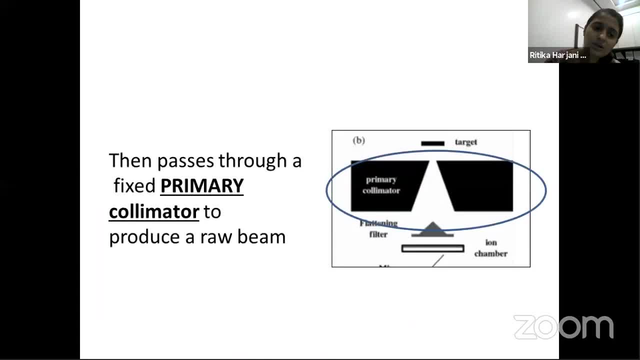 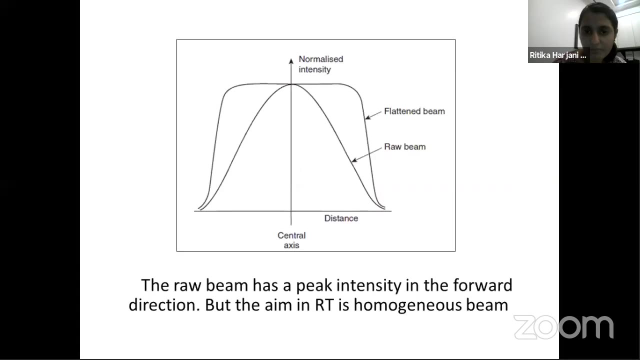 then, after passing through the target, as just a connotation- but the beam spreads in all directions, so we want something to collimate it- it passes through a primary collimator to produce our raw beam. now by raw beam i mean this: we had discussed that these photons that are emitted 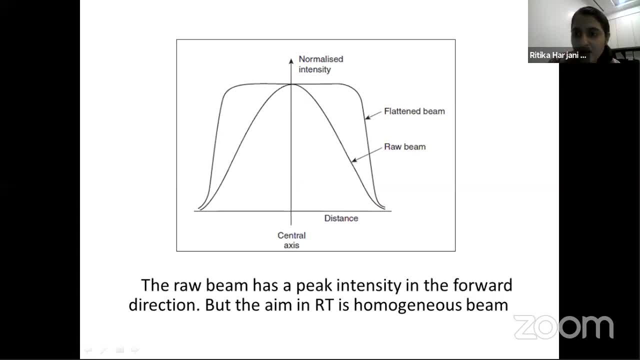 are actually forward projecting photons and they are forward direction because we are using in the mv range but not maybe in the most modern treatments. but historically we have always believed that we want a homogeneous dose distribution, so we want a homogeneous beam. so now this beam has to be made a flat. 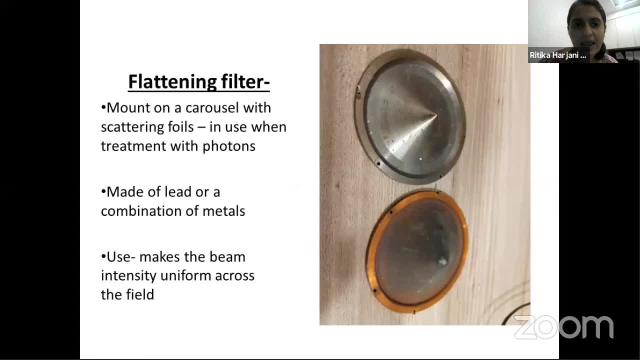 beam. we need a flat beam for our radiation therapy, and that is when flattening filters come up. they are basically mounted on a carousel, which can move- sorry, and with there is scattering foils and flattening filters on the same carousel. scattering foils are used when electrons. 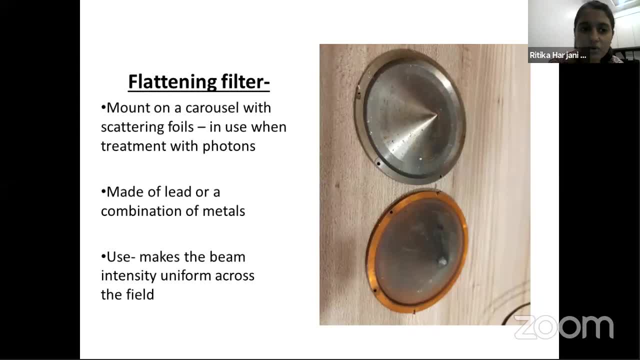 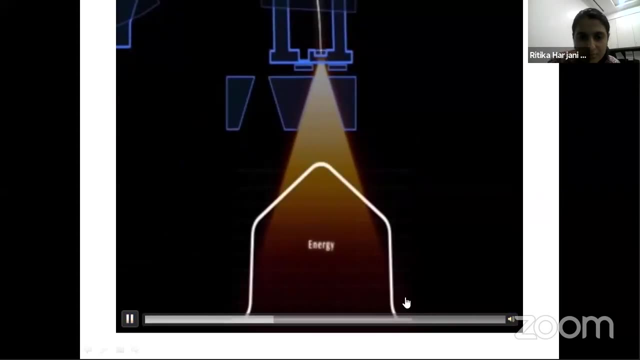 are in use, and flattening filter is used when photons are in use. it is made of lead or a combination and it basically reduces the beam intensity and makes it uniform. so another small video to show what it actually does. this cone shaped filter is placed in the path of the beam. 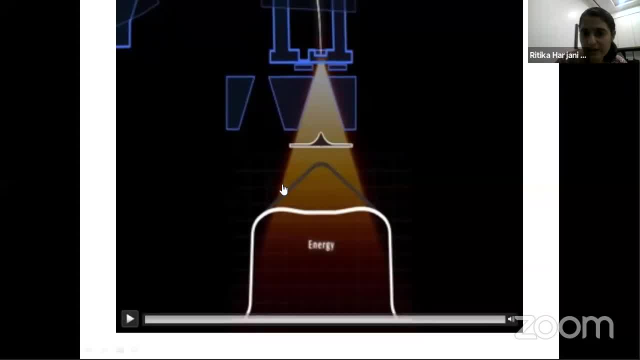 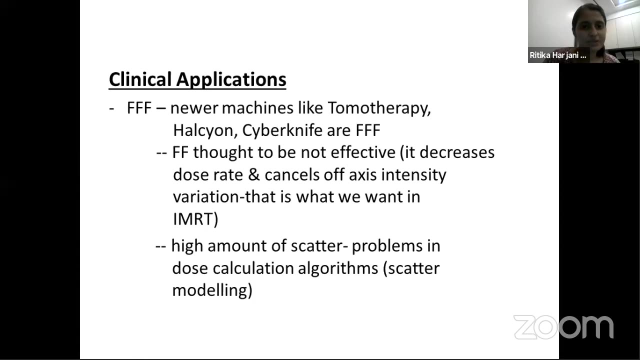 the cone shaped filter. this cone shaped, like you see this forward peaking beam is now made peak is now made flat by a flattening filter. so, but to actually tell the truth now, presently the hype is more about flattening filter free. so while we, while in the past, a filter was developed, 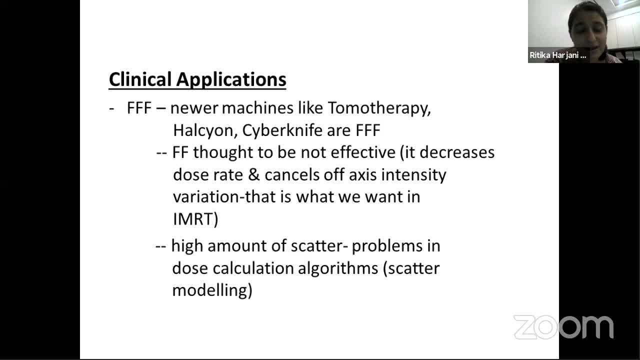 to flatten the beam. now maybe the thought is that why do we need a flat beam? actually we are just decreasing the dose rate and cancelling of an intensity variation and then in IMRT, VMAD, we actually try to achieve that intensity variation. so newer machines are now actually removing of that flattening. 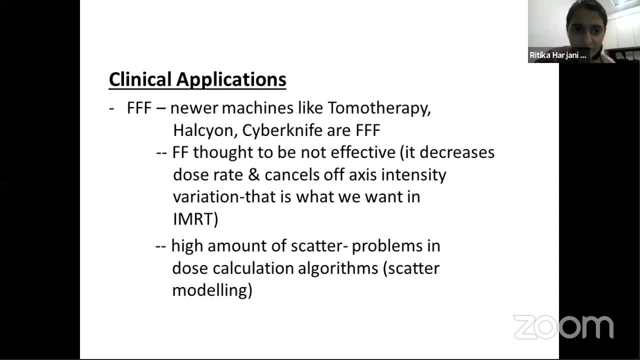 filter. tomo, halcyon, cyber knife are all flattening filter free. and the next problem with flattening filter is there is a lot of scatter because of the flattening filter and this scatter causes problems in there is problem in modelling that scatter in those calculation algorithms. 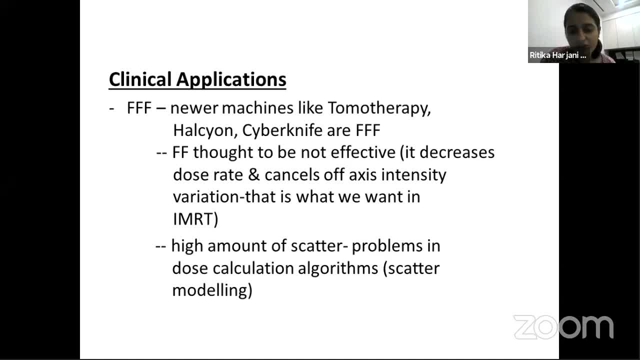 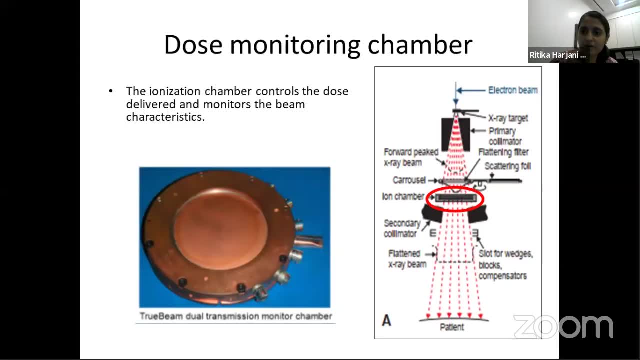 and that is why a lot of problems happen. so if the flattening filter is out, even those calculation algorithms are slightly simplified. next, after this diagram here overall, after striking the target primary filter in a flattening filter, there is something called as the ion chamber which is there in the path. 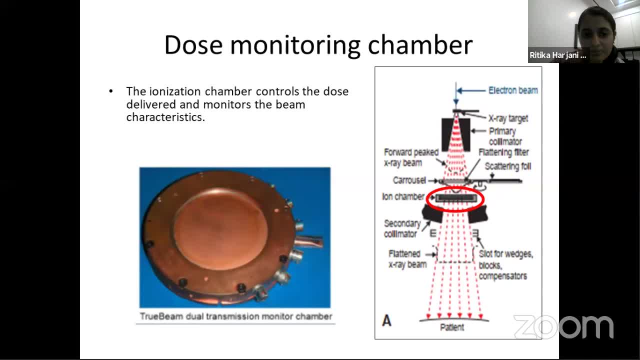 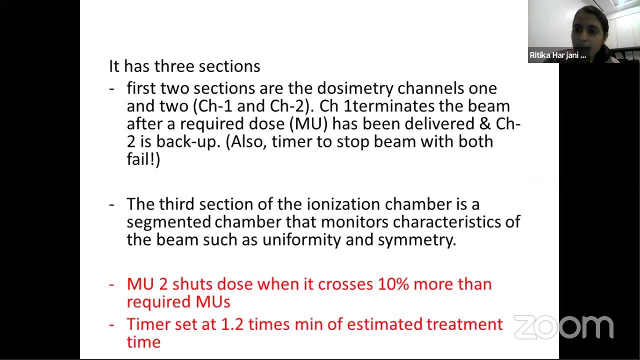 of the photon beam or the x-ray beam, this ion chamber. this is again a photograph of a variant ion chamber. the ion chamber basically controls the dose that we are trying to deliver and it monitors the beam characteristics. so it has three sections. one section is the first, primary. 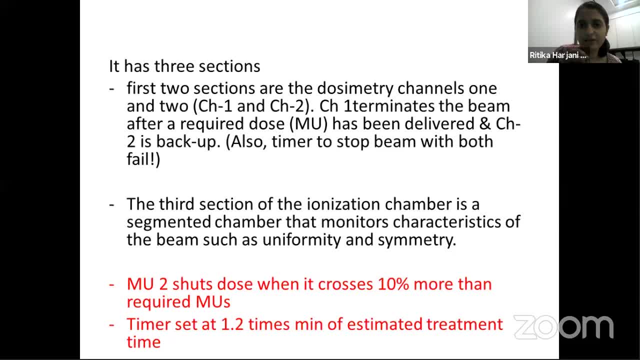 ionization chamber is the main one which tries to terminate. if we have said that we want to deliver 600 MUs, it will terminate the beam after 600 MUs have been delivered and a channel 2 is there which is just a backup. so channel 2 generally. 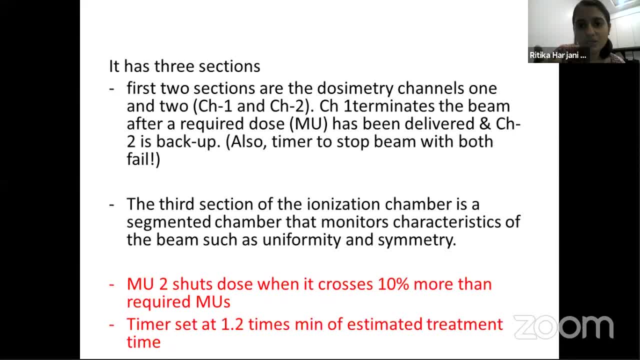 if the channel 1 fails and by how much it fails. so if it crosses 10% more than the intended MUs and channel 1 is still allowing it to pass, it has not stopped the beam. the channel 2 controls and switches off the beam and 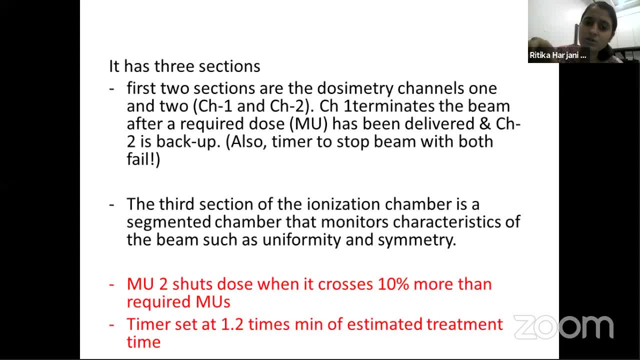 so if these two both fail, a timer is also there in the LINAC machine which is set at a particular value. so suppose, if my treatment is to last for 1.1 minute, so then the timer is generally automatically defaults at as 1.2 times. so 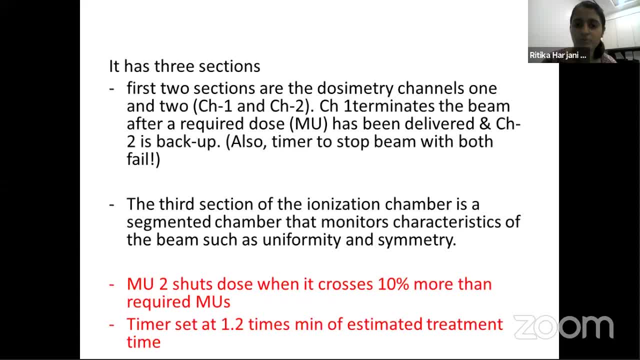 that if both the ionization chambers have failed to stop the beam, then the timer will at least stop the field. so this is just a double multi safe mechanism so that the patient is not at risk. the third part of the ionization chamber. there are three parts. 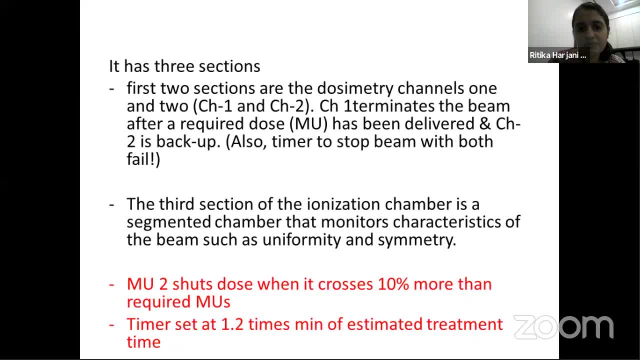 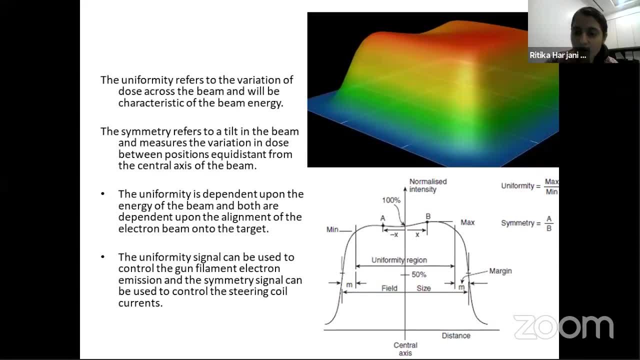 I mentioned. the third part is basically to check if the beam is uniform or not, it is symmetric or not. so these are important points when a beam is coming out, and all this is very reflexly controlled. if the beam is not uniform, then signals go and it is controlled, so there is a 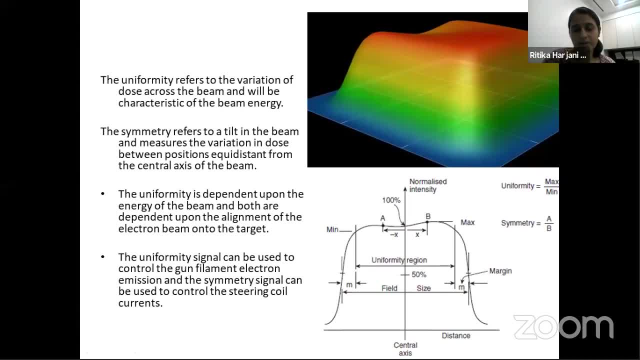 very efficient feedback loop present in all our LINAC. so this is basically a 3D view of a beam that would go inside and, if you notice, although it is more or less flat, but there is some amount of irregularity in the beam surface and just in a 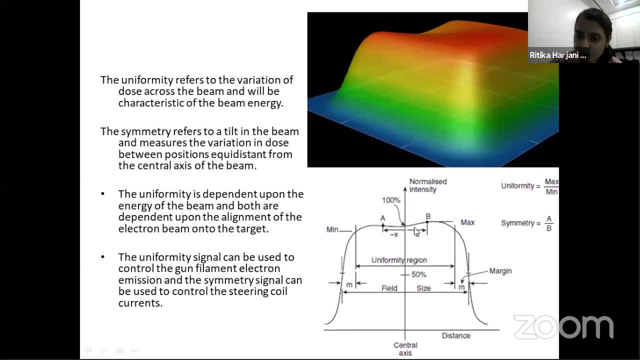 2D view, so the beam may not be very flat. and then there are these two points which we evaluate on that basis is symmetry and uniformity of the beam. so symmetry would be the beam symmetry at two points equivalent from the central axis, and uniformity would be 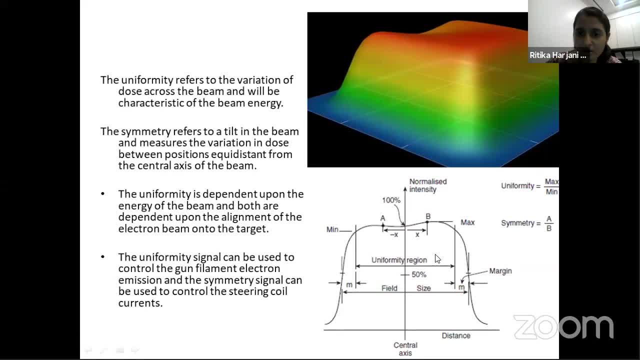 the variation of the dose of the beam at, overall, the maximum versus the minimum. so these uniformity and symmetry are dependent on the energy of the beam and the alignment of those steering coils and how it struck the target. so all that, so once the uniformity is, 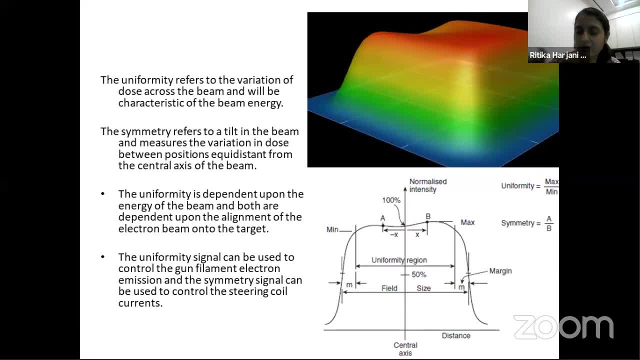 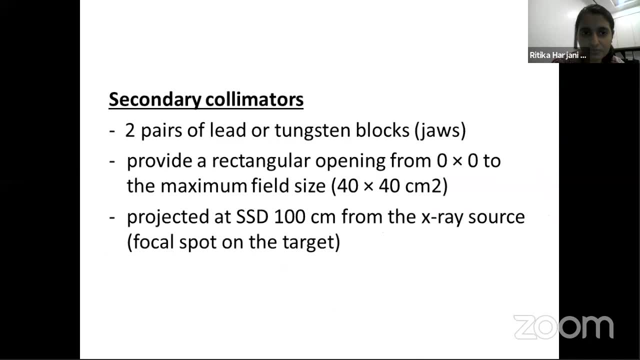 and the symmetry is disturbed. there are control reflexes that go on to the steering coil, focusing coil and even the electron gun. then, after passing through the ion chamber, it goes on to secondary collimators, which are generally lead or tungsten blocks, which provide a rectangular opening of maximum of 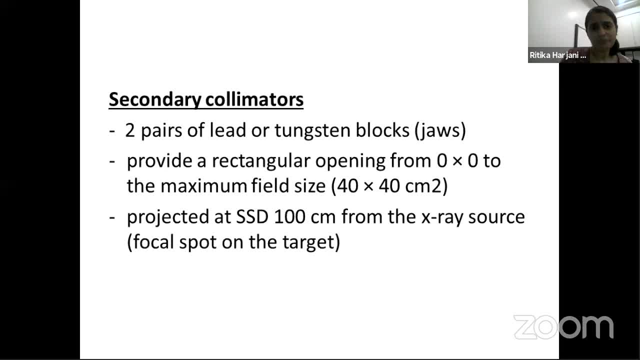 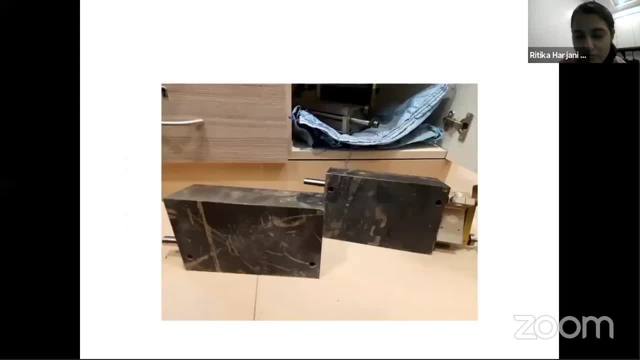 14 to 40 cm, but again, that is not something that we now are satisfied with, so sorry. before going that, these are the photos of secondary collimators from one of our old machines, and these are the jaws, basically, which would come from each direction. and now we are. 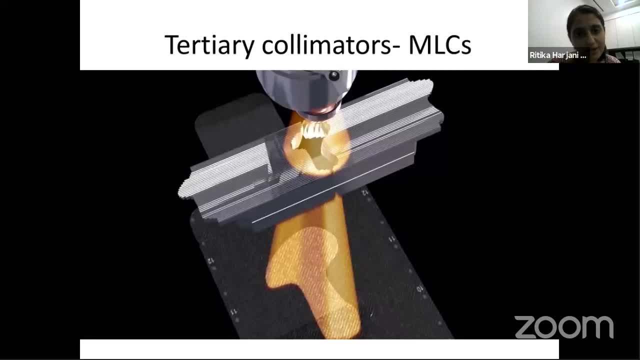 not satisfied with secondary collimators. we need more individualized beams for individualized fields, so MLCs are the ones that are used for most of our treatments. I would think that MLC would be in detail covered by the person covering IMRT and IGRT. 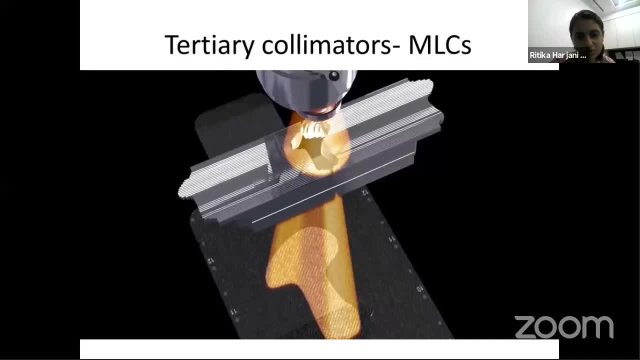 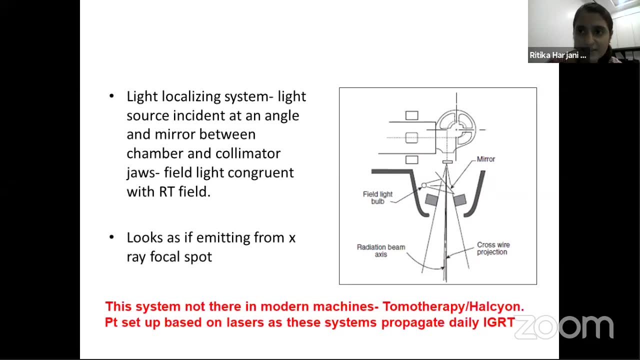 so I have not gone into details of MLCs today. so the another component of the LINAC would be a light localizing system. now, all that is we have seen the path of the electron and it becoming a photon, becoming flat. but we do see something on the 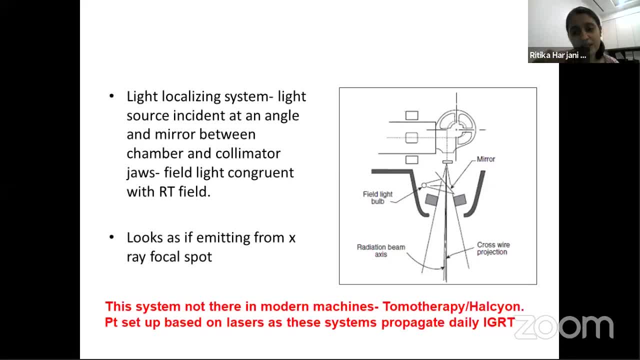 patient's skin, we see the field or we see the MLC openings. so that is basically because a mirror is placed in the path of the photon beam after it strikes the target. here, if you remember, I was mentioning about 270 degrees, having more number of magnets for 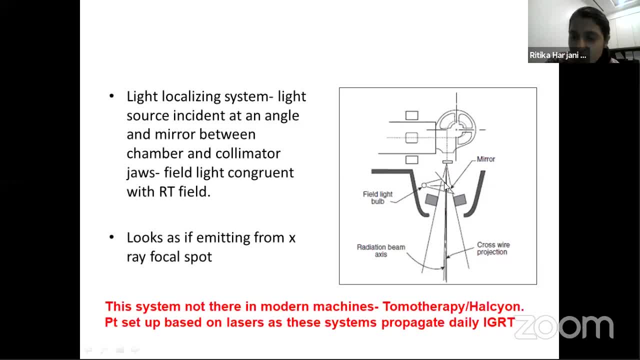 a better bending. so this picture clearly shows just to move forward the mirror here and there is a light source on the side. so this light falls on the mirror and it falls on the patient's surface through which we can see the field light. and that field light it just 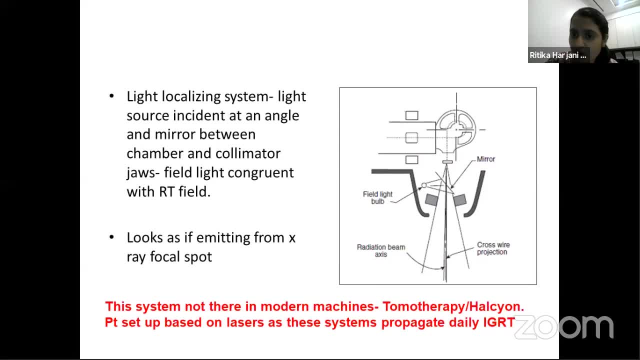 appears that it is coming from the target focal spot, but it actually comes from a field light bulb. again, we were very used to seeing fields in the past, but that is not something today. so again, this field light localizing system has been taken away from a tomotherapy. 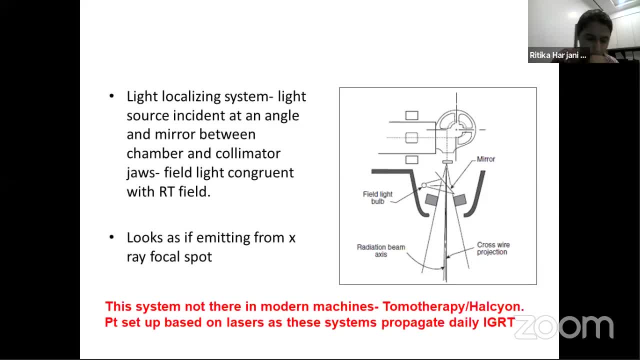 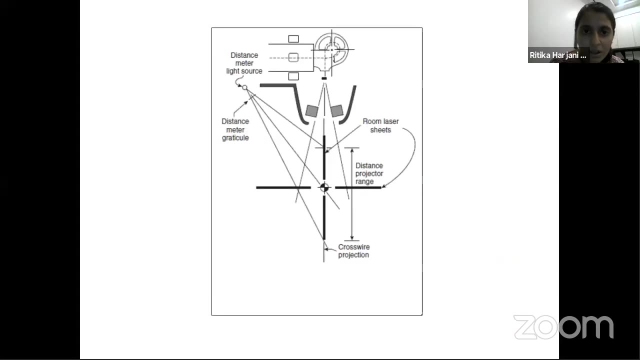 halcyon machine patient is based on lasers and they don't want us to see the field actually how it looks on the patient. they want the norm is IGRT, so image verification and treating. so that is now becoming going away with the newer machines. there is one more thing: the optical distance. 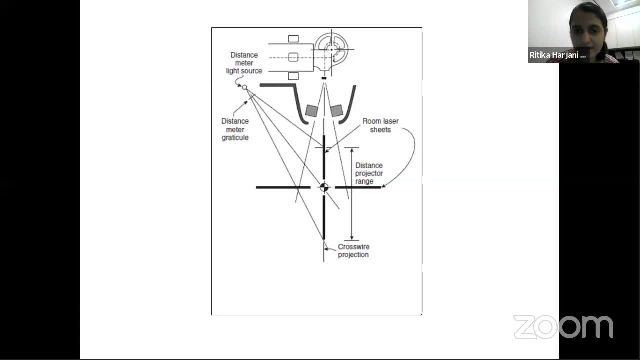 indicator. we check the SSD of the patient on the skin, at least all those we still do 3D CRT. so on the 3D CRT. so there is a distance meter, gratitude and light so separate, for that in the gantry which throws a projection on the skin. 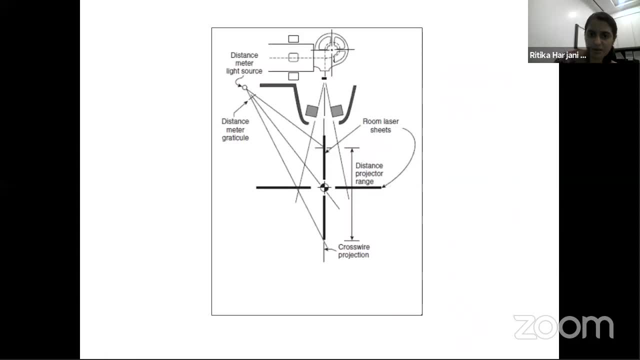 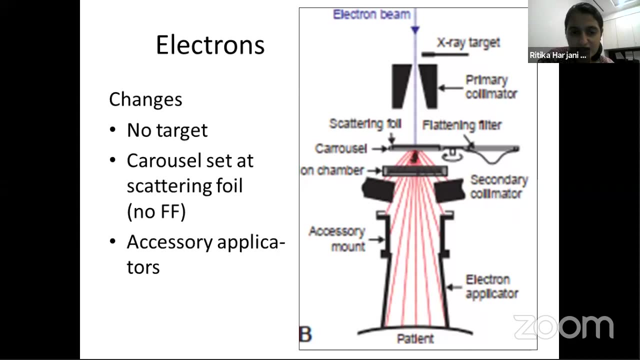 this was about a photon beam again in this. apart from these, there are also some slots for wedges and apart from the MLC there are even slots for wedges to modulate the beam externally coming to the electron beam. there are. in the basic flow of events there are few changes. 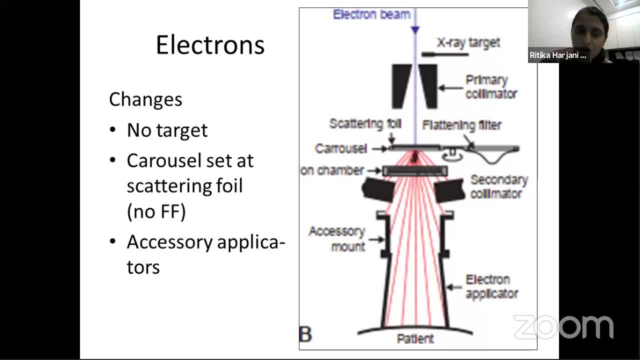 the major changes. there is no target, so electrons that are accelerated in the accelerating wave type come in directly, enter into the after having bended by the bending magnets are used for treatment directly at the carousel level. we do not use a flattening filter that is removed out and we use 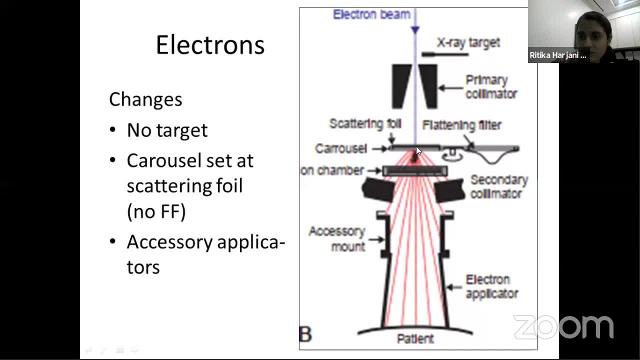 something called as a scattering foil. we want electrons in a wider area. we do not want that 3mm pencil beam, so that 3mm pencil beam is made to scatter into the required area that we want. and then we have accessory applicators- electrons we do not treat. 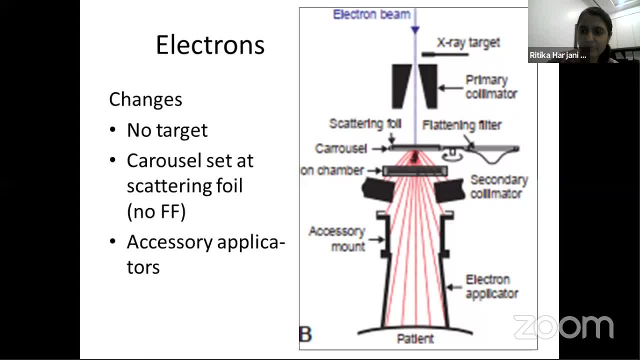 with the regular from the gantry at keeping certain amount of distance. we generally want the applicators to be as close as possible to the patient, so that is because I will come to that, but before that, the scattering foils that I had mentioned. so scattering foil, basically, as 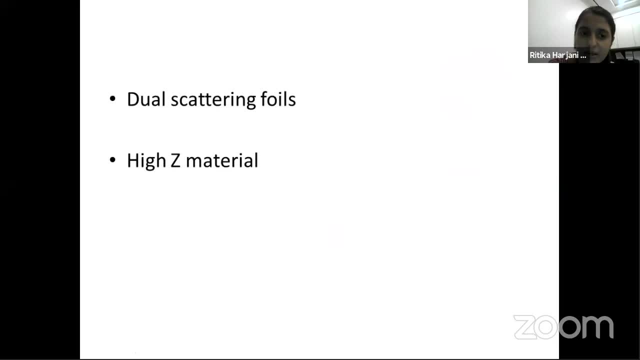 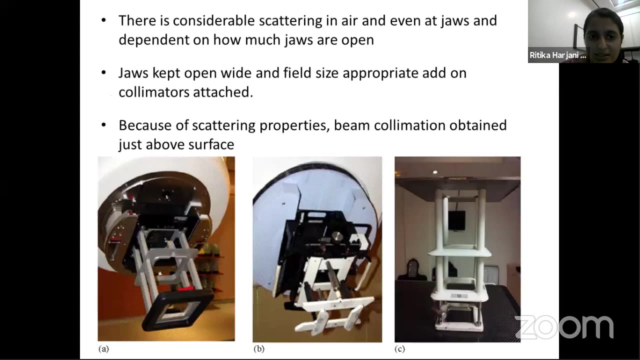 we remember from our electron basics that it requires electrons are absorbed by low z materials and scattered by high z materials. so a high z material is generally used and dual scattering foils are used to scatter these electrons and then these electrons which have a basic tendency to scatter. 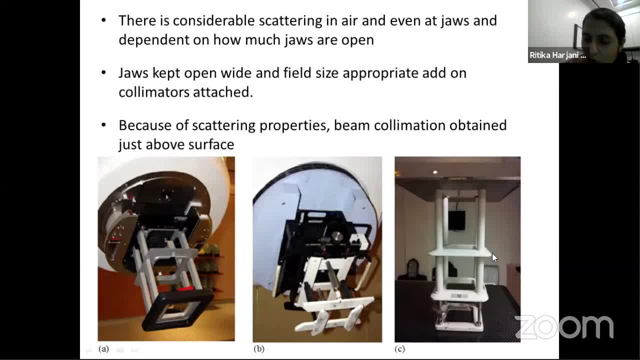 in air also and even at the jaw openings. so what is done is the jaws are kept wide open and then to direct those electron beam into an appropriate field size, external applicators are used which nearly come to the patient's skin or are about 5cm away, just for clearance. 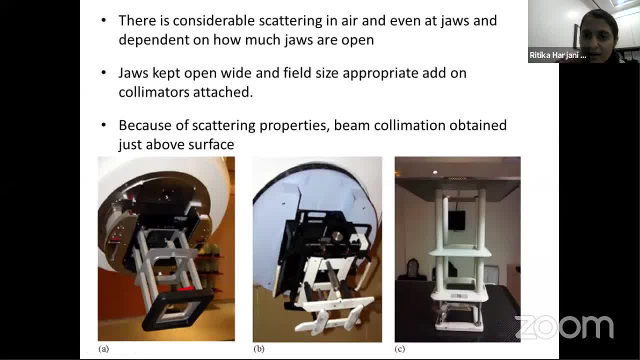 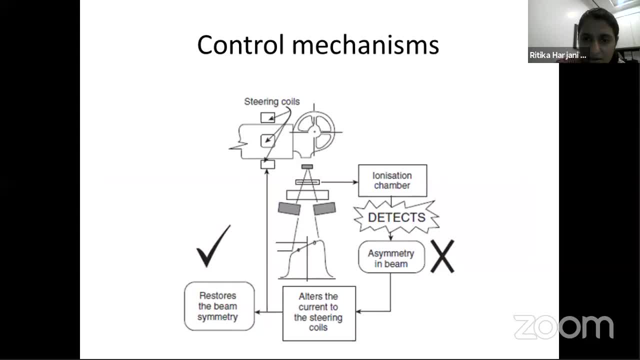 purposes. so because of these scattering properties, the beam collimation is obtained just above the surface. as I mentioned this already, these all things are very tightly regulated by control mechanisms and feedback loops. like telemetry goes to steering coils and it is corrected immediately. another thing: components of our linac. 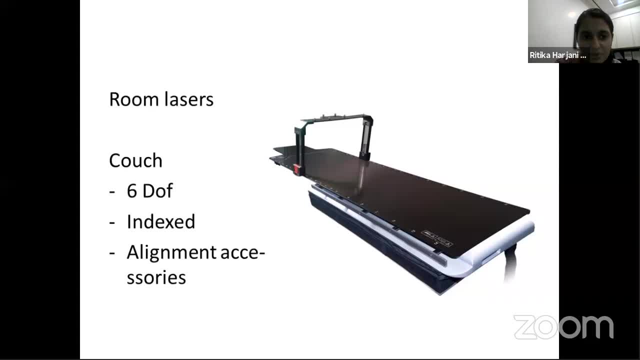 is, of course, our room, lasers which we set up the patient. and then there is a couch which presently most of our centers have, a couch with 6 degrees of freedom: movement for movement, the three translational movements of x, y and z axis and the three raw. 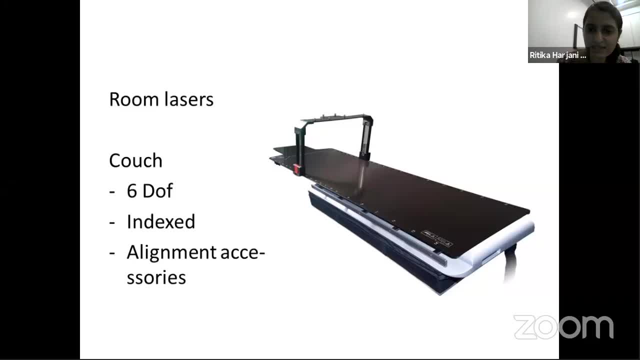 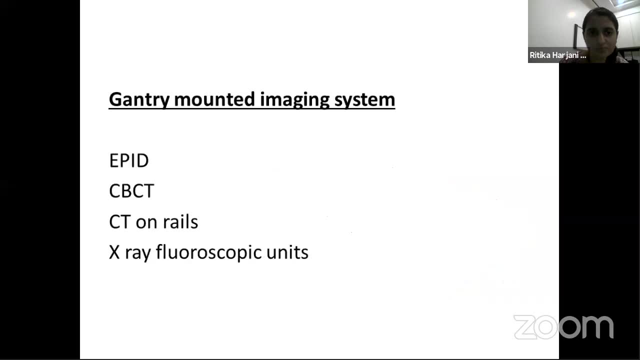 roll, pitch and yaw for the rotational movements. they are generally indexed and they have accessories that can be aligned to it and attached to it. again, apart from the arm with the linac head, we also have a perpendicular to it, generally a C arm for imaging. again, imaging is something that 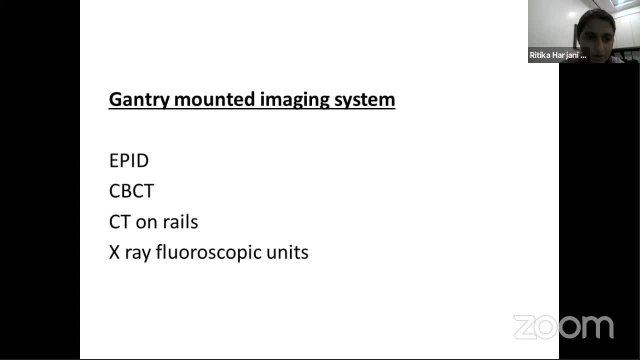 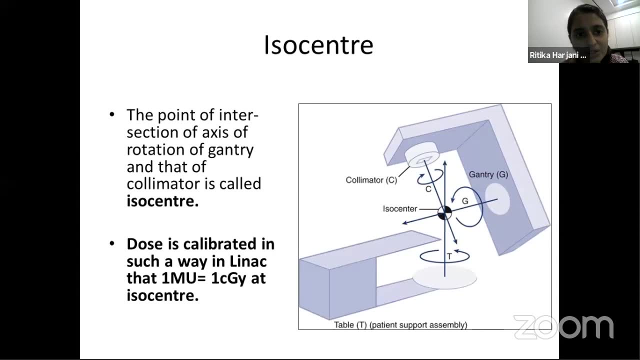 would be dealt in detail with IGRT class that I have not covered. so all these machines are our traditional linac is basically an isocentric machine. so the point of what is an isocenter, the point of intersection of axis, of the rotation of the gantry, 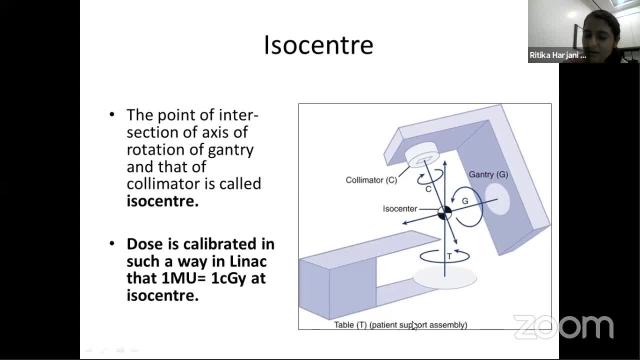 the, the gantry, the collimator and the couch. they all, when you join a line of the axis of rotation, they meet at the point and that is called as the isocenter of the machine. and when we, when dosimetry is done by our physicists, the machine is. 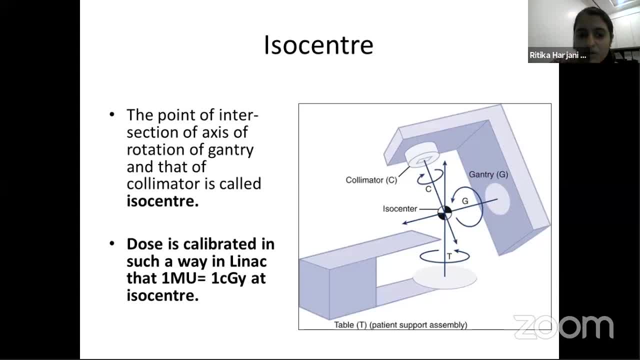 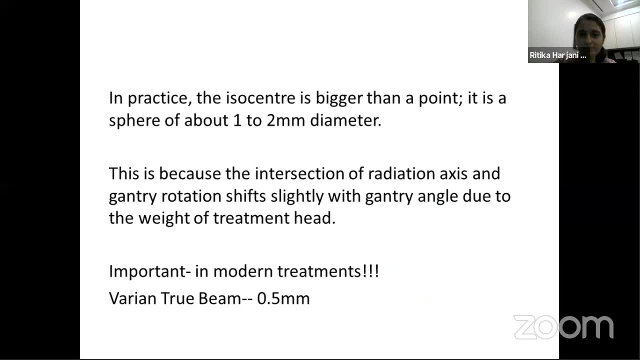 calibrated in such a way that one mu is equal to one centigrade at the isocenter. although we say that they all meet in a point, in practice the isocenter is not one point. it is about the sphere of one to two millimeters. 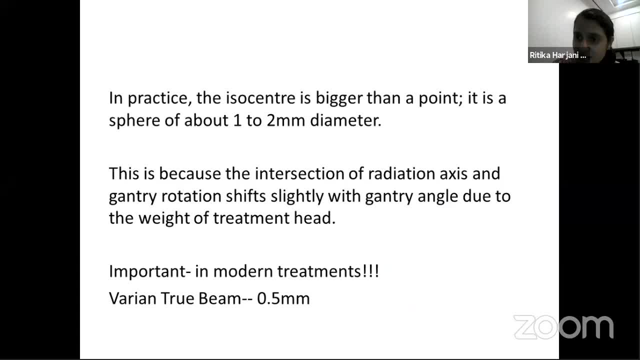 that is because the intersection of the axis of gantry- the gantry is really very heavy, so it causes some amount of violet rotates. there is some amount of the axis does not exactly meet through the point and so it is about one to two millimeter now. our 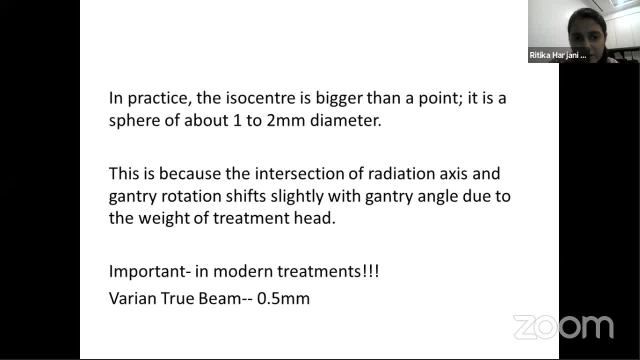 newer machines, that is, that may not be important when we are treating our 15 by 15 fields, but in techniques wherein we are using a linac for srs treatment or sbrt, an isocenter, being very point specific is very important. so now 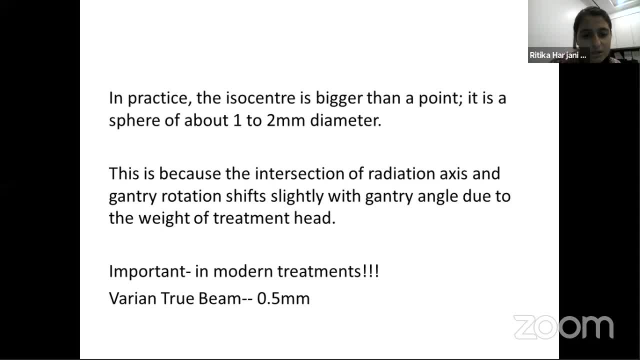 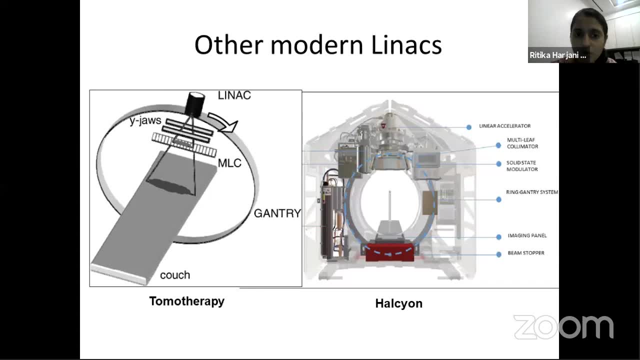 like the newer machines promise an isocenter with a sphere diameter, so variant crew beam has a 0.5 mm diameter. then we have evolved to newer linacs. just a brief about it: from the c arm based linacs we have moved on to ring based. 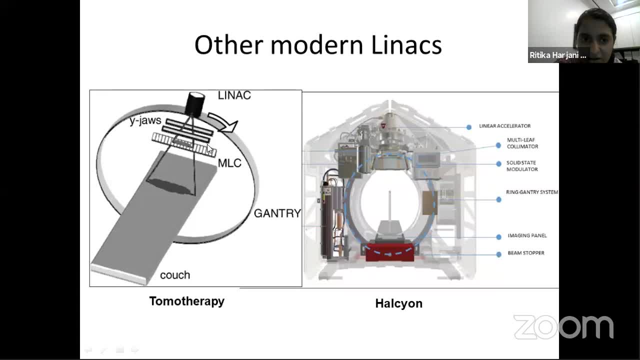 linacs, wherein we have gone away with our flattening filters and the light systems. we have some jaws and mlc's in the tomotherapy and similarly many of our institutes in india are now taking up the halcyon by variant. so that is also a similar design. 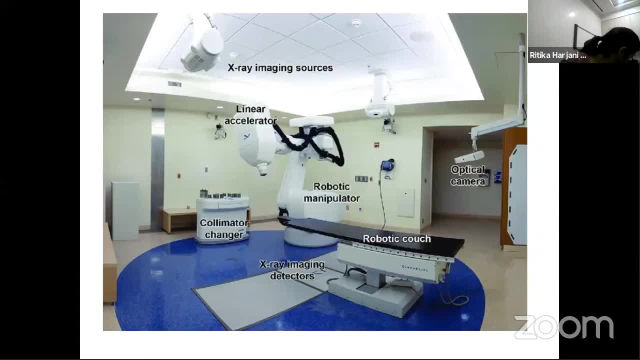 of a ring based gantry. and then, to top up, we have our srs robots like the cyberknife, wherein we still have the same components, and a 6mv linac, but it is a miniature linac with a robot and very specific and sophisticated imaging system for 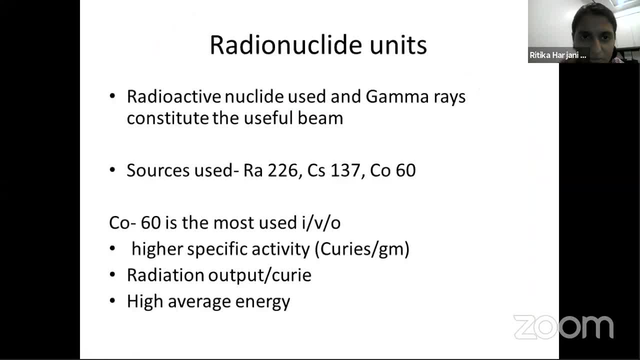 appropriate sbrt treatments. coming to the next part of it, the radionuclide units. radionuclide units, basically, are gamma rays, are what constitute the useful beam, and there are many radionuclide units, radionuclides that have been used in treatment. 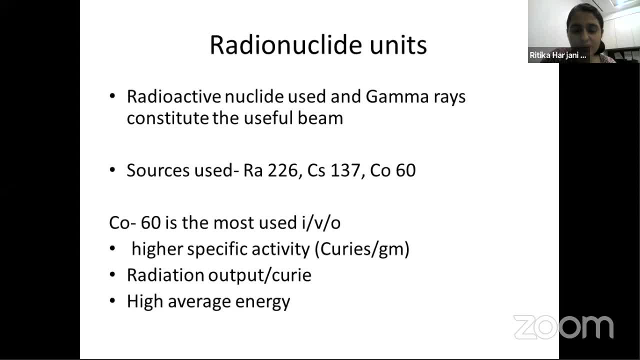 like radium or cesium cobalt, but mainly teletherapy beams. cobalt is the one most commonly used because we want a higher specific activity. specific activity was again dealt in detail by dr jiva, but basically it is the amount of curies or the activity per unit gram. 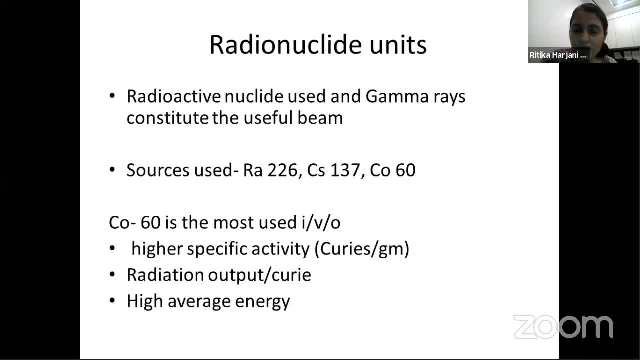 so the higher the specific activity. like cobalt has a specific activity of 200, versus cesium has 50 and radium has something less than 1. so based on that, cobalt is a preferred material. we need a good radiation output per curie and a. 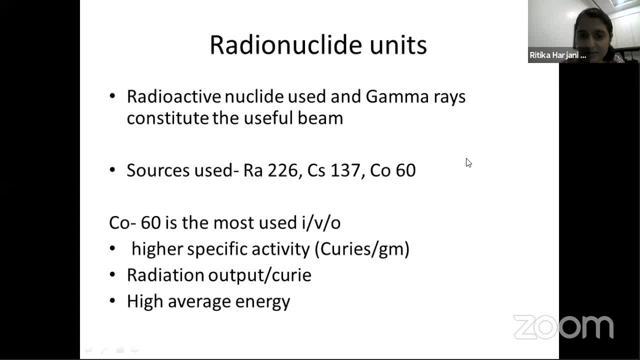 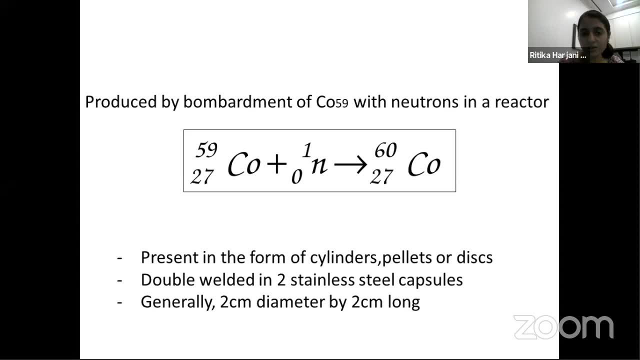 higher average energy. again, amongst the three, cobalt has the highest energy. so how is cobalt 60? cobalt in its stable form has a cobalt 59 is the number and when it is, how it is produced is in cobalt 59 are made to. 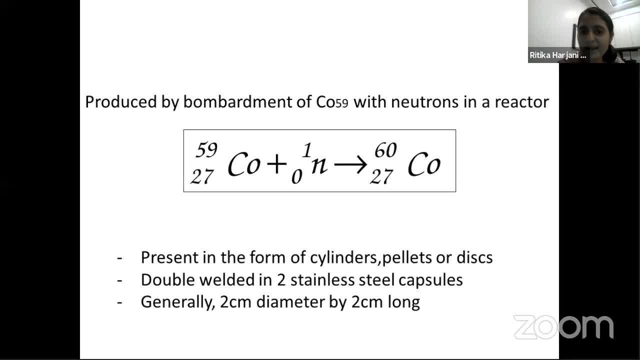 interact with neutrons in a reactor, there is bombardment and that leads to production of a cobalt 60 beam. these cobalt 60 is present in the form of cylinder or pellets or disc and double welded, basically in two stainless steel capsules to prevent leakage. generally, the cobalt 60 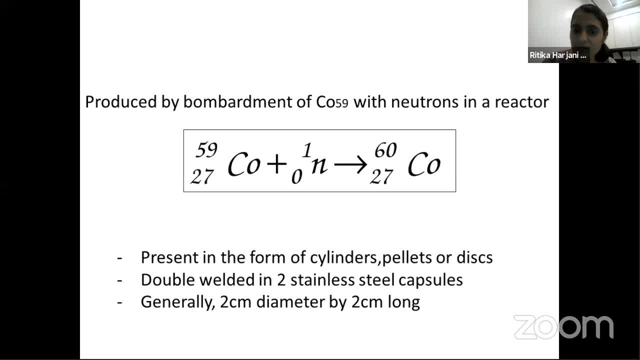 source in our therapy machines is 2 x 2 cm, and this actually is a drawback because, as against the focal spot- where is which is, we are dealing in millimeters- this 2 x 2 cm creates something called as penumbra, which we will come to in a while. 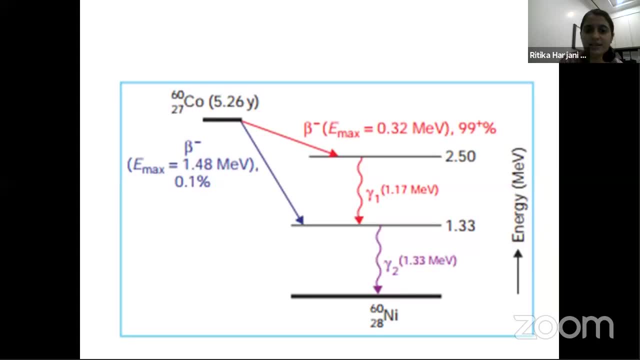 so this cobalt 60 now gives off part of its energy through beta emission, and then gamma rays are emitted with the energy of 1.33 and 1.17 and an average energy of 1.25 generally, and then it gets stable into nickel 60. 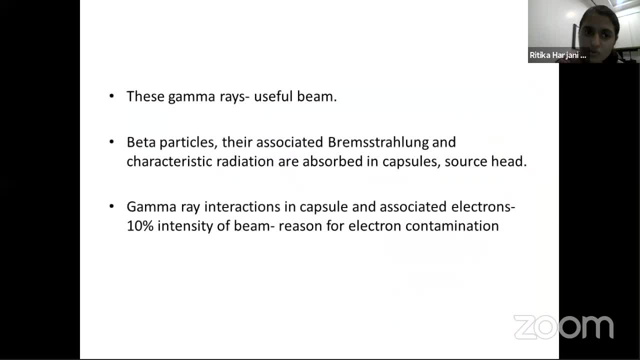 these gamma rays form the useful beam and there are some amount of beta particles that I mentioned. they and their associated characteristic radiation are generally absorbed in the stainless steel capsule or the source head. the gamma ray interactions in the capsule and their associated electrons do contribute to some amount. 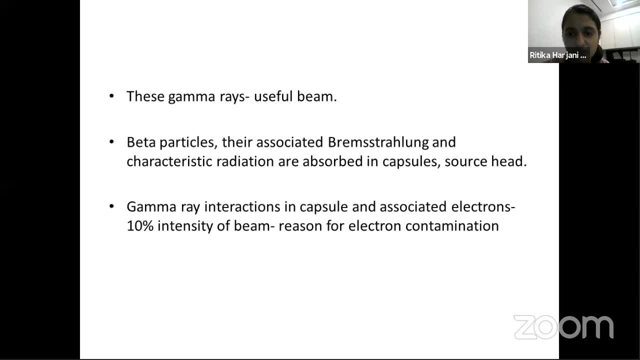 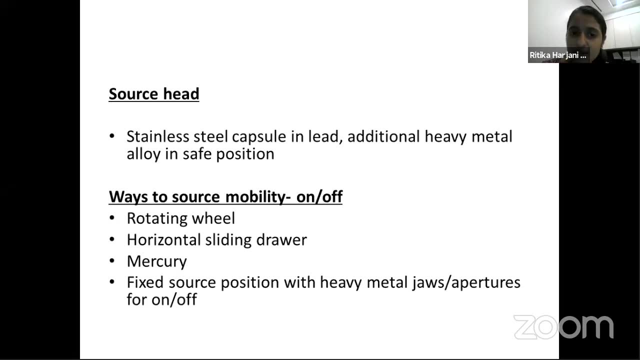 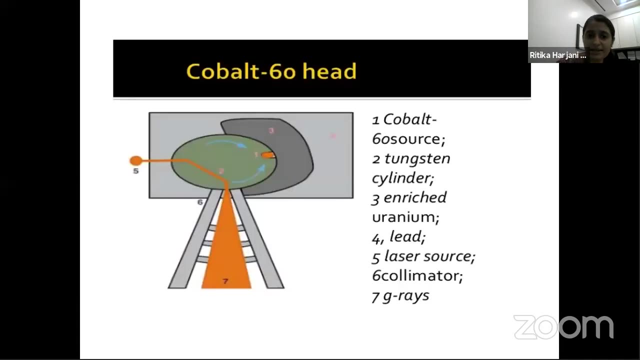 in the beam and that is a reason for the electron contamination. the source head- now we have a cobalt source inside, so it is a very heavy source head with lead and additional heavy metal alloys and there are source- is generally kept in an off position, wherein it is not in the direction. 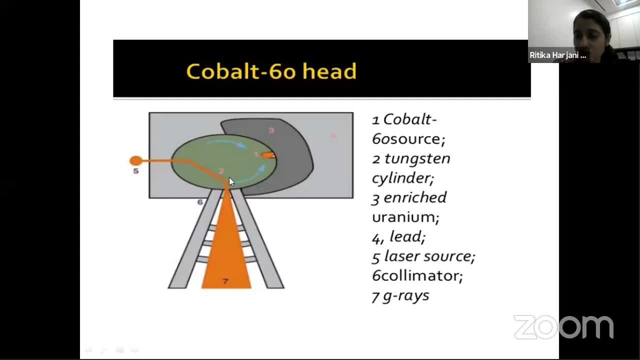 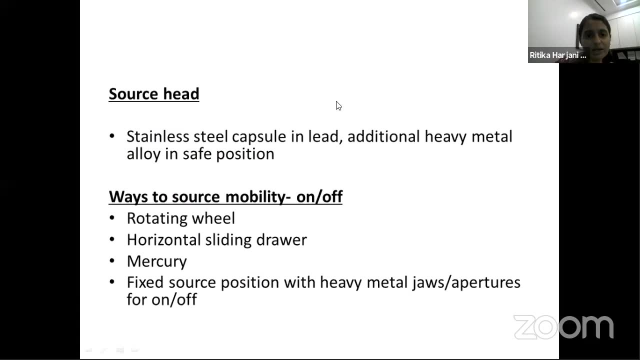 of the beam and it is made to come in the on position when required, when we switch on the beam. so there are ways to bring it to the on position. there is generally a rotating wheel, which is this in the picture, this in the off position it comes to. 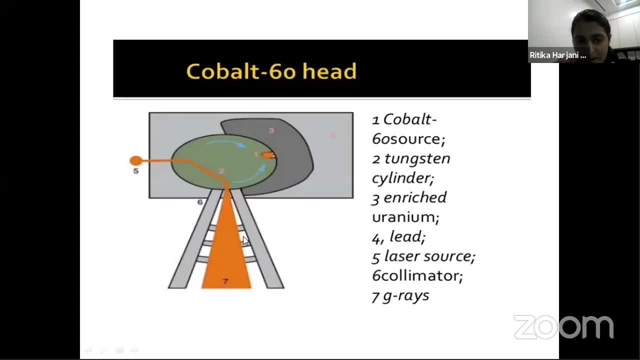 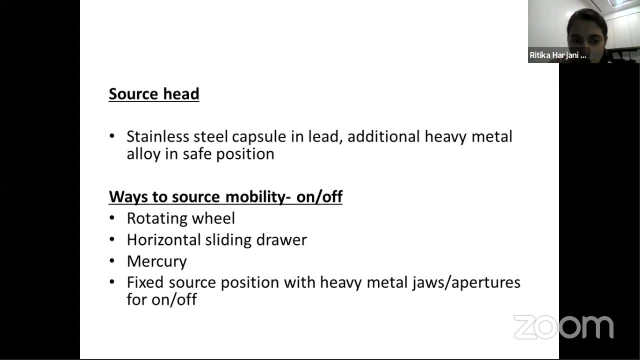 the center and then delivers the gamma rays are emitted out. or there is a drawer sort of a mechanism. you open the drawer and the source comes into the on position. no one mechanically opens it. the mechanism is such: there is mercury based with with the help of pneumatic pressure. 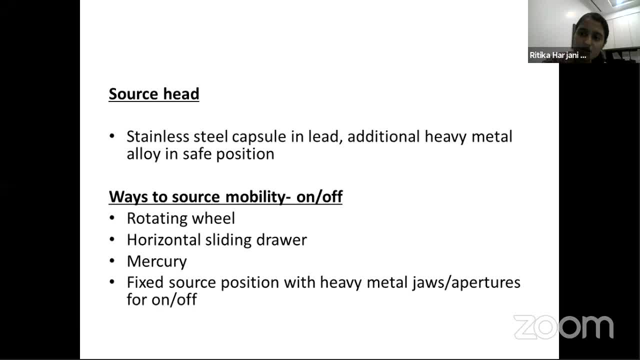 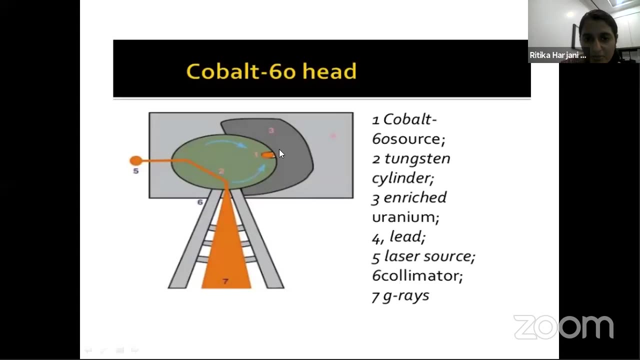 and then sometimes really, the source is kept in one position itself and there are heavy metal jaws which close and open to make the beam on or off. so this is just a rotating wheel diagram wherein source is in the off position and while it is in the off position there is a very 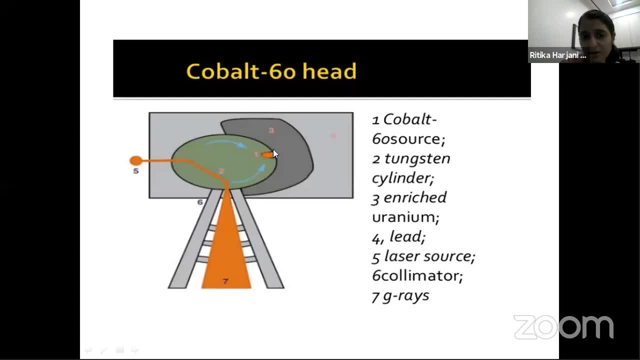 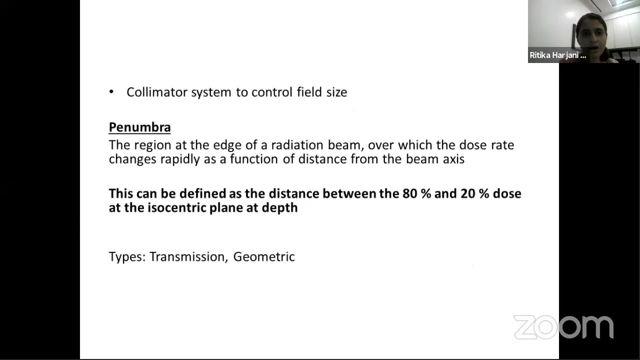 heavy material like enriched uranium, to protect the exposure anywhere and when it is rotated, it comes to position 2 and the beam is called collimated through the collimators and gamma rays are used for treatment. a collimator system is used to control the field size and 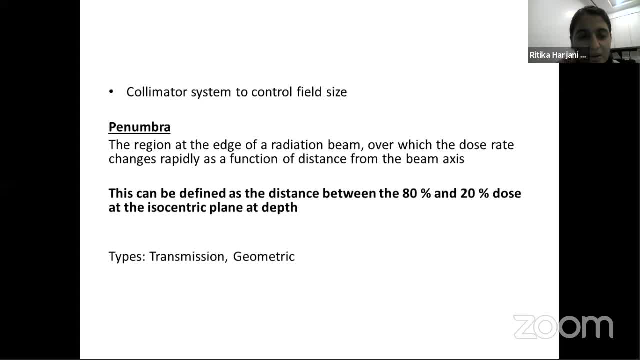 now, as I mentioned, because of the size, there is something called as penumbra. so penumbra is basically when we see the field. this is the region at the edge of the radiation beam, over which the dose rate changes rapidly as a function of distance from the 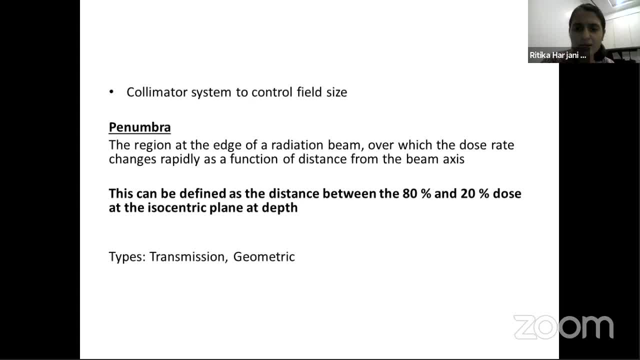 center of the beam axis. so generally it is not a hard and fast thing to say 80 and 20 isodose line, generally, any two fixed isodose line, but for practical purposes commonly or exam point of view, it is asked as may be mentioned as a distance. 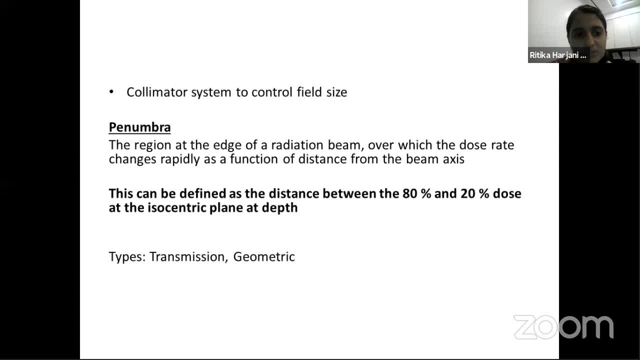 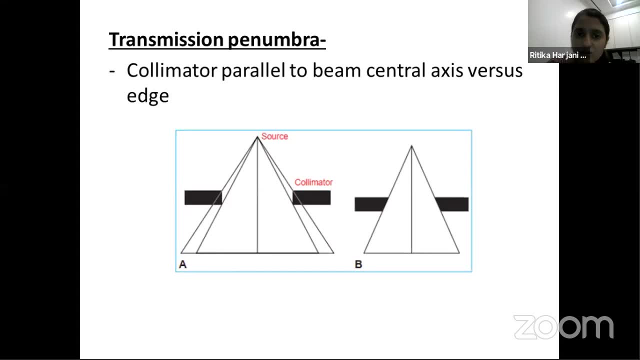 defined as a distance between 80% and 20% isodose lines. there are different types of penumbra. I will come to it. one is the collimation, collimator, associated penumbra called as the transmission penumbra. so basically, collimators can. 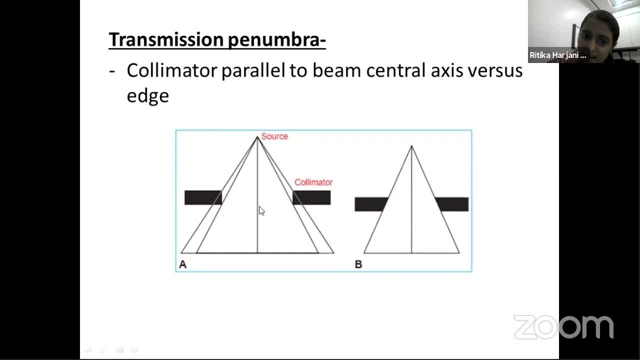 have an edge which is parallel to the central axis of the beam or can have an edge which is parallel to the, the beam, the divergent beam part. so if it is, if it is having a angle or the edge which is straight or parallel to the central axis, then 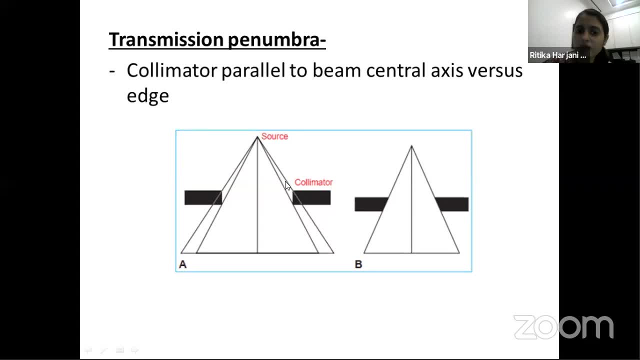 periphery of the beam passes through the collimator, so of course the intensity of the beam is decreased, so that contributes to the penumbra which is called as transmission penumbra. transmission penumbra is not zero when we have a collimator which is parallel to. 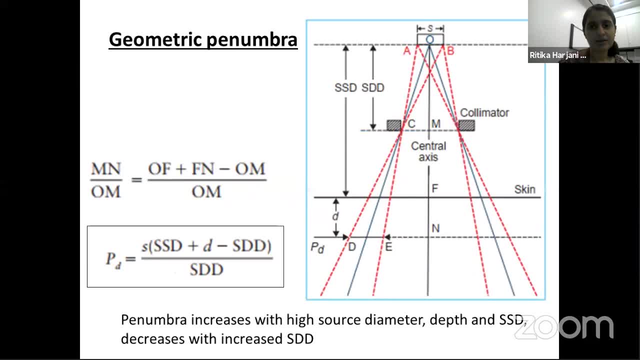 the divergent beam, but it is reduced significantly then the another important thing, and sometimes commonly asked in exams also is, or we try to study- is geometric penumbra. so geometric penumbra is basically what depends on a lot of physical points like the source size. that is why I had mentioned 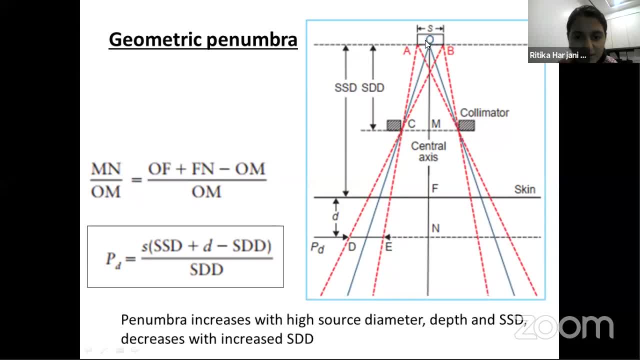 two centimeters is not the ideal but the best that we can achieve- and the source to surface distance, the source to diaphragm distance. so just to explain this diagram, if we consider this, of course, this is the cobalt source. here at the top S, these are the collimators. 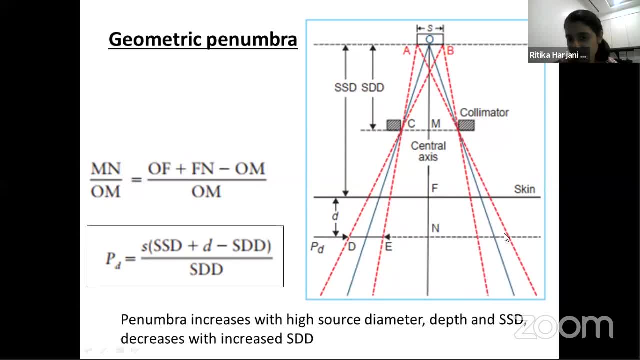 and skin surface and the depth at which we are measuring penumbra. so if we- and these are the diverging x-ray beams- from B it will go to each point, and from A also and from the center also. so if we consider this, CAB and CDE as equivalent triangles, 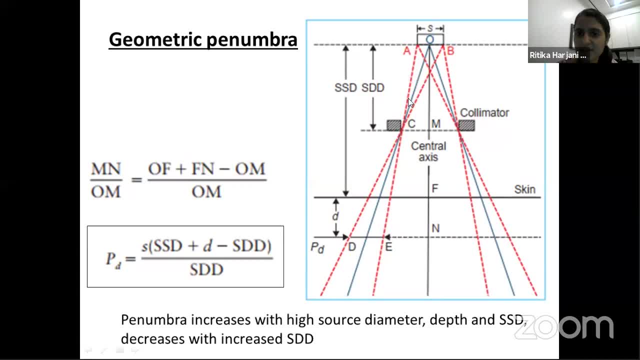 each of its size ratio will be equal. so CA upon CE will be equal to CB upon CDE, will be equal to AB upon DE. so this, and then, similarly, extrapolating your OM, it will be equal to OM upon MN. so that way, the MN upon OM. 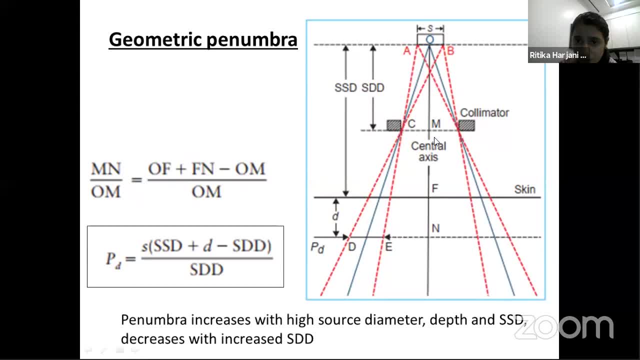 will be equal to when we consider it on this side, the equation comes up to when you try to write it out. it comes up to OF upon FN. so basically, OM, OM upon MN will be equal to the entire thing OF upon FN minus OM. it is just. 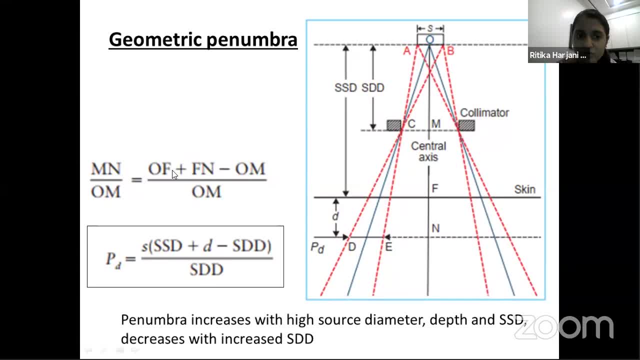 subtraction of these numbers here. and then, if you O, F is the SSD and FN is the depth at which we are measuring and SDD is the source to diaphragm distance, which is OM upon the source to diaphragm distance. so the penumbra. 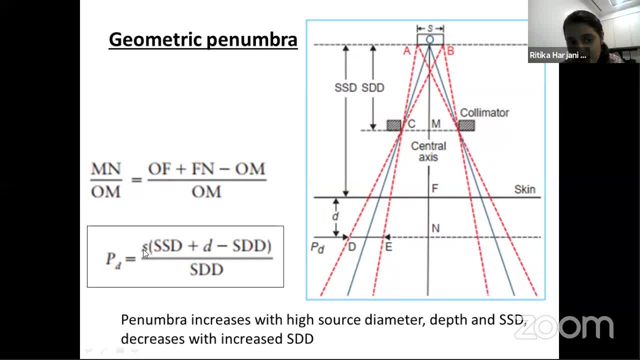 at a depth depends on the source diameter which goes up here, the SSD and the depth at which we are seeing and the source to diaphragm distance. while it increases with increase in source size- and that is why 2 cm is not good- it increases with increasing SSD and depth. 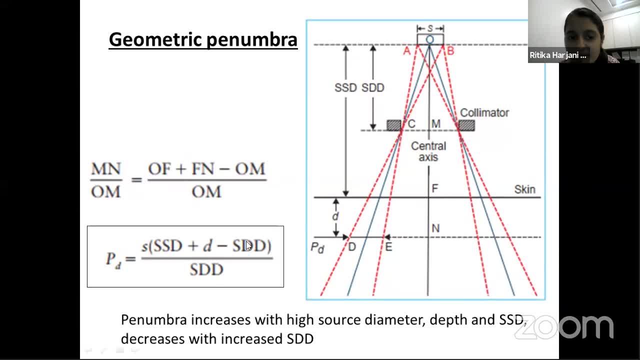 it decreases with we want to decrease it, so it decreases with increasing. source to diaphragm distance. this is the source to the collimator, or the diaphragm distance. so now this penumbra, we could be decreasing it by increasing this, bringing this collimator close to skin. 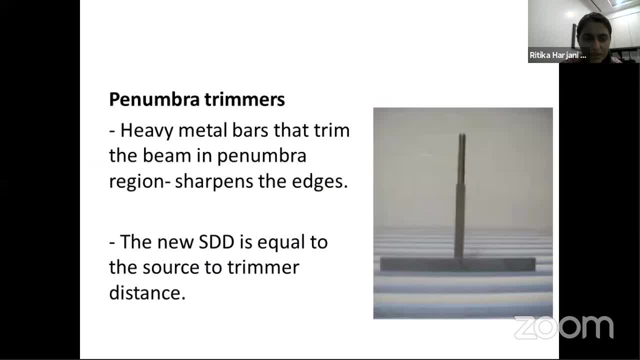 so an application would be will come to it. we have penumbra trimmers. these are metal jaws or bars which are attached to the collimators. this is from our cobalt unit during my PG. we could attach this to the collimators and bring the source to. 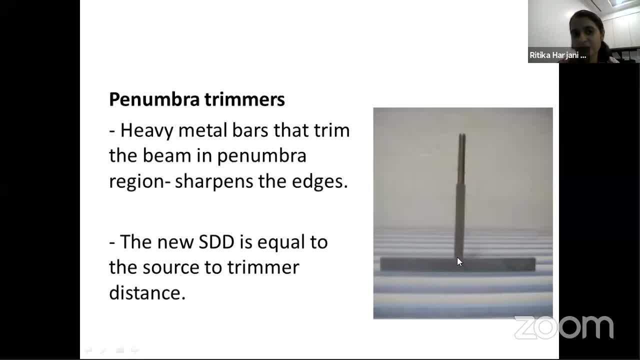 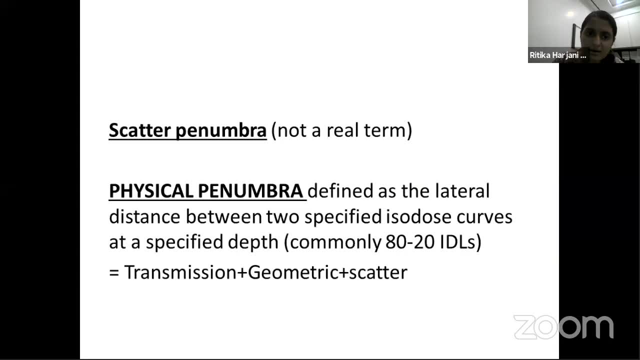 the diaphragm distance can be increased and thus the penumbra can be decreased. so the new SDD would be the source to the trimmer distance. again, there is something like physical penumbra which is defined as the distance as I mentioned: 80 to 20. 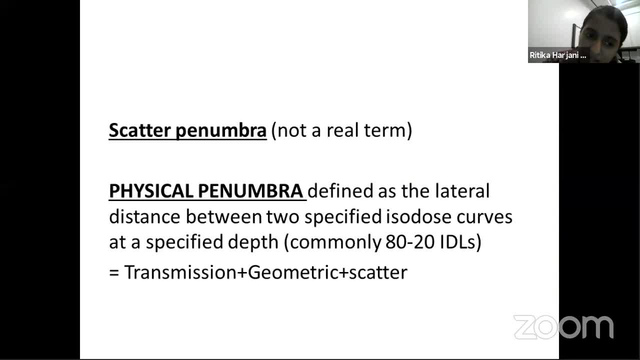 isodose line and it is basically a combination of the transmission penumbra and geometric penumbra and when the beam actually interacts with the patient initial depth, there is also some amount of scattering, so it accommodates the scatter component also, so physical penumbra would be. 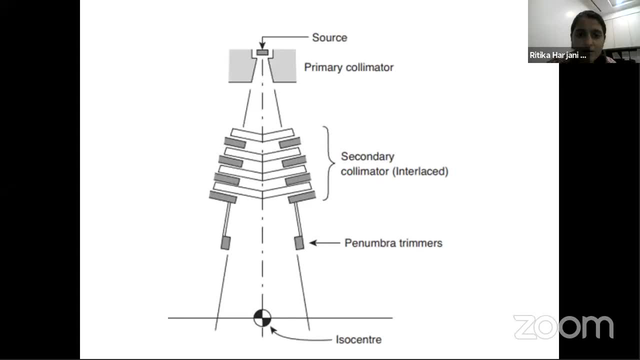 a sum of all these three, and so this is again one more diagram wherein a penumbra timmer is attached. so the source to diaphragm distance has been increased, so the penumbra would be less, and alternatively, sometimes secondary blocks are placed close to the patient. 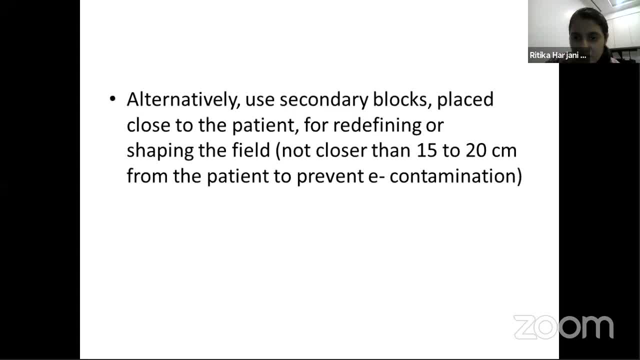 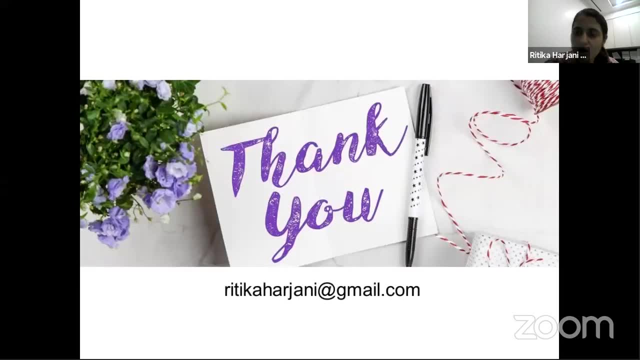 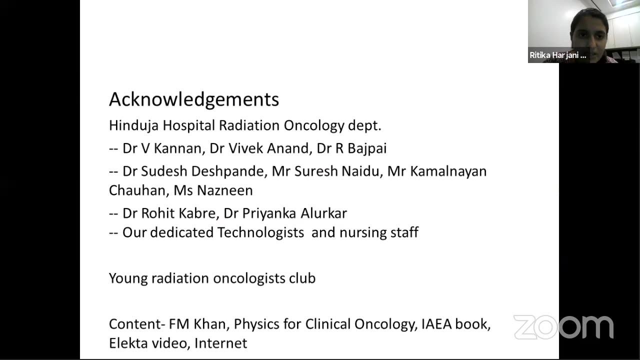 but not very close, also because we do not want electron contamination in a gamma ray beam or a photon beam. I think this is all about X-ray therapy machines in use, the cobalt and the linac, and I would like to acknowledge Hinduja hospital radiation oncology. 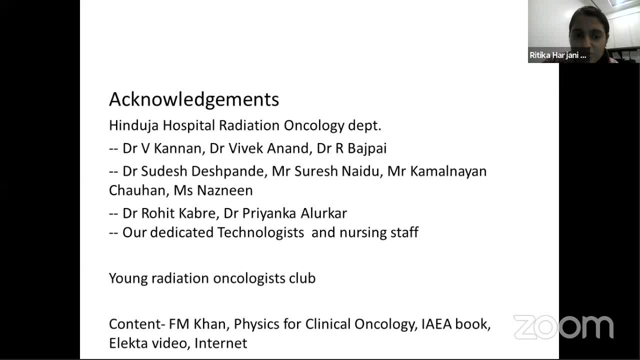 department, Dr Karan, Dr Anand, Dr Bajpayee, the physicists without whom I do not think today this presentation would have. all these have details. so Dr Sudesh Deshpande, Mr Nayadu, Mr Kamal Nayan and Nazneen. 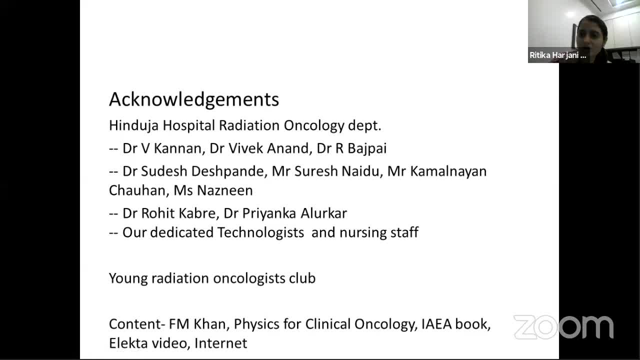 my colleagues Rohit and Priyanka, and our dedicated team of technologists and nursing staff, of course, the young radiation oncologist club, and the content I have taken is from some books and internet, thank you. thank you, Dr Rithika, it was an excellent. 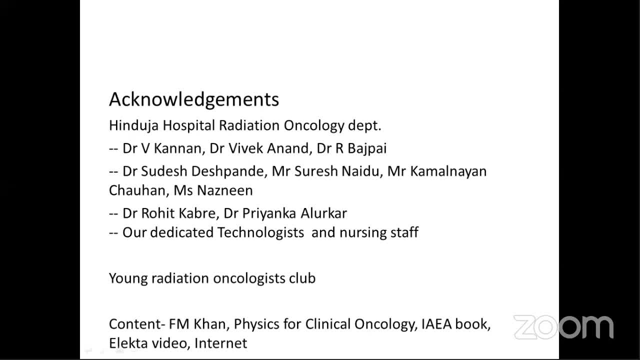 class and it is very nice to see you all, my ex-colleagues. name you have written in the acknowledgement and probably you are in the hospital in the same department I worked eight, nine years back. so thank you for the presentation. before we go to the question answer session, I have 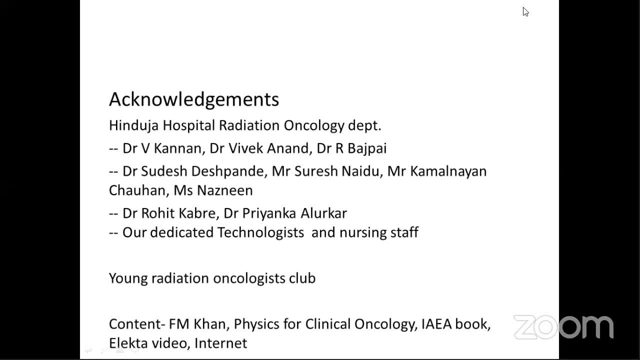 one announcement: that repeat study participants, who have been all, have been registered in the national cancer grid e-learning platform, so you may have got your login id and password. if you have not received it, please email us. we will send it again. so now, Dr Jeebo, can you? 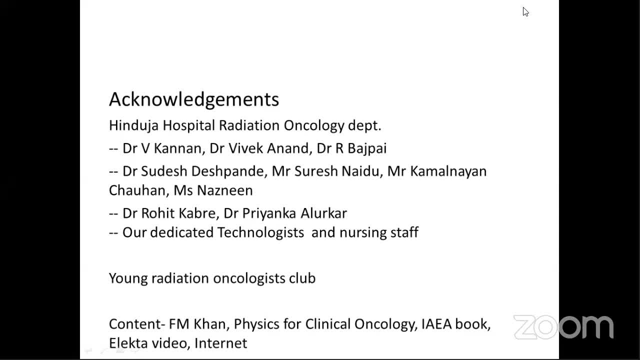 go to the question answer session? yes, so the first question is: what is the difference between KeV and KV? so basically, KeV is kilo electron volts and KV is kilo volts. the difference of that central e is: generally we, if you have noticed, we apply the. 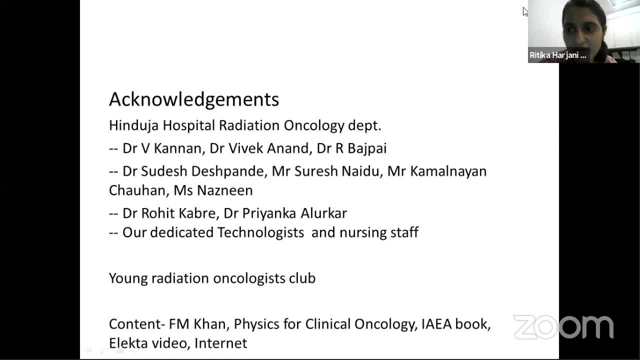 KeV to the electron beam. energy and our photons are more of KV because the x-rays have a range of energy, so that KV is the maximum energy that it has. like I said, 6mV is maximum of 6mV but an average of maybe. 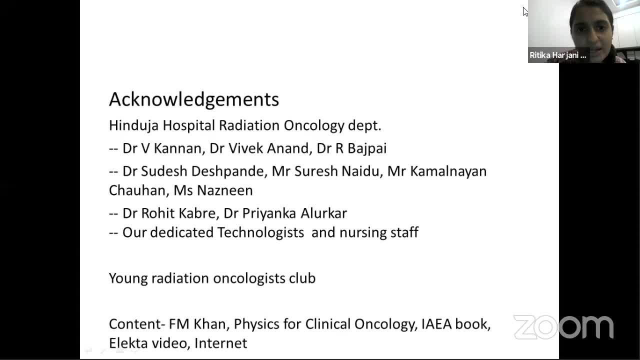 2, whereas electron is a mono energetic beam, so it has a kilo electron volts. in the sense, 6 MeV is only 6 MeV, there is no filters to it. that some of it is less and some of it is more, okay, thank you. 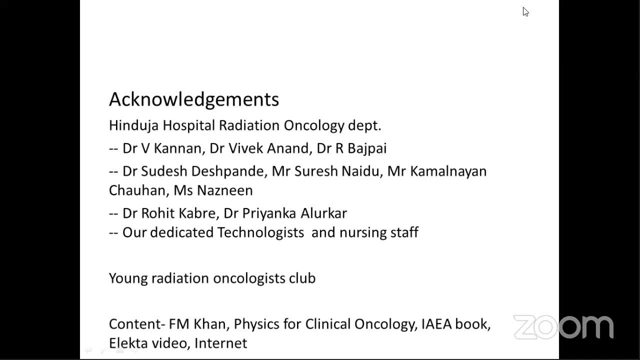 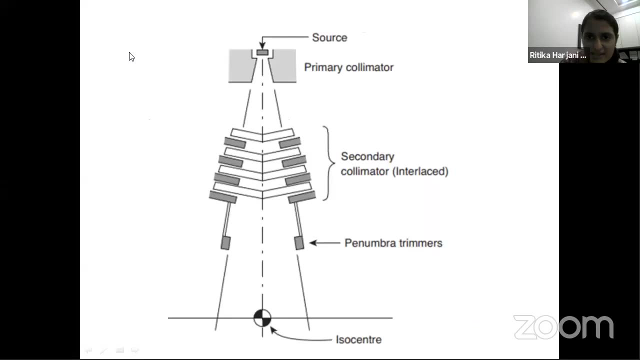 the next question is: what is the SSD? so I think you have explained it already, but they wanted to know again. so SSD is basically, if I just go to the slides, so SSD is if I would say this is the source and if this is suppose the patient surface, not 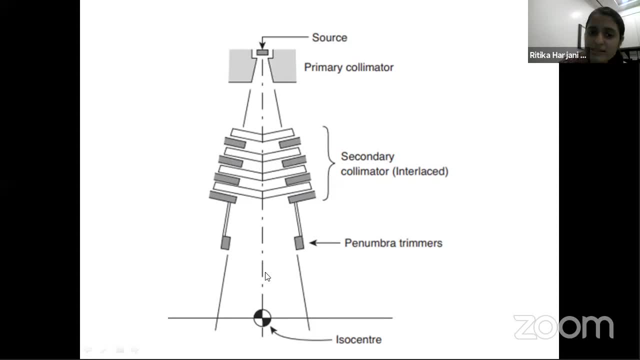 really the patient surface here. but if this is the source to the skin distance is SSD. okay, then what is penumbra actually? this question came before you discussed about penumbra, so I don't think it needs again discussion. next question by Rakesh is how microwaves 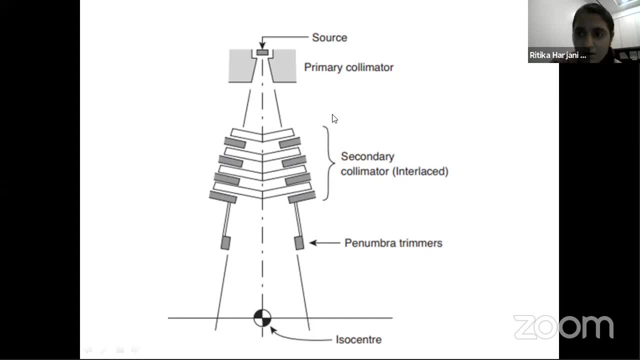 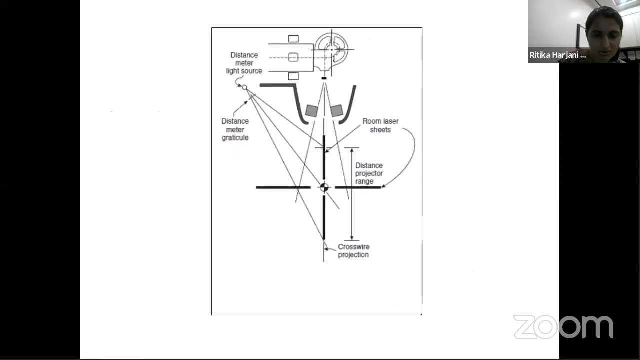 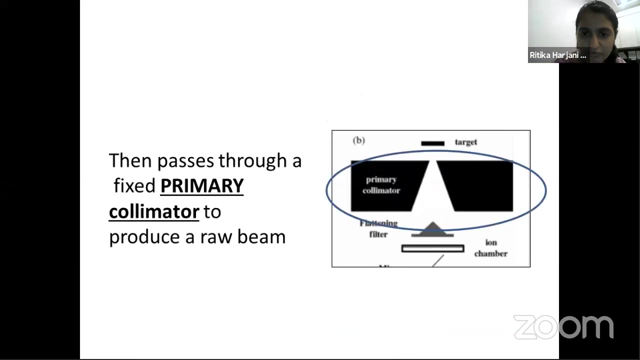 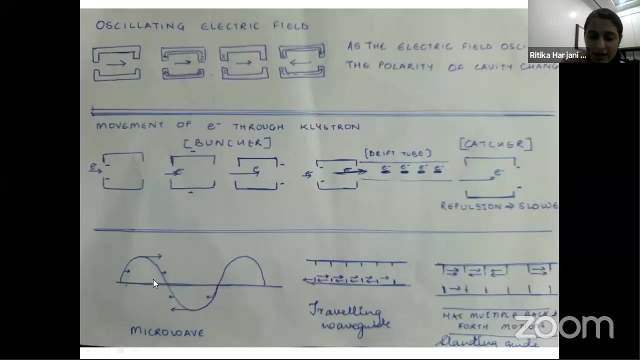 accelerate electrons. I had a. so microwaves accelerating electrons. just in simple terms, is that video that the microwaves and electrons go on to the wave guide and are accelerated, but to talk in detail, so when these, again, these microwaves are a wave form, and when? 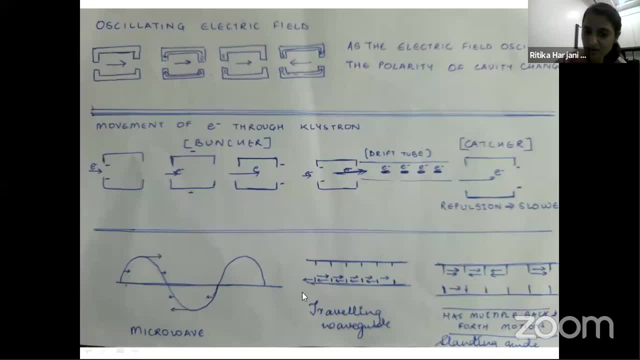 when these microwaves are in the wave, in the travelling waveguide or stationary waveguide, they also. these are basically small, small cavities in a waveguide and they are producing oscillating electric fields, going in one direction the one moment and other direction the other moment. so 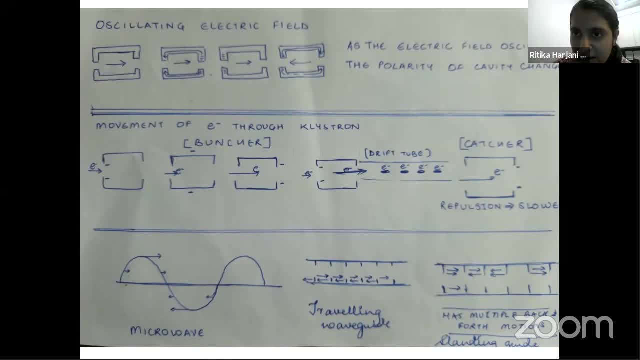 basically electrons and microwaves are already in the waveguide. electrons are injected at such a point that their frequency resonate and it is like they say that like a surf rider. these electrons are injected when microwaves are at its peak and they then travel with. 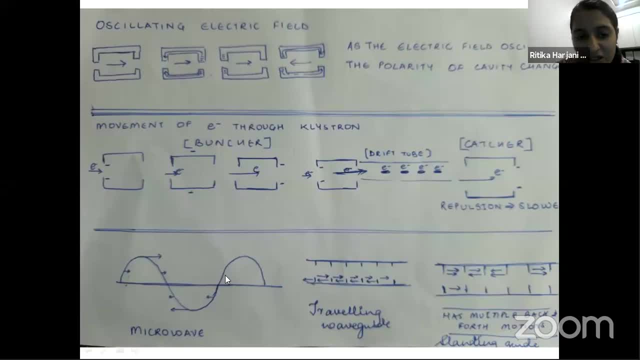 the microwaves gaining its energy. these are very high energy microwaves that are inserted into the accelerating waveguide, as we saw in the that we had produced earlier and we have generated microwaves. does that answer the question? i think so. next question is: 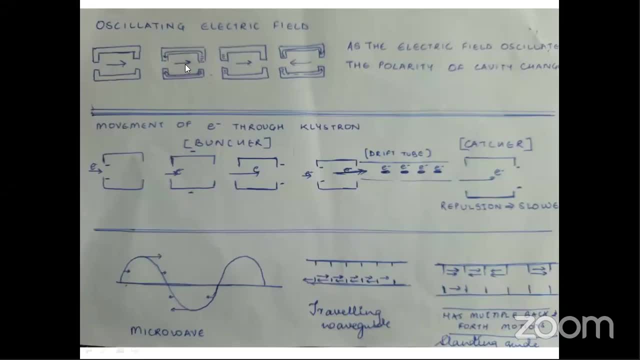 if only amplifies and does not produce microwaves. what produces microwaves in machine? there is a separate modulator, provides the microwaves and there is a microwave force attached to it. so somebody wanted to explain once again the standing and traveling waveguide. 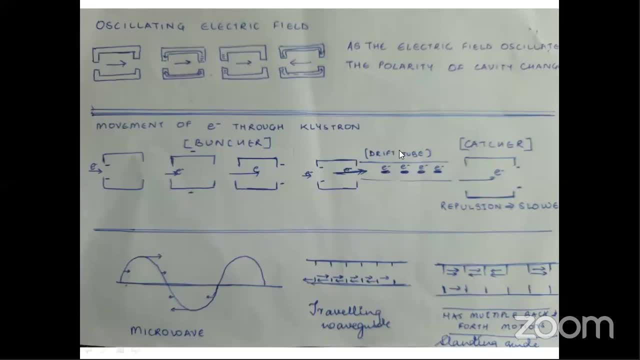 okay, i think this was the last question, only still, do you want me to go through it? i think you have just explained. yeah, i think so. yes, so why is the beam forward picked? kindly explain. so, beam. as in the initial point itself, we noticed that when with the it. 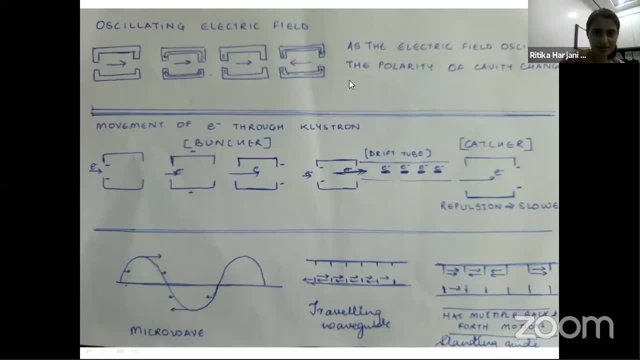 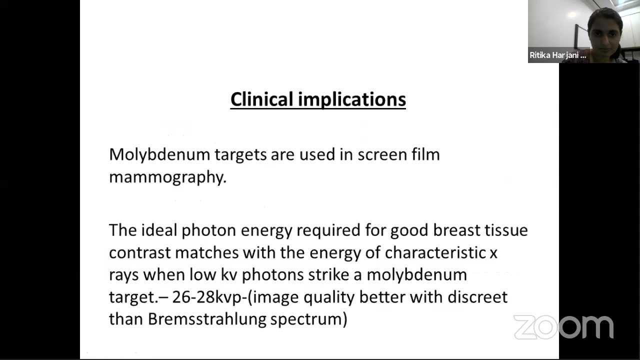 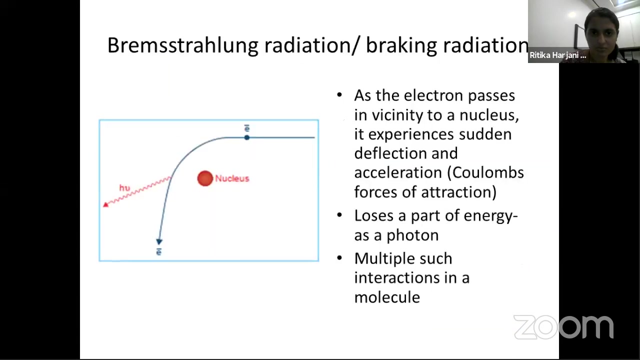 depends on the energy. the energy- again i go back in the power point. so as the as the bremsstrahlung x-rays are produced by interaction of an electron with a nucleus. as the energy of the coming electron is more, it provides more and more energy. 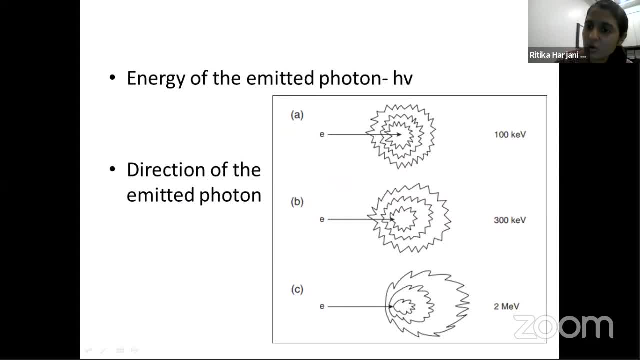 to the photon which is emitted and that is why in a low energy electron it gives, it is not able to give so much of energy to the photon to retain its direction. versus in a high mega volt, the energy provided to the photon is high enough and it retains its direction. it becomes 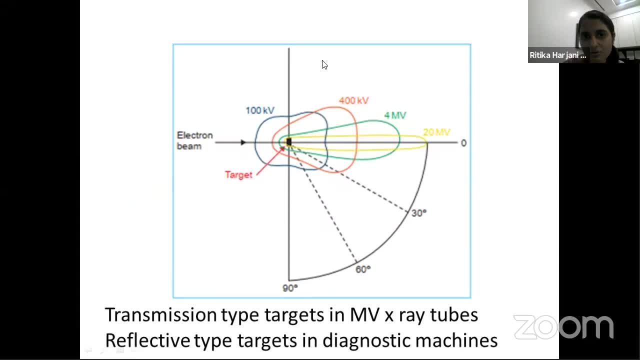 forward peak because of the energy provided. so can you just explain movements of couch, uh, couch movements, basically, um, we have a regular x, y and z direction, which are called as translational movements and like, if you can imagine an aeroplane, so along the longitudinal axis of the 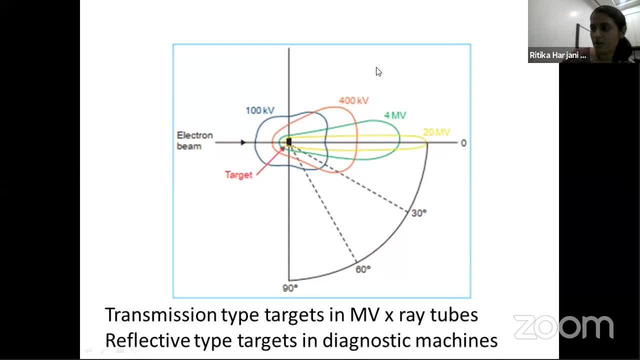 aeroplane, if the aeroplane is trying, or if you try to imagine a pen, if i don't know if you can see me, but this movement along the, along the longitudinal axis, is called the roll, and the pitch through the, the perpendicular to it direction. 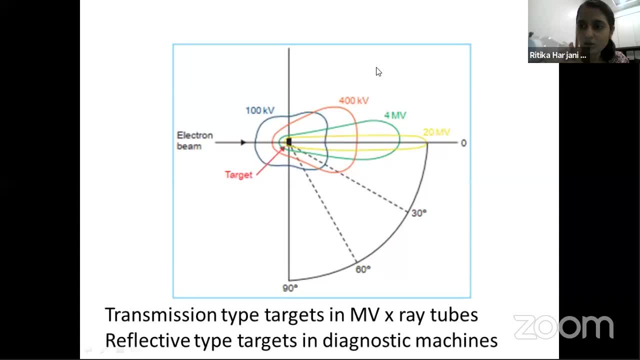 or the perpendicular to the longitudinal, would this movement would be the pitch- i don't know if my video is visible- and the and the yaw is the third direction, which would be um this: so this is roll, this is uh pitch and this is uh yaw, this one. 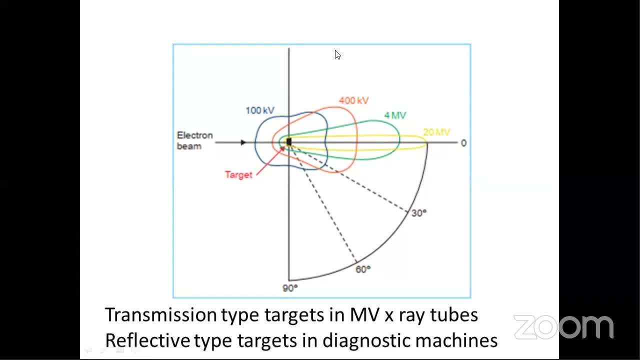 okay, so uh. next question is: uh in linear, when photon beam is used and when electron mode is used? it's kind of clinical question. so just if you can answer in what is the question? question is: uh in the neck when photon beam is used and when electron mode is? 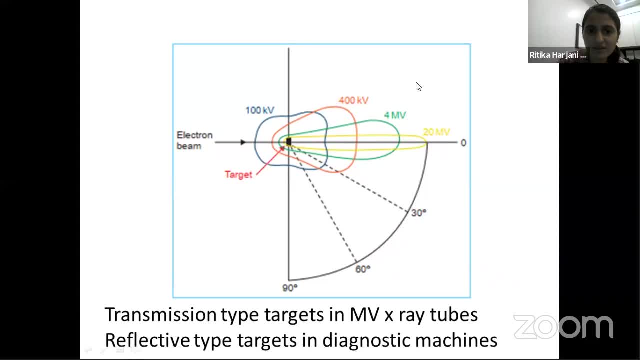 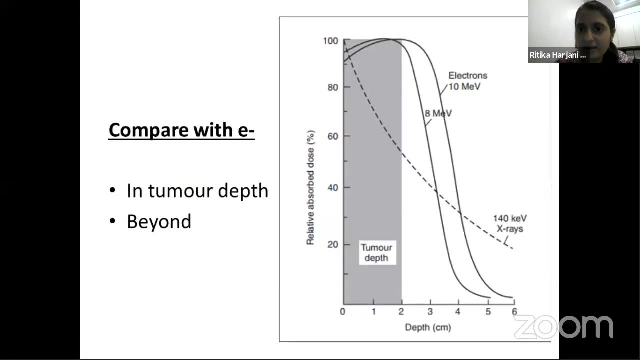 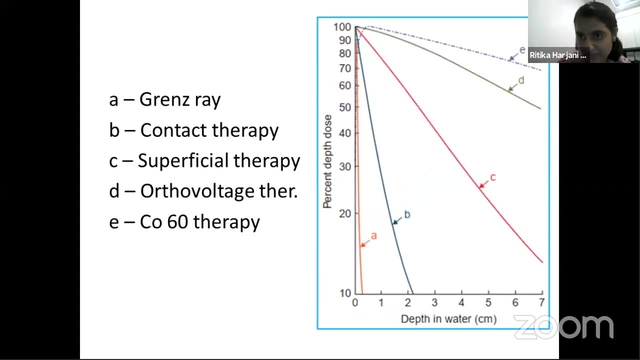 used. so electron, if you have seen the dose distribution, uh, they have a very good dose distribution in the initial part and initial depth and then it falls off. so electrons are generally used for superficial targets and a photon beam like- if you see the e section here, the cobalt beam. 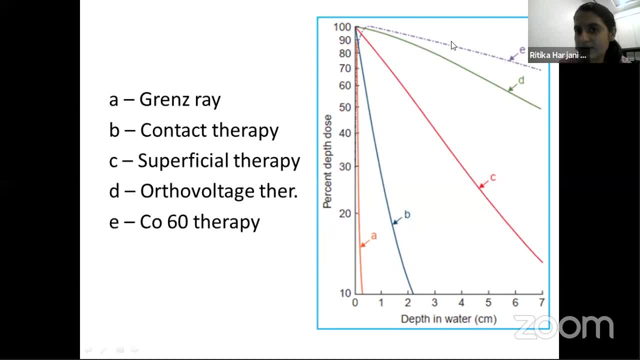 uh, it has a. it is used for deeper areas because it can produce a good depth at a deeper depth, and so, uh uh, depth also, depth also, okay, uh. the next question is from selena uh, who asked: what is the difference between radiation isocenter and? 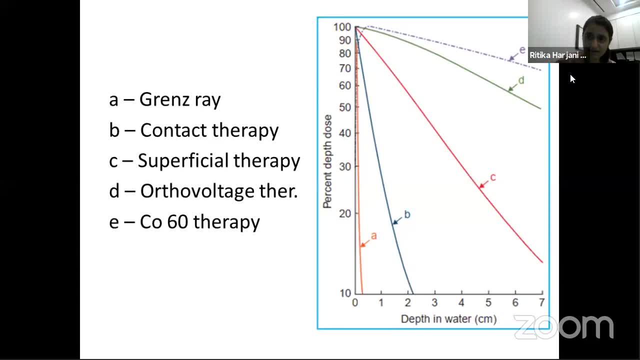 mechanical isocenter? uh, so basically i think radiation. uh, what i understand by your question is mechanical isocenter is the one that is the machine and the radiation isocenter would be for every treatment. we set up an isocenter, radiation isocenter. someone can correct? 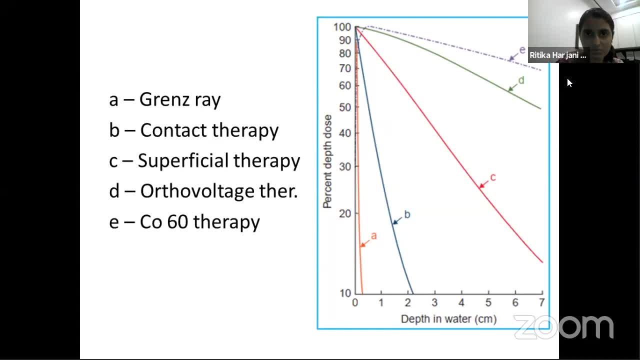 me, if required from the panelists, i think so. uh. next question is: uh, what is the disadvantage of penumbra? uh, so we want the entire intensity of the beam throughout the field size and penumbra. we are seeing that there is lot of uh. dose fall off from 90 degrees or 80. 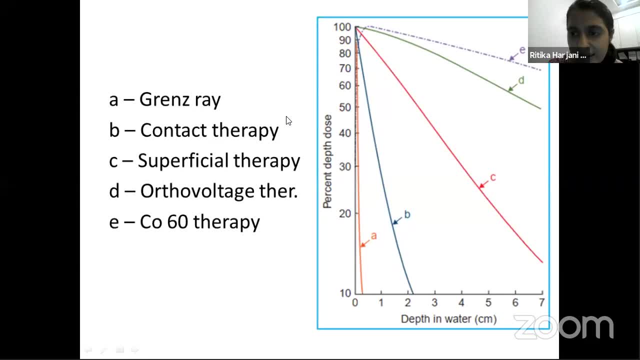 degrees to 20 degrees. it is very steeply falling in that edge. so we do not want those low doses to actually be received by the target. so we want a more homogeneous beam throughout the field and that is why we do not want the penumbra. 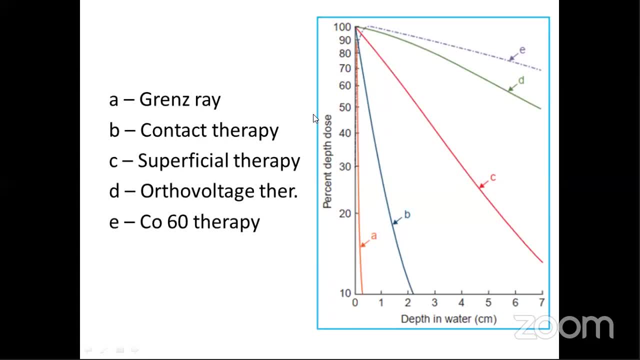 okay. the next question is: what is beam hardening? i think this will be discussed in quality of x-ray beam, so you can omit this. then please explain vandy, graph, beta, tron and microtron. if required. i can, but i think we have short of time because 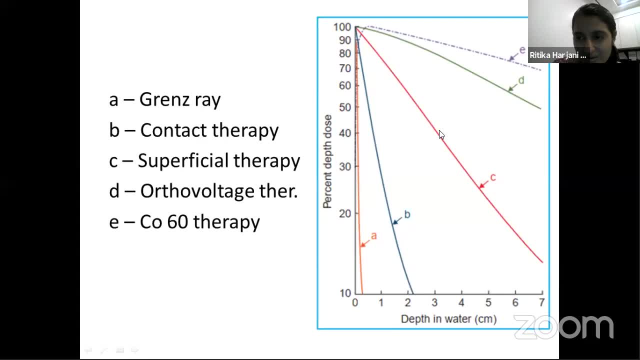 it's already 9: 23.. the presentation- i don't know if it will stream on youtube later- has slides on betatron and microtron and vandy graph also. okay, that's great. uh, can we get the video? it is, it will be available for. 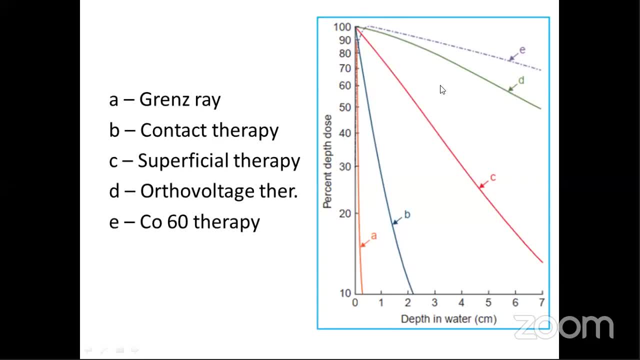 download in the ncg portal and you can see it in youtube also. um, ma'am, could you explain the relation of target size with linac energy again? so they want to know the 6 mb and 15 mb with inverse target size relation. yeah, so basically. 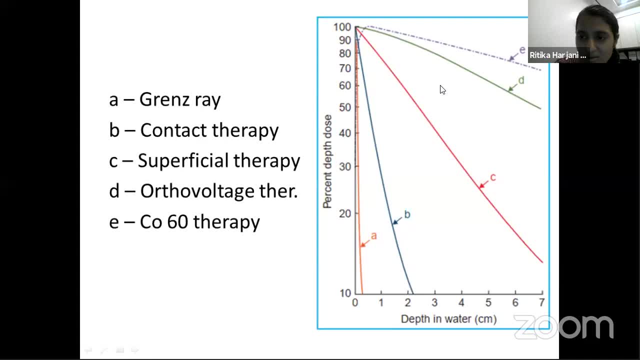 the efficiency of the beam depends on the voltage of the beam also, so 6 mb will have a lower efficiency of production than 18 mb. 18 mb will produce more photons and lesser heat than a 6 mb, and 6 mb will produce, uh, uh, more heat and lesser uh. 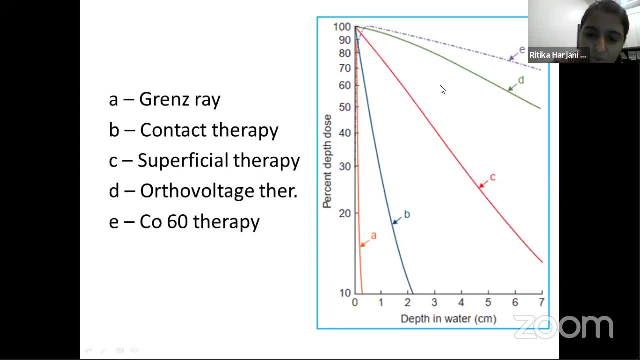 photons. so that is why uh 18 mb will have a smaller target, because it produces more uh photons and that and doesn't require a wider surface for the heat dissipation also. okay, uh. next question is: uh, what all components does, and linear accelerator need to have both electron and photons. 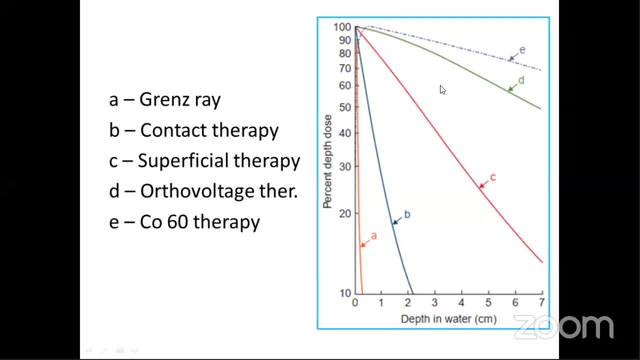 as if is it just scattering file availability or something more? you don't understand the question: what all components doesn't need. i can't hear you properly. can you be little now? yeah, sorry. the question is what all components does. an la need to have both electron and 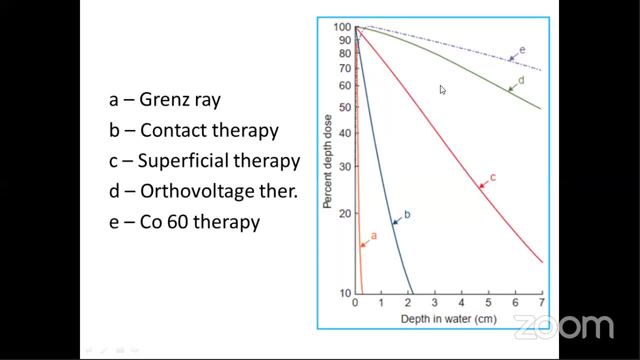 photons. is it just scattering foil availability or something else? i mean, for any linear accelerator you will need electron and photon, i mean, and you will need all of those components. it is just that those two components are different. you need everything: the ion chamber, the collimators, everything. 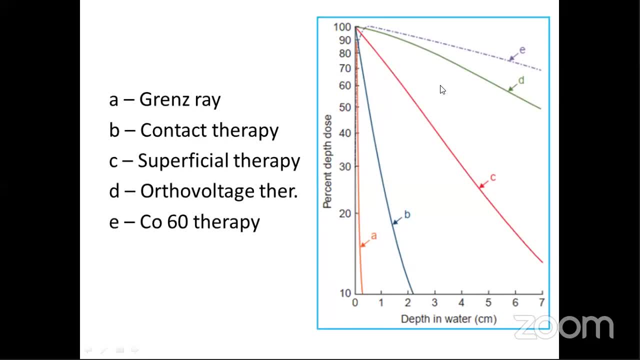 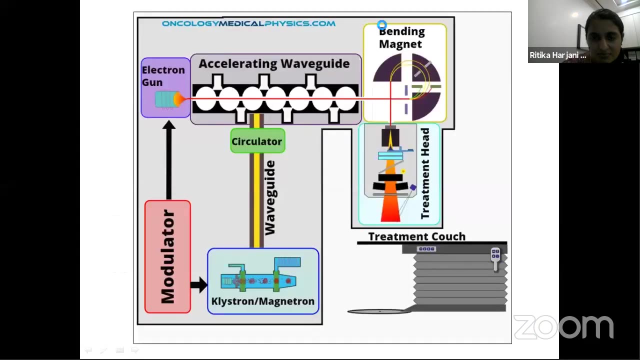 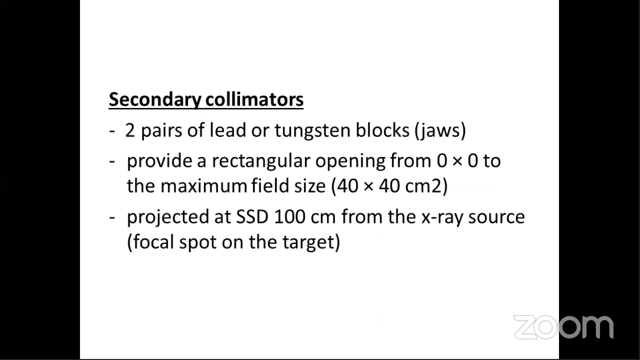 then, uh, how? in geometric penumbra diagram the vertical distance ratio was equivalent, though it was not a part of the equivalent triangles. um, can you go to the penumbra? and the next question is again geometric penumbra explanation. so i think you will do. 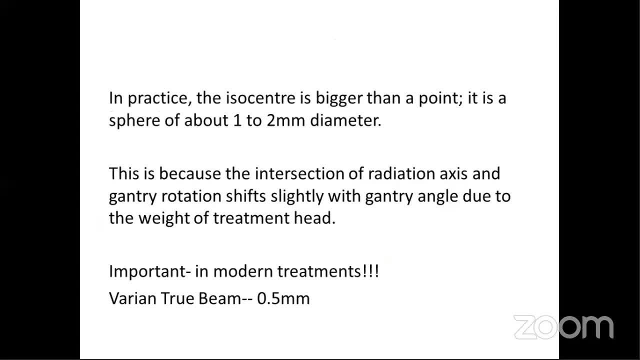 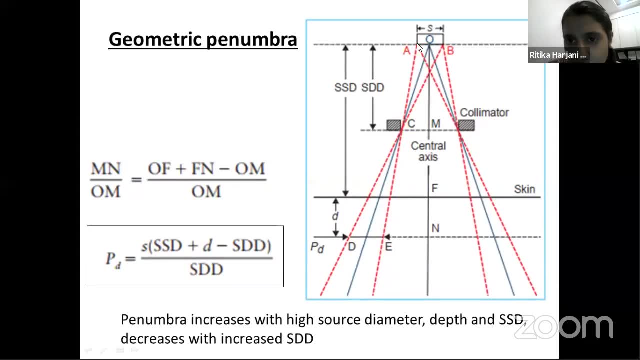 it so. so, uh, i know that c a, b and c d e, and suddenly we are coming to the central axis. but then just that, if you take these sides to be equal, then hypotenuse, or also the ratio of the hypotenuse, also becomes the same. 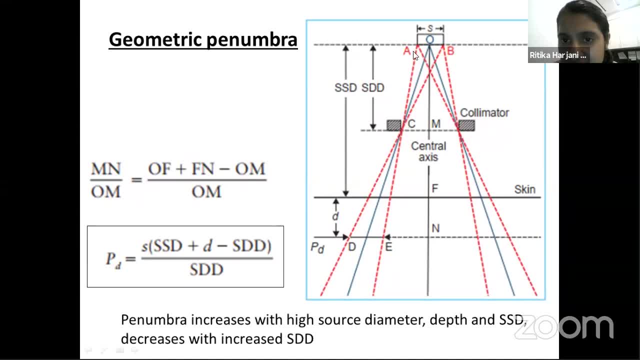 so, uh, in equivalent triangle, if c a upon c, e is equal to c b upon c, d, it is also equal to c o upon c. this point here, which is not t there, and then this triangles are equivalent if you form a triangle here. so basically, this projection from the 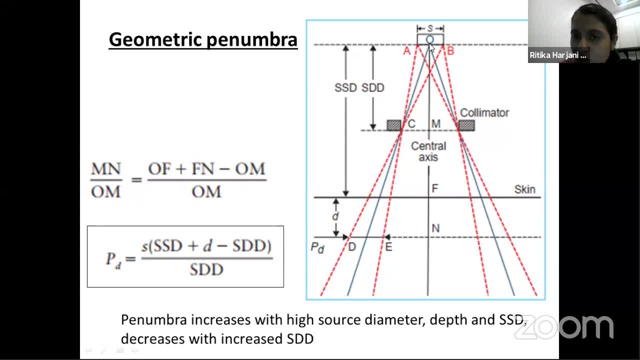 center of the angle to the center of the opposite was also the ration. they are not equal, of course, but the ratio remains constant. and then this is quantified to this triangle, and that is how the om and the q angle have full infants and and will stay the same. so now, this has been, this has been quantification here, and that is how. 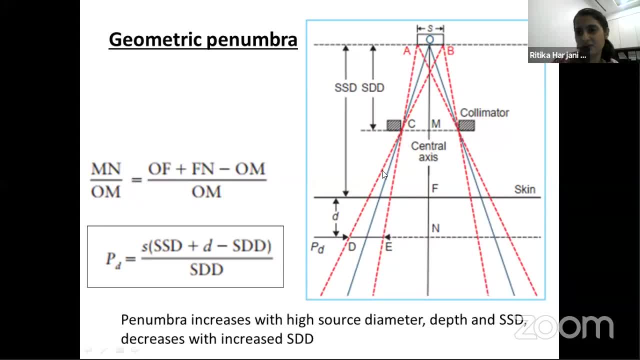 the om and the mn is included in this calculation. and to calculate this, this, uh, in this we are basically now taking sides of this: ab upon de is also equal to um, om upon mn, or here they have written in the opposite. so mn upon om is also equal to de upon ab. and then, uh, this, this, oh.